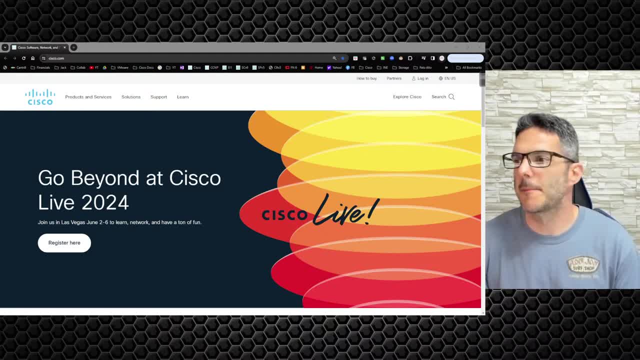 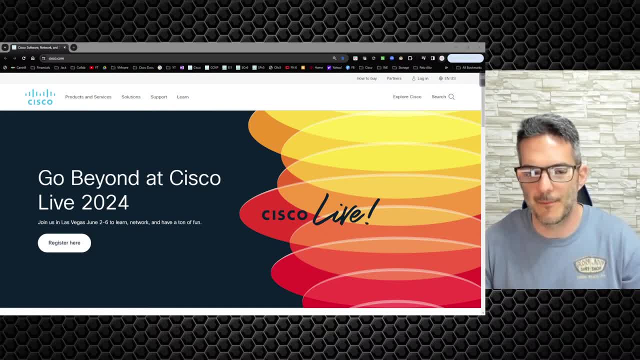 not going to work. Okay, Why does it do that? I don't know. People share invite. copy meeting link. Let's try it this way. There we go, All right, so if anybody's interested in joining the team session. 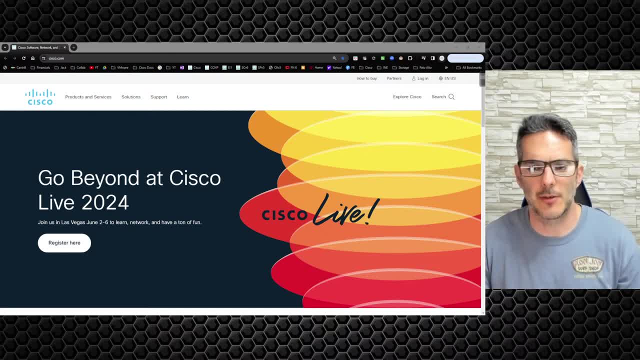 feel free to join on that. I normally run it on the coaching sessions on Friday, but I figured it couldn't hurt to do it here, in case anybody's got a specific thing that they wanna talk about, or what have you. So, like I said, we are going to talk about. 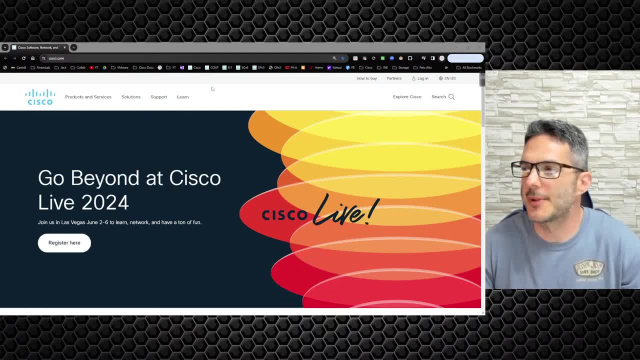 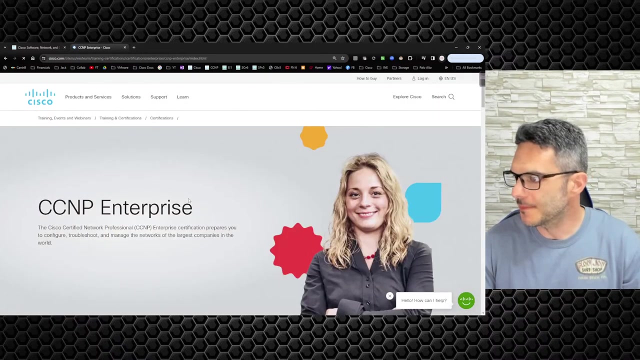 addressing structure and things like that. So I'm actually gonna pull up the CCMP blueprint and we'll go from there And with the intention of talking about the preparation for the exams and things like that. So let's go ahead and jump over here to exams and training. 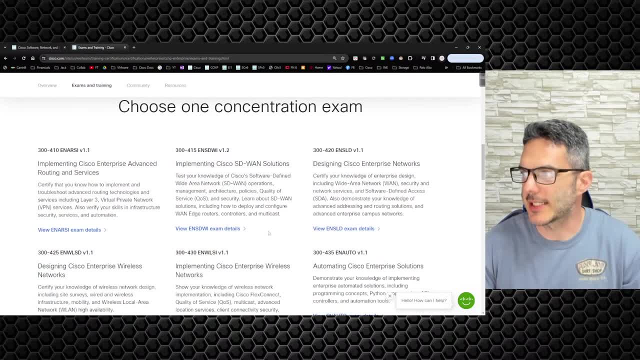 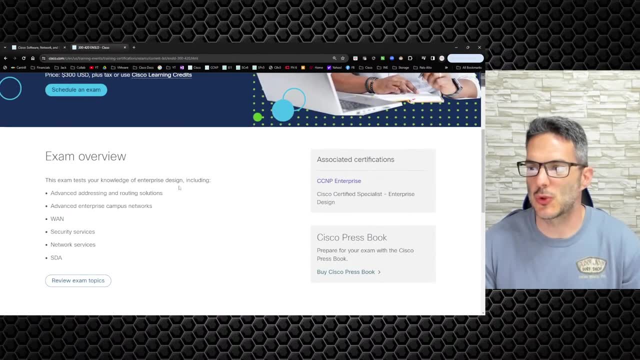 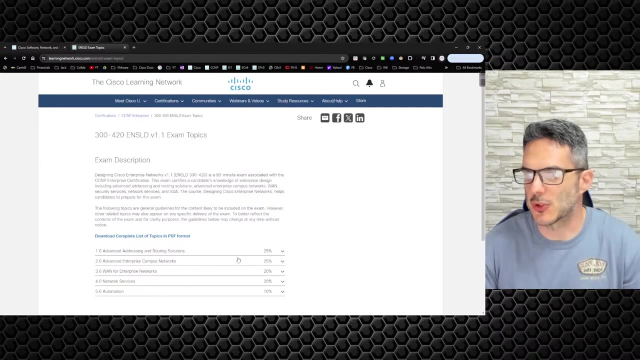 So we're gonna look at the design exam, because there is a big section in there that is specific to addressing. So we're gonna take a look at what that would look like and all the good stuff that goes along with that. So let's go ahead and take a look at. 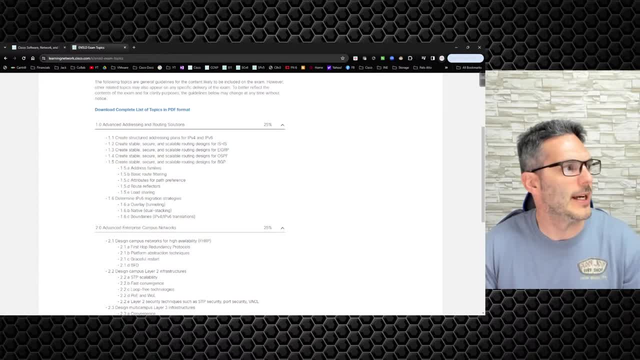 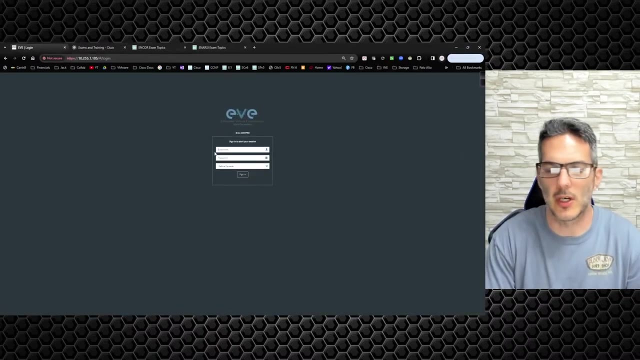 what this might appear to be, And I'm also going to pull up, let me. I have a lot of screens open, So let's see here. So this guy- yeah, I think it's this guy. Let me go ahead and log in here. 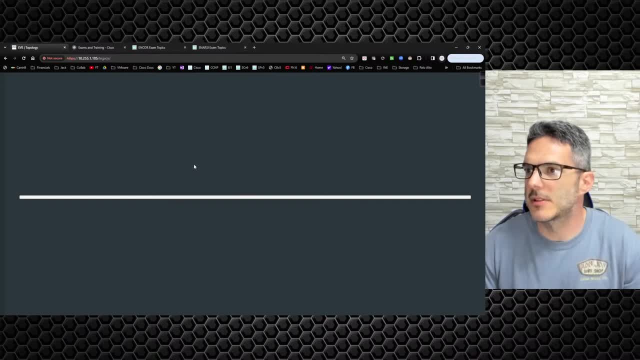 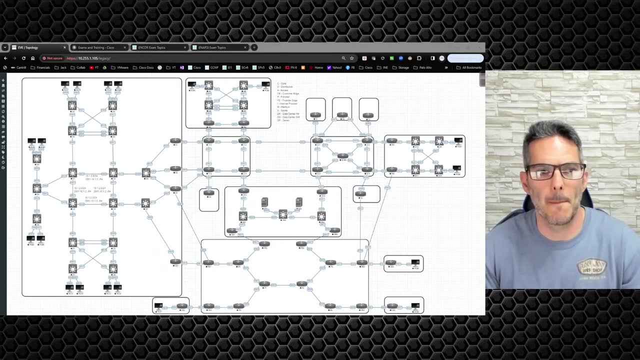 and we're gonna go ahead and this will work. so this is going to be the topology we're going to kind of run with and this is the on CCMP encore in an RC topology that I'm working on that is going to be there for the CCMP studies, if you guys are working on those. so we'll take advantage of this topology. 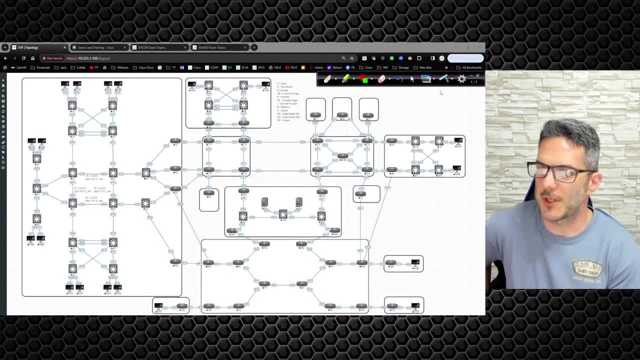 here for our discussions for this evening and stuff like that. so I know there's a few you guys currently in watching the chat or watching the video live. so thanks for stopping by. I'm gonna go ahead and mute my phone real quick. I forgot to do that before I got in here, but we're gonna. 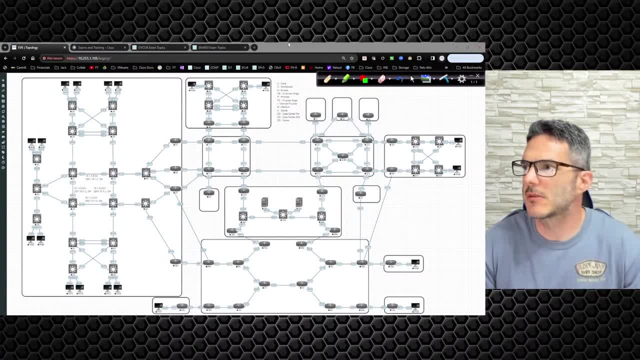 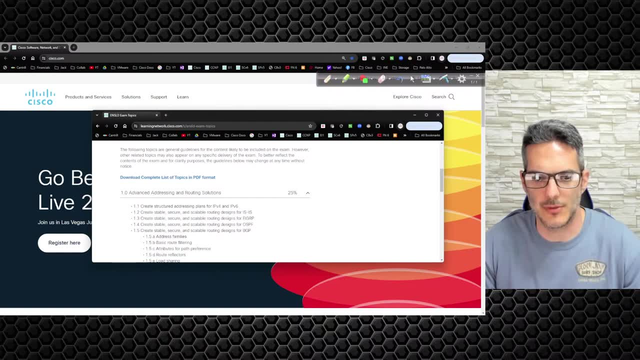 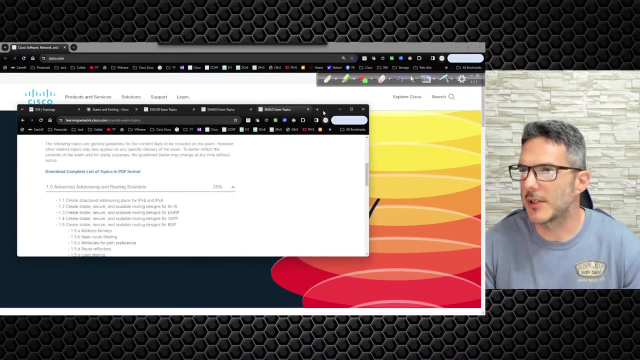 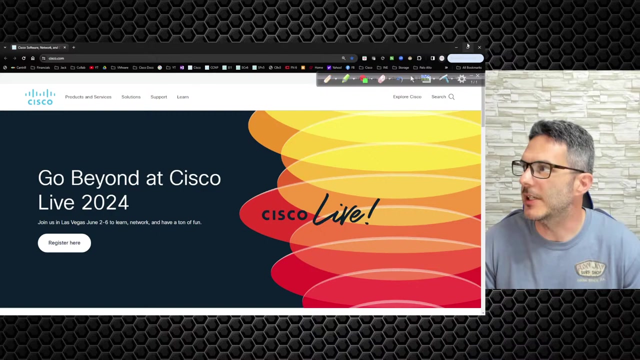 bounce back and forth between the. actually, let me grab whoops, I want to do this- and we'll drag them all together and then I will make that full screen and then we'll grab this guy here and we just get rid of him. we don't need that. all right. so, and if anybody's 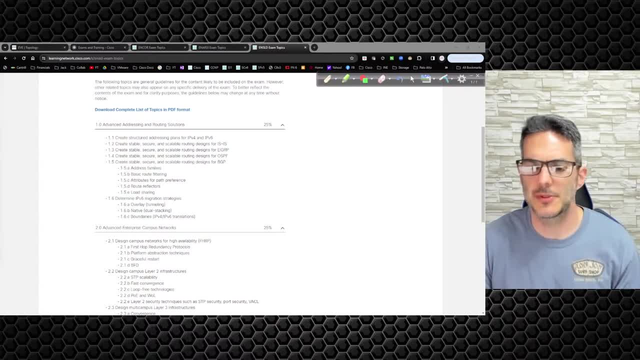 interested in chatting with me, live in Microsoft teams. you can go ahead and click on the link. if you don't see the link in the chat, do me a favor and let me know in the chat where I'll be able to let you in and you'll be able to chat as if we were actually in, like a customer meeting. 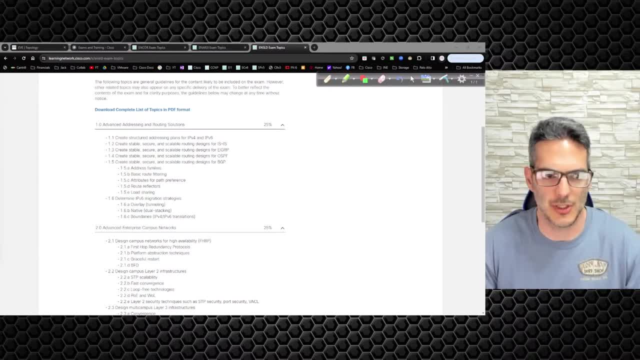 or something like that. or if you've got a specific question, you can word the question and all that good stuff that goes along with it. so if not, that's okay. it's really dependent on whether or not you want to go ahead and get rid of that. so good stuff, alright. so I'm gonna go ahead and we're. 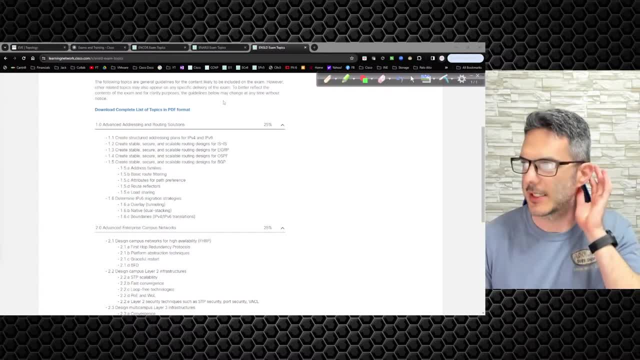 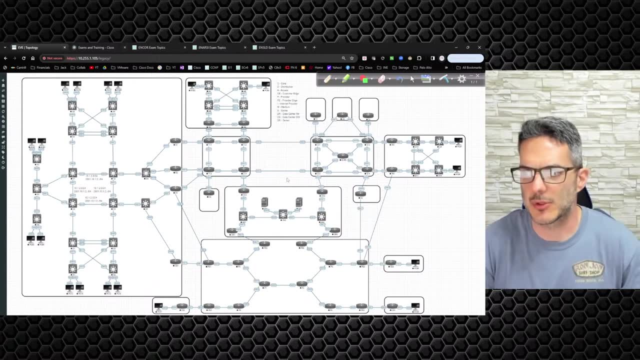 gonna start diving into the interesting structure and the plans, and I think this is important because if you're- especially if you're- like new to large-scale network design and you're looking to get a better grasp of what comes into play with that, it's important to understand the details behind it, because it 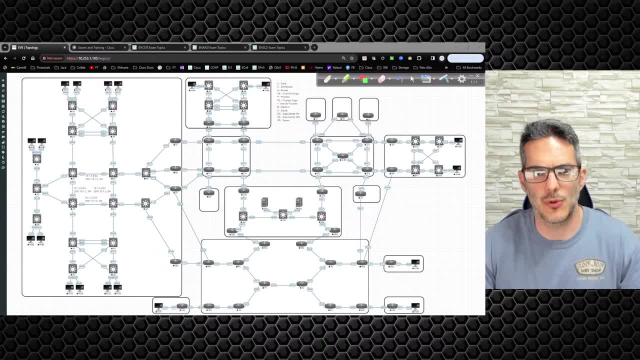 can be very overwhelming if you you have an idea of what you're trying to accomplish, but you may not know what you're trying to accomplish. but you may not know what you're trying to accomplish, know exactly how to get there right. and so the the common thing that I see a lot 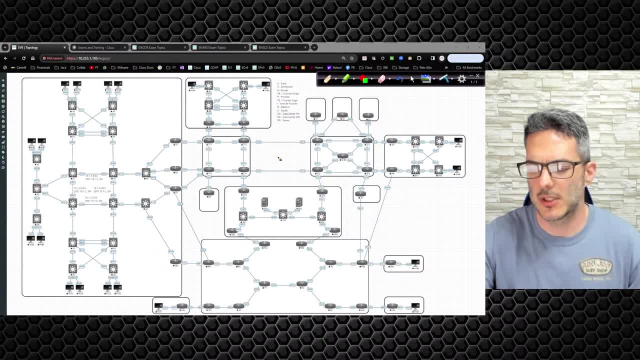 of folks struggle with, especially when they start getting into design work, is it's not. it's not binary, like the technical pieces are right. so, for example, what I mean by that is, if you enable OSPF, for example, let's say, we use all of these devices right here. we're just gonna draw a big circle around all. 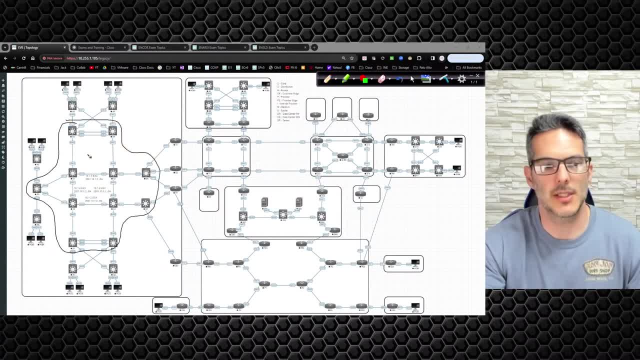 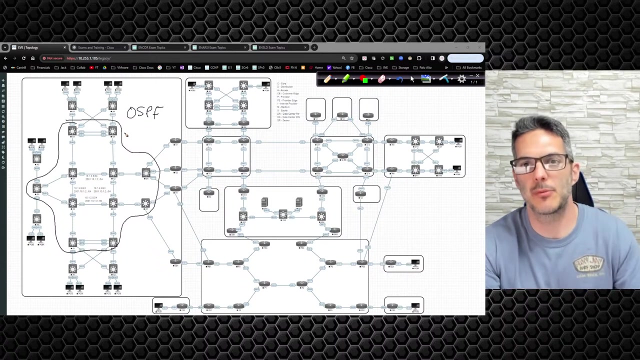 of these guys. for the sake of argument, let's say that all of this is gonna be OSPF enabled, right? excuse me, I just had dinner. I was actually rushing up here right before the live started. so OSPF has enabled and we just turned it on, right? we don't do any optimization. 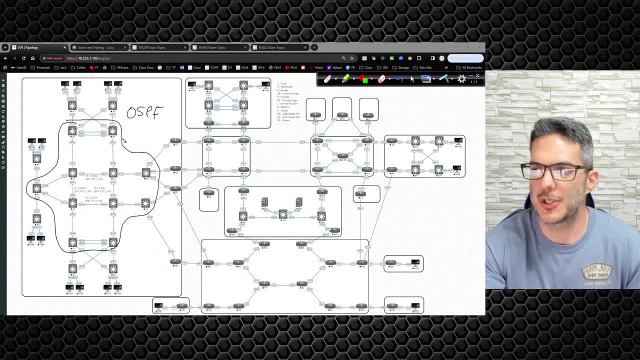 and what would an optimization be? an optimization would be: we go to all the interfaces on the devices and we use the command point to point. so what does that enable? well, that enables us to get rid of the type 2 LSA. right, so, no more designated router backup. designated router election- so, but that's a binary. 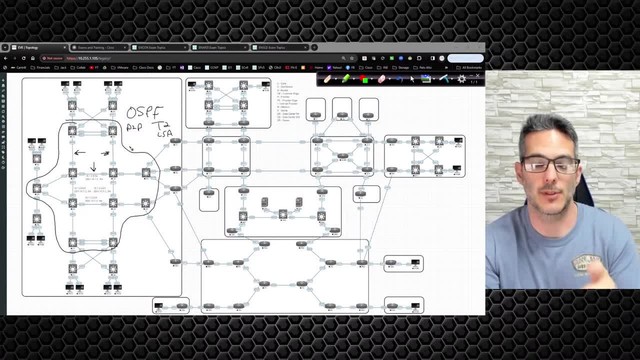 act right. so it's: either you turn it on or you turn it off. it's either on or off. so where's design is kind of subjective, now there are aspects of it to it. where are? they are more direct, where you might get a scenario in the exam that says, hey, we want you to go ahead and try to optimize. 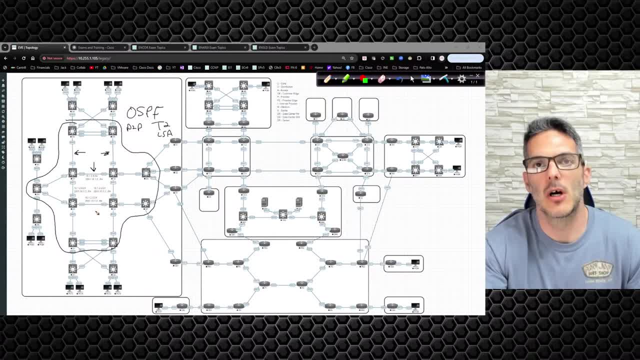 the routing table or, I'm sorry, not the writing table- optimize the OSPF database in such a way that you can. optimize the OSPF database in such a way that you can. you're gonna get rid of any type 2 LSA is. or they might say, go ahead and move. 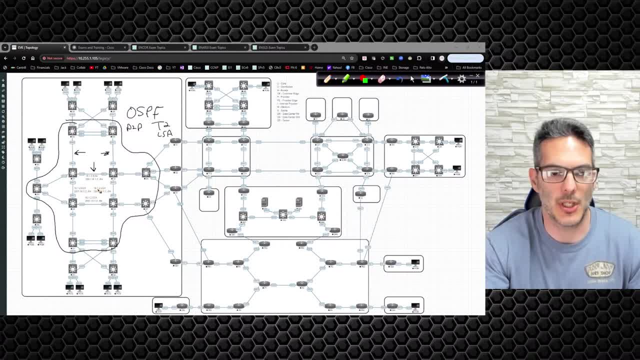 away from doing a drb Dr election process. so that's gonna be based off what they're asking you to do. they're gonna want you to move to point to point network types. now, though, the caveat there is that's not really a subjective network design, that's more of a 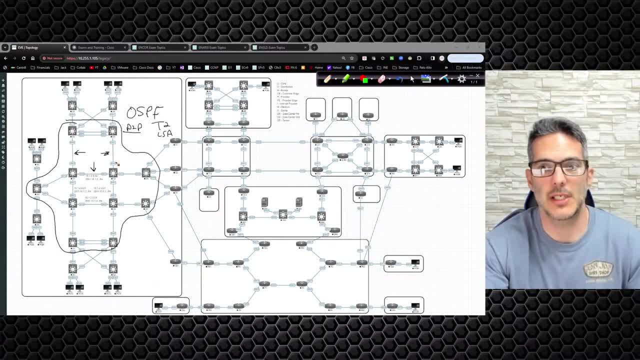 It's very easy to based off the way that they're wording something. it's very easy to make that a reality. right, Because it's binary, It's either on or it's off. So that's that Now. another example of this would be not specific to the point-to-point network type, but enable OSPF in this. 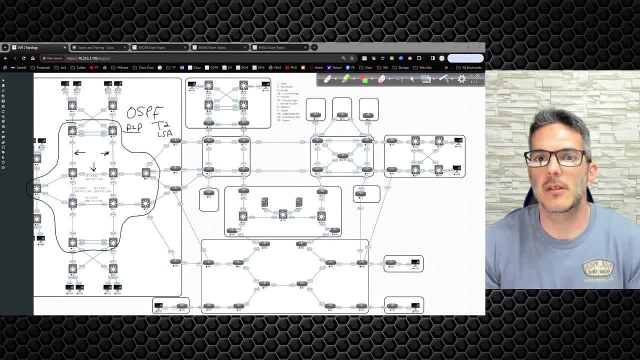 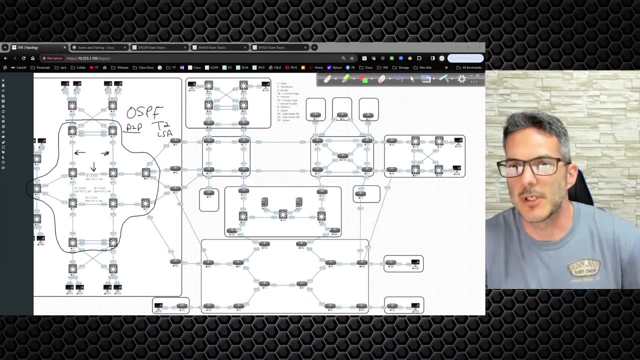 Oop, I have somebody trying to join And who's coming in? Sure, we're going to admit Dave. Hey, David, Can you hear me? Oh, I wonder if my settings are goofed up again. Device settings- my speakers. 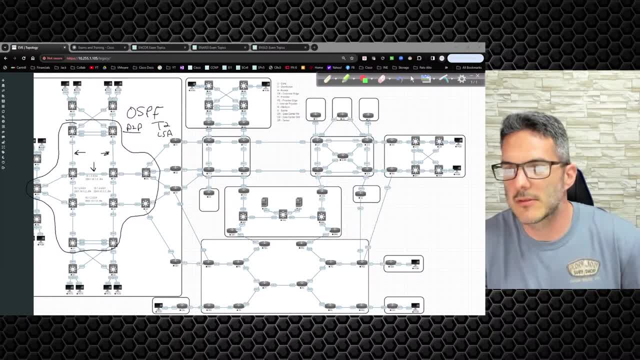 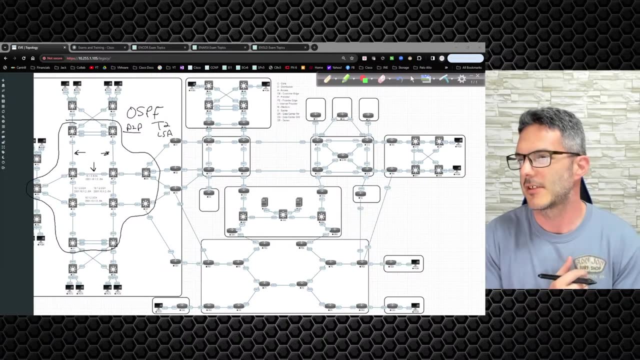 Oh, my microphone's correct. Okay, good deal, All right, Can you hear me? Yes, I can hear you. Okay, you're good man. How's it going? Doing well, That's good, Hopping in to say hi or just hanging out. 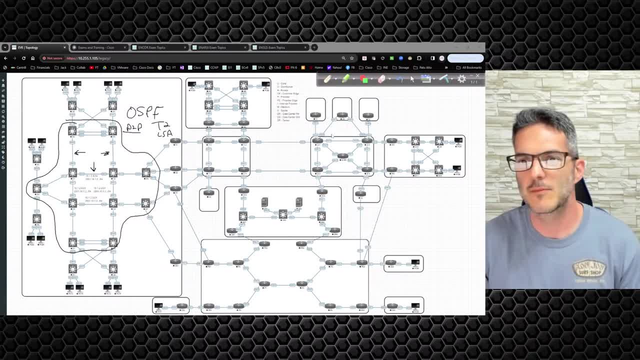 I just heard you talking about joining on Microsoft Teams versus the YouTube, so I was just going to try this one. Oh cool, Yeah, if you do, if you want, if you got something you want to chat about, we can go ahead and do that. 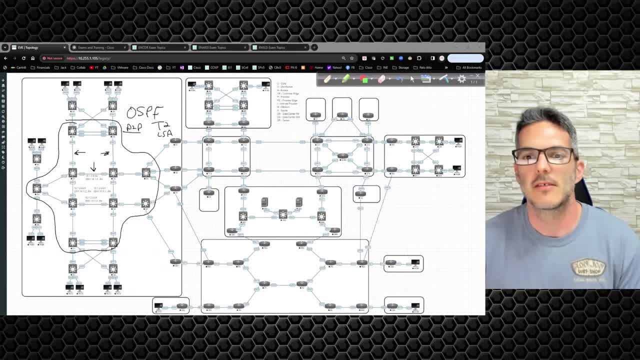 If not, you can just sit back and be on mute and hang out. Either way works, So no worries. So when we take a look at how somebody could make design subjective, so when you look at enable OSPF in this big area of the network, 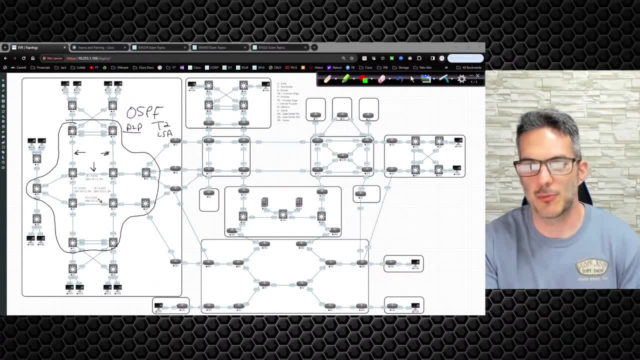 the caveat here is there's multiple ways of getting the job done right, And that's where when I say subjective, is there one way right or wrong? No, they both get the job done, Whether you use the network statement underneath the global routing process. so, router OSPF 1,. 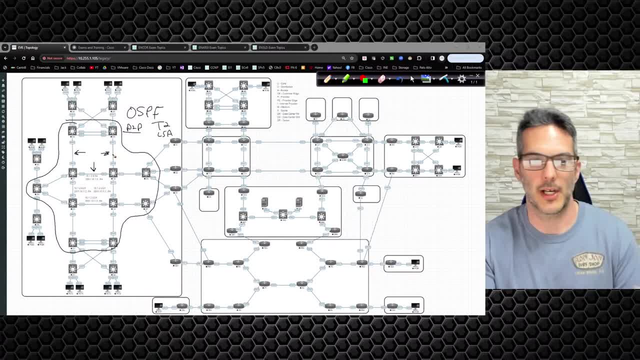 or if you go to the interface level and you type in IP OSPF 1, area 0. They do the exact same thing. So, in terms of that, that's where it gets a little subjective, because you have options And there are multiple ways as you progress through when it comes to the design. 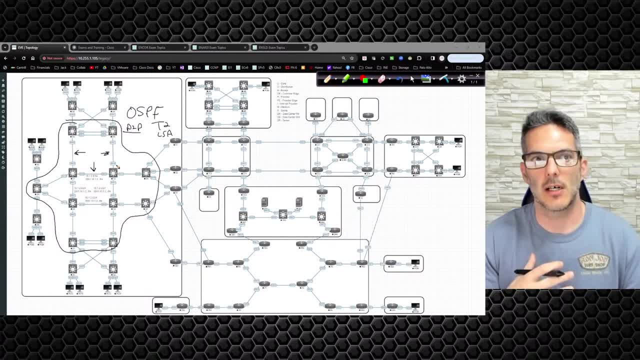 that you have to keep in mind what your options are, And a lot of times, at least in the more senior level roles you get into- is you have to be more cognizant of the end goal, of who the customer is. So the more technical you become, the likelihood is you're going to be much more technical. 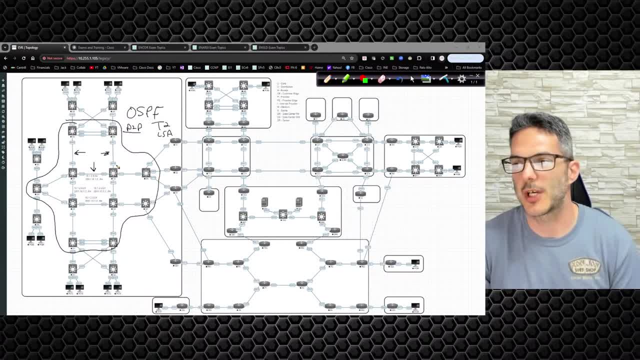 than the people you're talking to. That's just the reality of the situation in most cases- Not every time, but I'd say more than 50% of the time. I'm typically the more technical person in the room And they're normally okay with that. 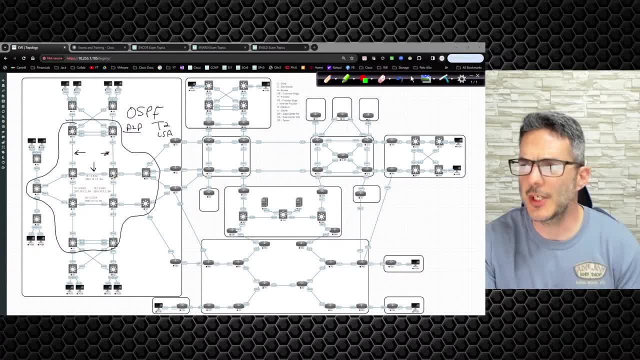 That's why you're there, right? So, when you get into things like this, these are the times where you need to be able to say: okay, there's three or four different ways that we can accomplish something, and they're all going to get us to the same destination. 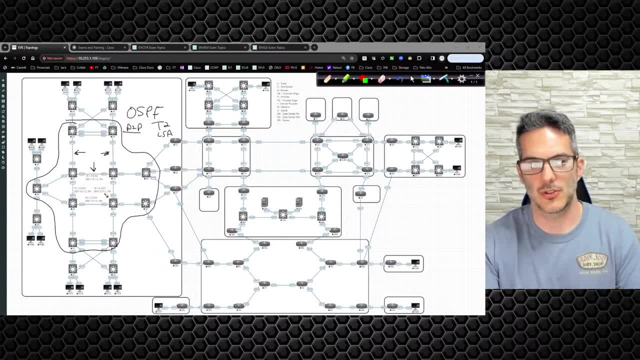 But, at the end of the day, your goal is the consultant or the subject matter expert- is to be able to provide them different options and things like that. So in that particular case- that's where I say subjective, in terms of the options that you have available to you. 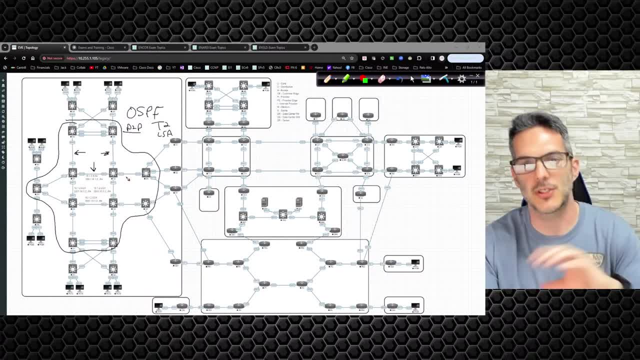 Not saying that you're going to be criticized by going one way or the other. You might be questioned and then it's your job to be able to break down those differences, But overall, most of the time, most customers are pretty lazy Yeah. 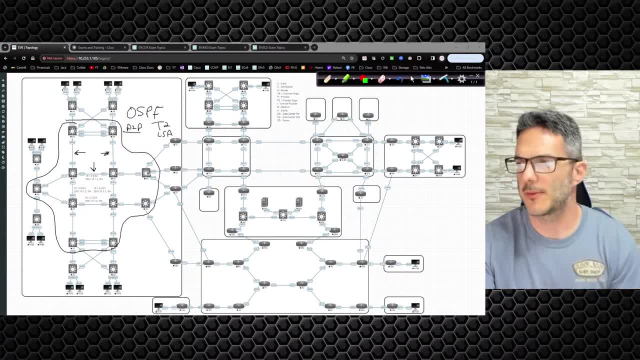 Yeah, Yeah, back and chill about how you want to proceed with something. now, specifically to addressing that, because you have a little bit of flexibility with addressing right. you have your your 10 net space, right, 10 slash 8, you know your 172 dot, 16 through 31 slash 6, I'm sorry, slash 12, and then you have your 192 dot. 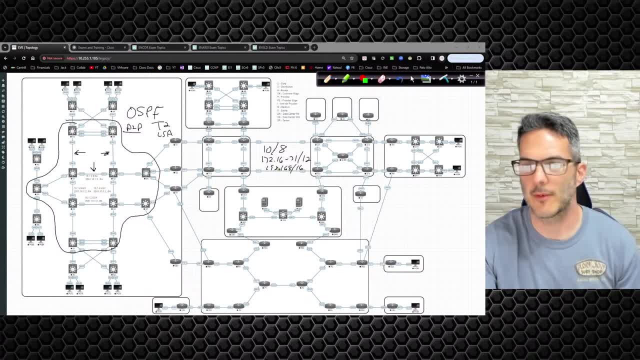 168 dot, slash 16. right, you have RFC 1918. so if you ever heard hear somebody say RFC 1918, that means ipv4, private address space. so when do you use one addressing schema over another? well, again, that's subjective. I personally like the 10 net whenever I'm working on a customer environment, because 10 is a. 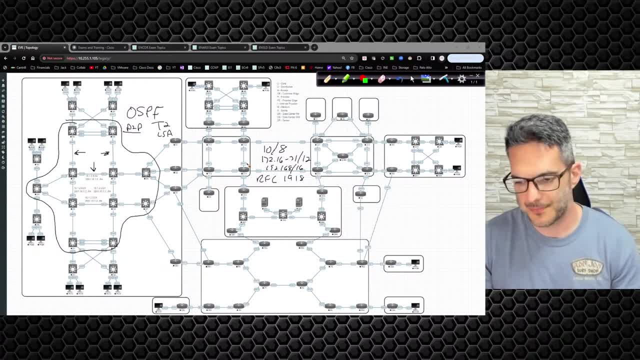 lot easier to type in the 172 or 192. now a lot of customers that I've worked with and a lot of the routing designs that I've worked on. you're typically going to have them broken up into two. you're typically going to have them broken up into two. 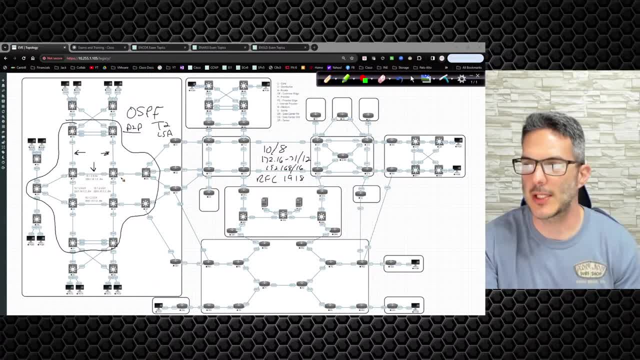 different areas. so a lot of times you'll see transit connections between your networking devices are going to be typically 10, 10 dot something and you're typically gonna see a bunch of slash 30s or slash 31s. so is there again is one way. 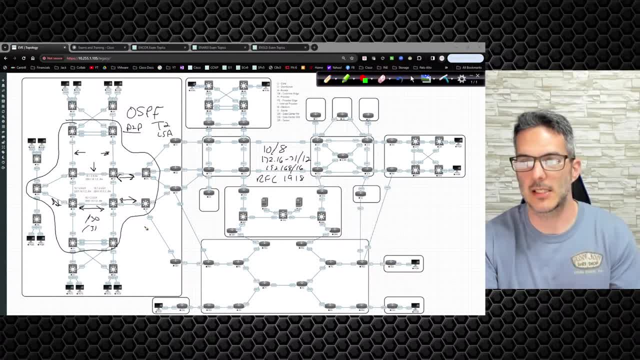 better than the other. no, they all get you to the same end state, and that really, at the end of the day, is the bottom line. so what you'll end up doing is, unless you're working with a customer that's standing up a brand new site, and I can. 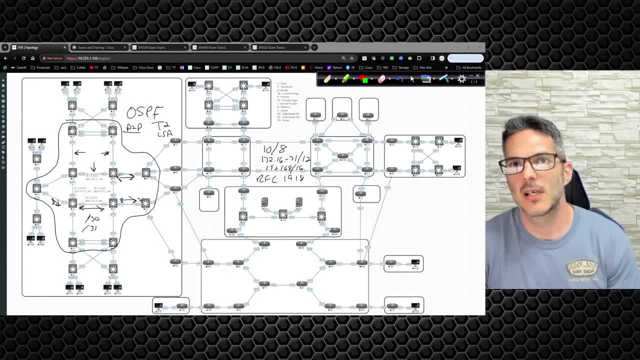 say, in my career I've probably done less than 15 or 20 greenfield deployments where we're starting out fresh and there's nothing already there. most of my career has been some sort of network refresh. so there's already infrastructure there. they're taking, they've gone out capital expenditure, they went out bought. 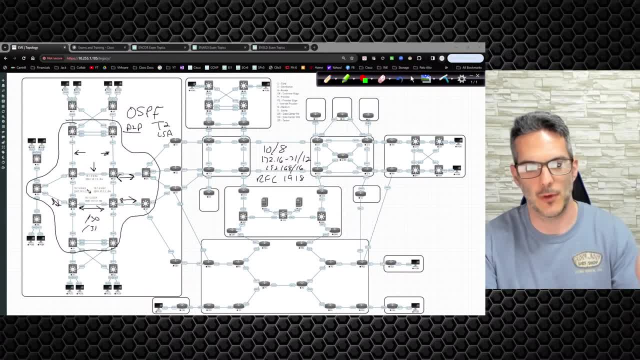 new hardware, they're bringing it in and then my job is to help them go from old to new. So when you look at other things- like not the infrastructure itself, but you're taking a look at it from a logical perspective- what would that look like? 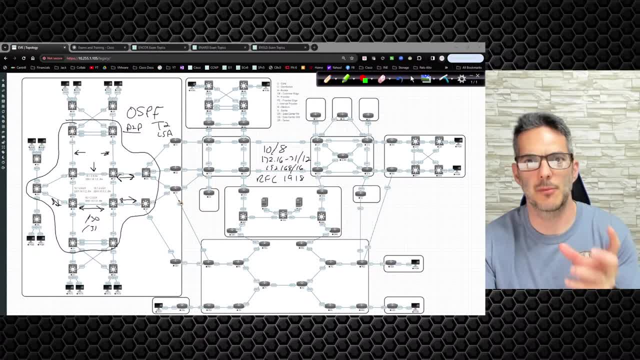 Well, let's say, for example, now on the blueprint for an RC there's DMVPN. Well, the reality of it is, especially with today's architectures, no one's actively deploying new DMVPN solutions, meaning it is the architecture that's chosen over something. 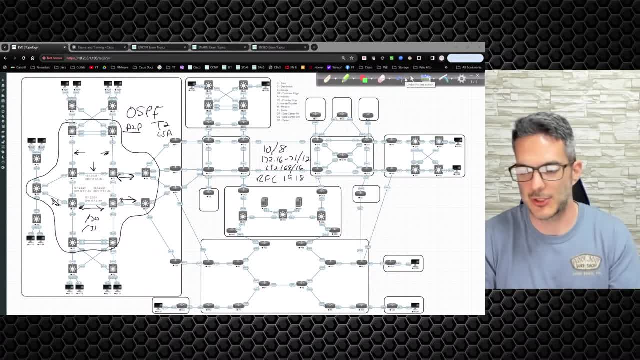 else Most customers are going to be going SD-WAN. That's just the reality of the situation. Not every customer, but I've got several customers right now that have active DMVPN deployments. They've got rolled out and they are looking at getting rid of the legacy hardware, whether 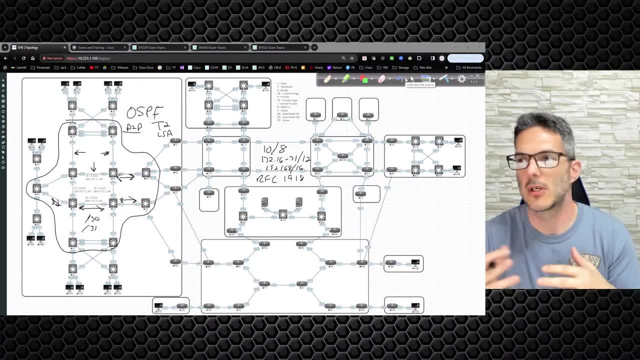 it's been out of end of life or is end of support, whatever the case might be. So when we take a look at designs like that, those are one of those situations where you walk into the environment, you realize they have DMVPN. 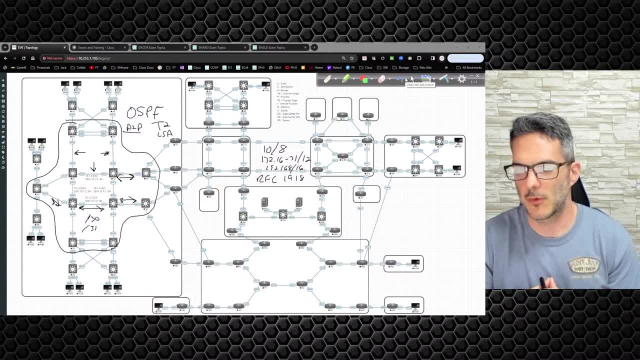 And you're like, oh okay, well, we can work with that. So when it comes to specifically the tunnel, because it's on the blueprint and if we look at this and we scroll down to the bottom here, we're going to see our friend DMVPN even. 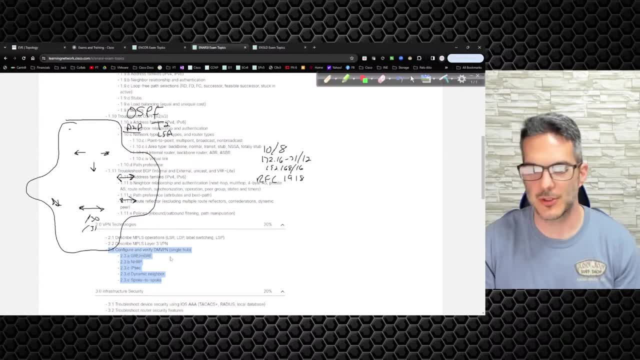 though my overlay is right here. right, DMVPN is on the NRC exam, so we're going to dive into it and cover it because of the fact that we have to. So is it hard to understand? No, Is it difficult to implement? 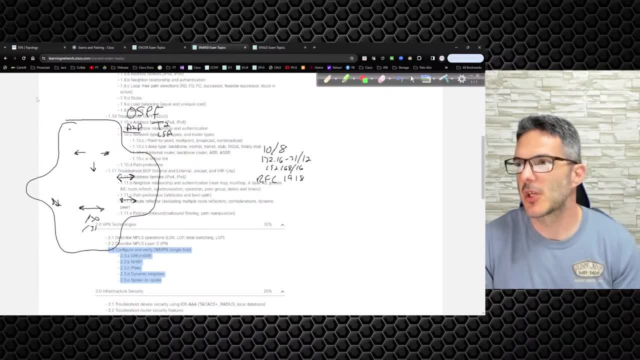 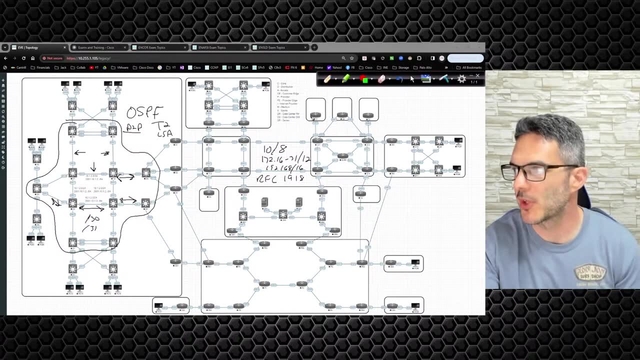 Not really. You walk through a little bit of configuration and you're there. Where it comes into play is, and I purposely built this topology so we would be able to lab it up. We have these spokes spread throughout the entire topology and all but one of them is: 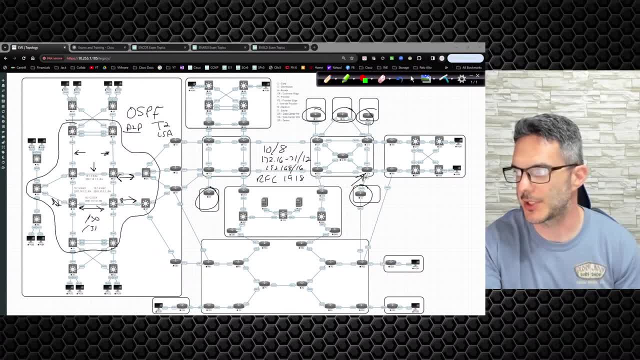 dually connected. What I mean by dually connected is we have a connection to the internet and we have a connection to the MPLS cloud. Can you do that with a DMVPN? You absolutely can. You can have two different clouds if you want to. 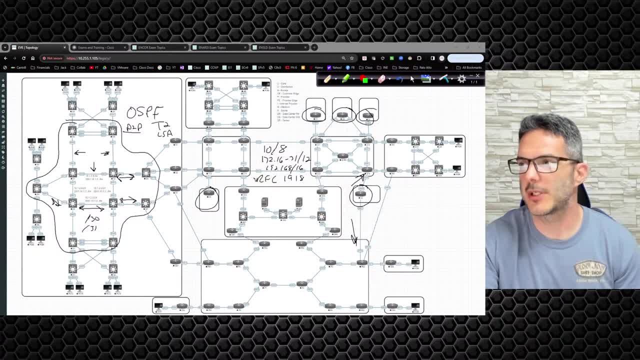 Get from where you want. You can be where you want to be or where you want to go. Now the blueprint says single cloud, which is why, and single hub, So that's why I have a single hub, but you can have multiple clouds. and what's a cloud? 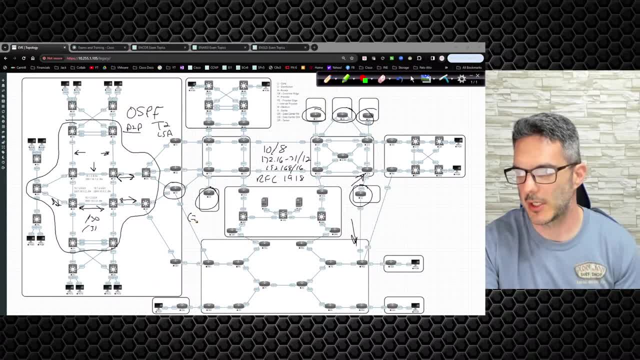 equal to Well, a cloud- I'm just going to draw a C for short- equals a subnet. That's what it really comes down to. So you're going to end up having two clouds so two different subnets. So, for example, you might have 172.31.1 and .3.2.. 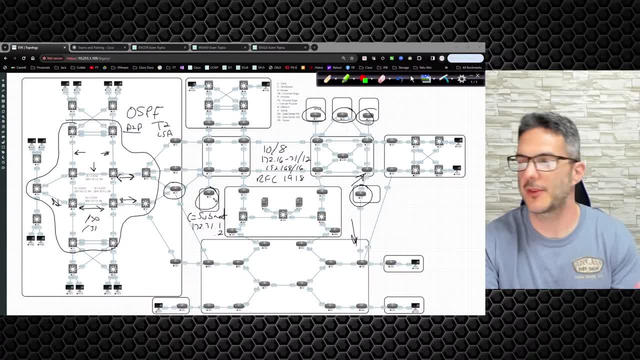 So one might be your preferred path, that might go over MPLS, and then two might be your secondary path and it might go over internet. I've seen addressing structures broken down specifically like that, so that it's obvious which way the traffic is going. 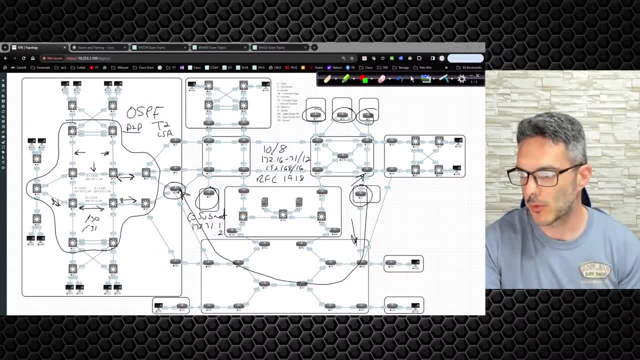 So if you're taking the MPLS path from point A to point B, that's the preferred path, But if all of a sudden you see twos showing up in your traffic, then that's the preferred path. That's the preferred path. 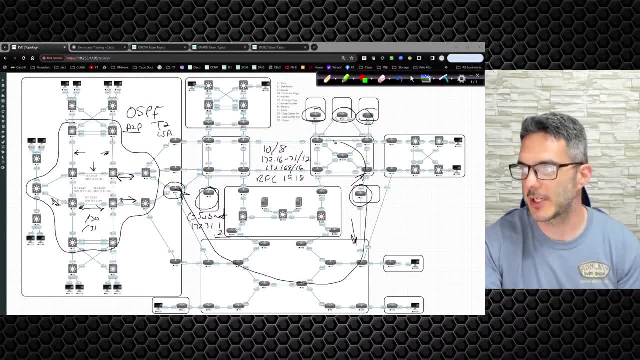 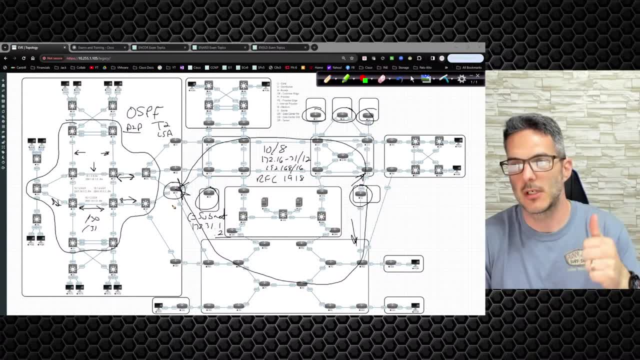 somebody randomly threw something into a spreadsheet and you did a peer review and you're like, yep, looks good to me. But at the end of the day, your job as the architect and the engineer is to be able to look at what they've got going on and maybe put a little bit. 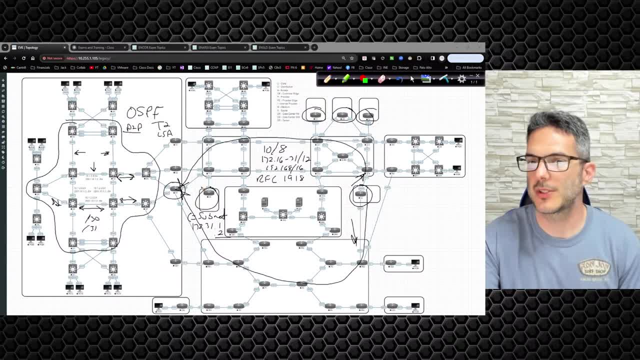 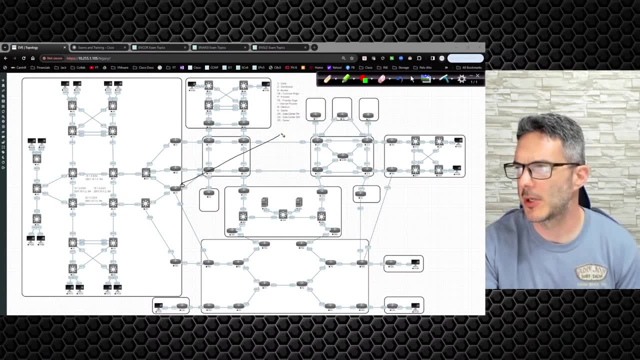 of logic to it. Now, funny story: There was a scenario where- and I'm going to go ahead and clear the screen off- There was a customer that I worked with for a long time where they had GRE tunnels deployed to every one of their spokes, lots of spokes, hundreds of spokes- And I said: 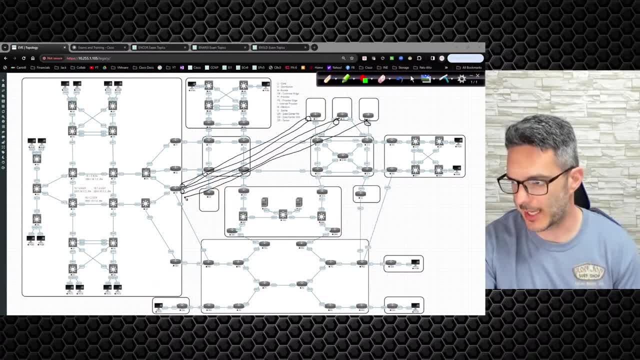 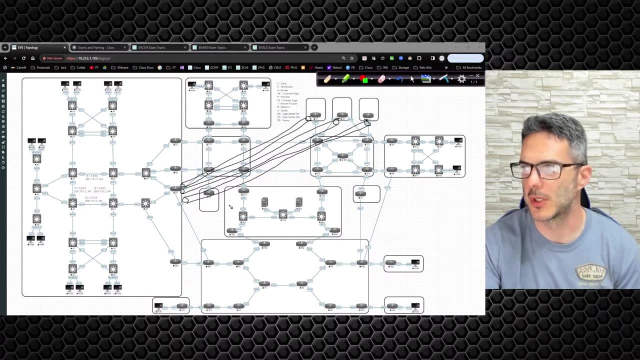 well, why don't we do? why don't we eliminate that and move to a single tunnel, DMBPM, we can migrate over? I put a whole architecture together and migration plan and brought it to the senior guys on my team that had been there for like 30. 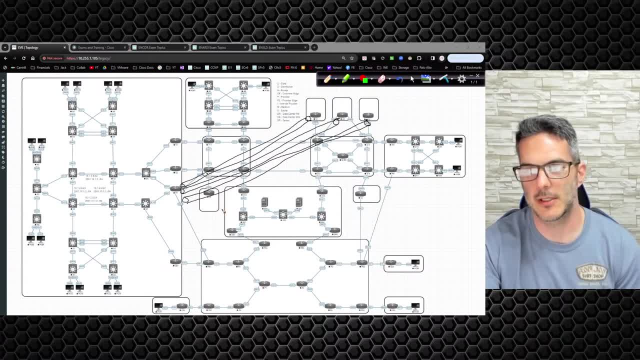 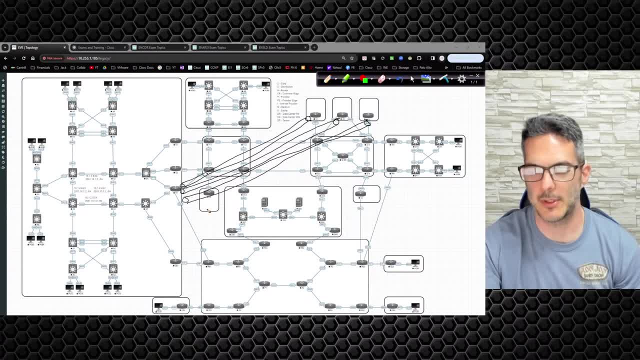 So I started a migration scheme to get away from single tunnels and move to DMBPM, because at the time, DMBPM was a hot topic. Everybody was rolling it out, And we're talking 2014 through 2016.. I was deploying DMBPM probably three or four times a month with multiple customers. So 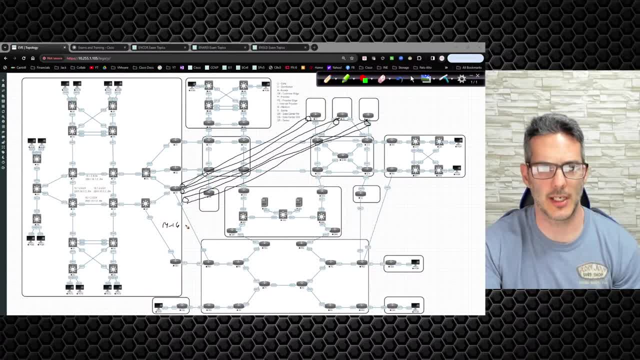 when you're rolling something out that frequently and it's a hot commodity. everybody was deploying it, So it gives you scale right And it didn't matter the routing protocol, I had deployed it. in every facet that you can think of I rolled it out in And that essentially made me the subject. 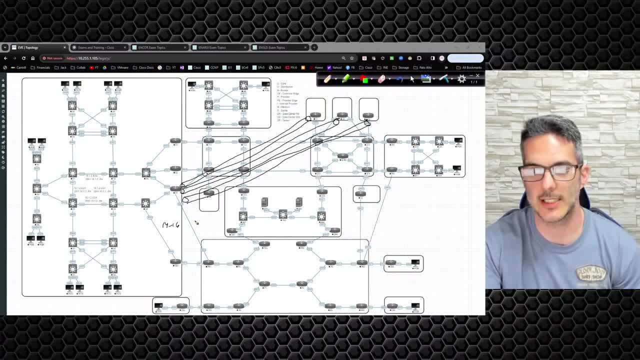 matter expert on it And I became to the point where it was just like I got tired of rolling it out. It was all scripted right. I had the hub config, I had spoke config, routing config, optimization configs. you know Vizio's drawn out for the whole thing, So it brought into PowerPoints. 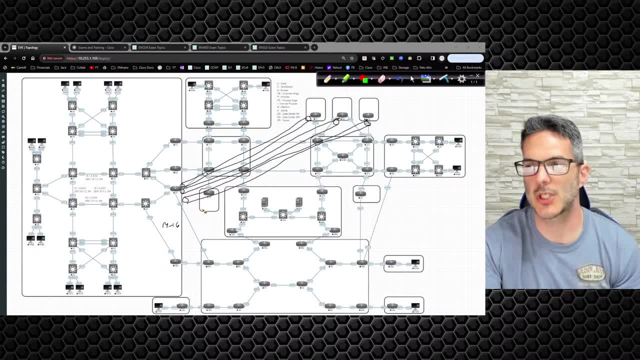 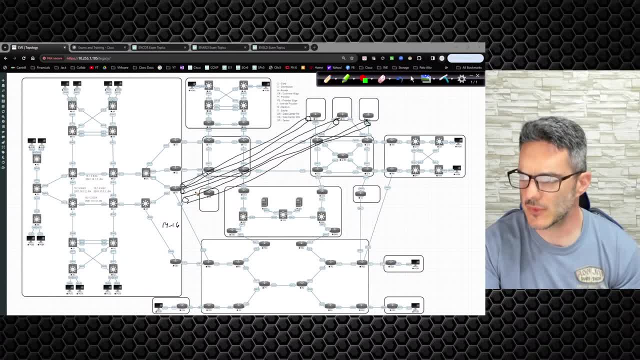 You're going to get really good at it and be very thorough. So what this customer would do is they needed to be able to- one of the things that they did was kind of funny- To control their routing, because they did EIGRP everywhere to control their 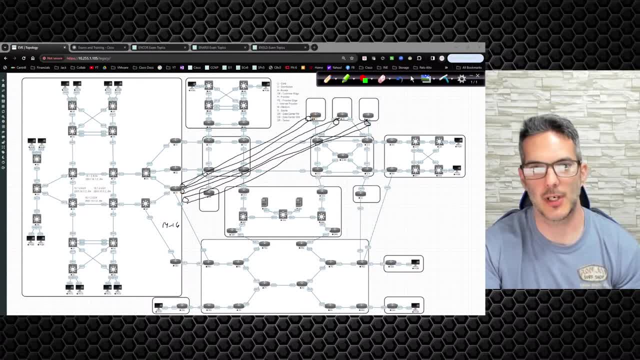 routing they would do. every location had its own autonomous system number. So what they would do, let's say: this is autonomous system 101.. And this is 103.. This is 104.. This is 105.. You get the point Over. here we're going to say this: is you know one, what they would? 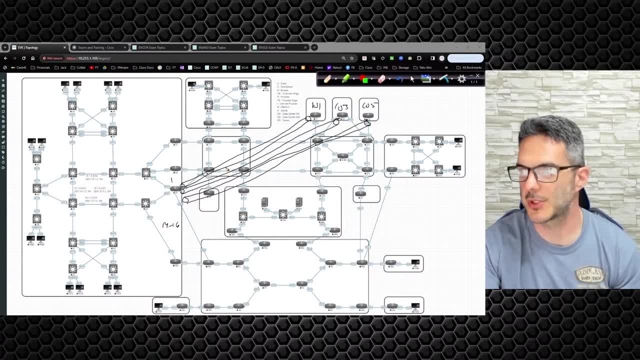 do is over the tunnel. this would be its own autonomous system number. let's say 11, we're going to do 13. And then we're gonna do 15. And what they would do is they would redistribute between their autonomous system numbers. totally valid make gets the job done, so that they would 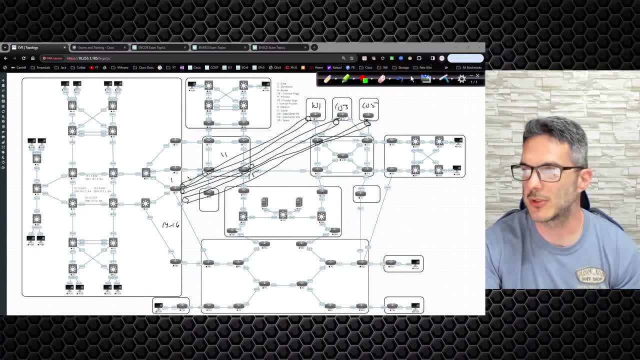 be able to do route leaking between their locations And then they would do between the route, between the redistribution statements. they would create prefix lists that would be called from route maps And that's how they would control the routing If they needed to leak something through. 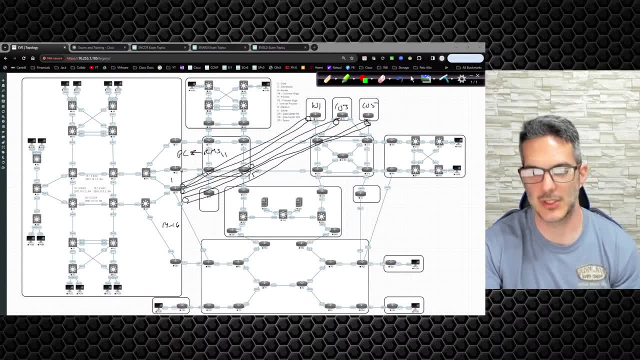 they would add it to a route, a specific prefix list and things like that. So what they would do is they would have these autonomous system numbers- let's say 101 to 103. And what they would do is they would create these route maps, they would be able to control the routing, And then they would 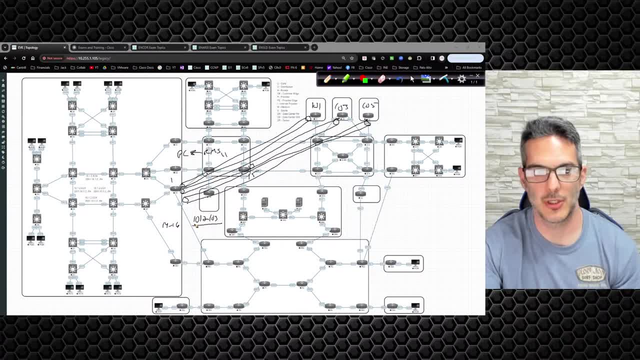 be literally mapping which traffic was going to which And 103.. So 103 to 101.. So was it a little harebrained? It was. it took me a while to understand their routing design, But they had ran it poor design And this is a classic example of why it's important to think through your. 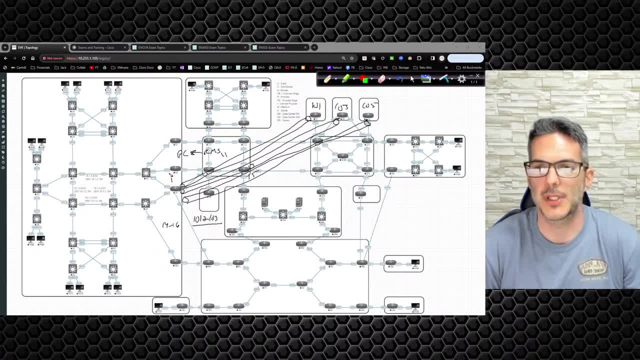 addressing architecture and how you're moving forward with it. Because in this particular case, I'm sitting there looking at their- their addressing structure, their addressing design, and I'm trying to understand how they're making all this work. I had never seen anything like it done before, So I was a little taken aback when I first started. 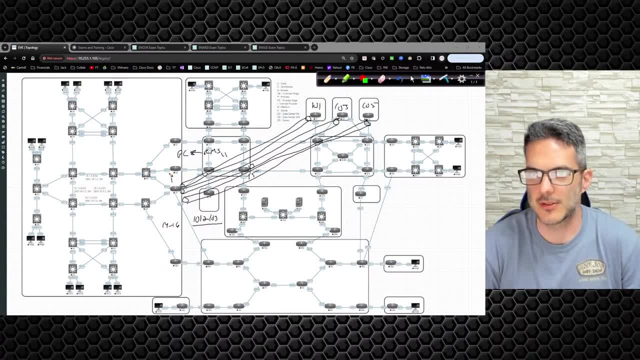 looking at it And it wasn't until I took the lead engineer and I said This is what I'm seeing Like, does this make sense to you? And I literally had like write it all out to try to make heads. 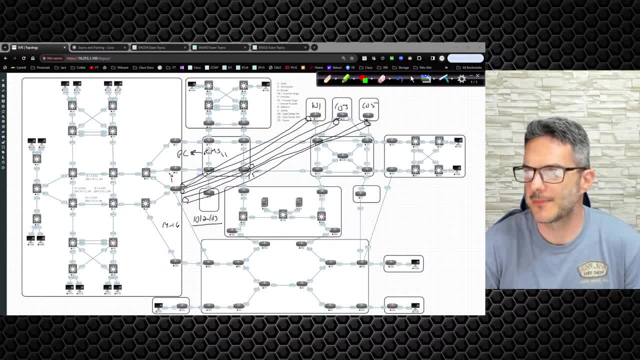 or tails of what was going on. It was very, very confusing. So now, mind you, I was a pretty newly minted CCIE at the time, So we're talking to 2000,, late 2015,, early 2016.. So I was looking at this going: wow, this is, this is messy. And so what I ended up? 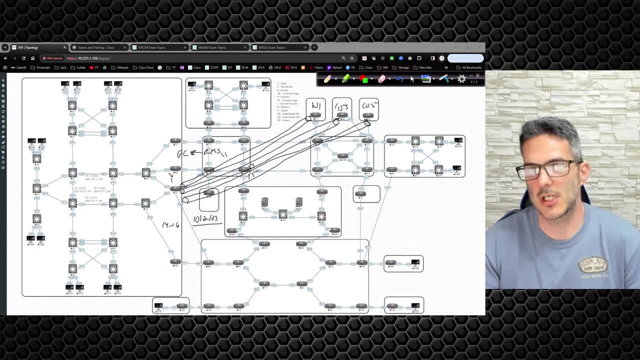 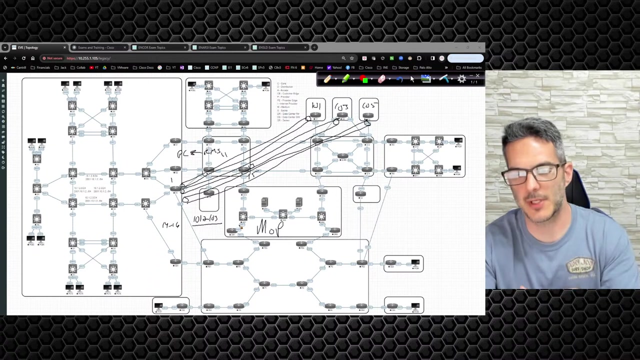 doing is I rebuilt their entire design inside of a lab And I come, I came up with a in the value added section from the ソ, the, the pieces, the configurations, the devices you're going to be touching, the show commands, the verification commands- all the things needed for your change window is going to. 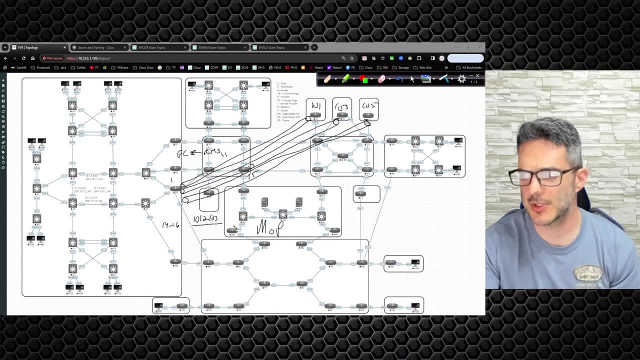 be built into this spreadsheet And that's what the you guys are hearing me talk about. this, for This is your 8020.. Where are you? Where are you? so I'll see this part. I'll be shown a little bit so it's not a lot of noise. I don't know if you can hear me from the bottom of the camera. 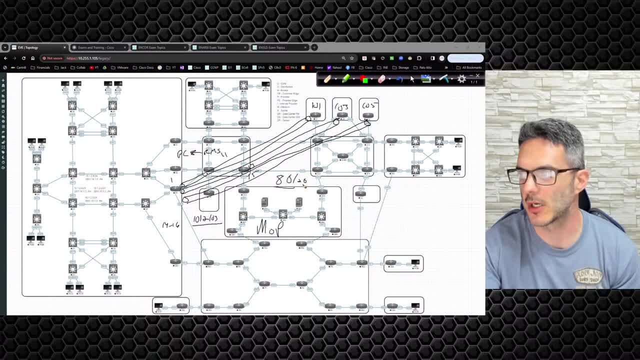 rule right, You're spending 80% of your time doing that kind of work, So the other 20% of the time your actual change window goes as smoothly as possible. You've labbed it out, you've tested the migration strategy, all of these things, So essentially I ended up building this out in a lab. 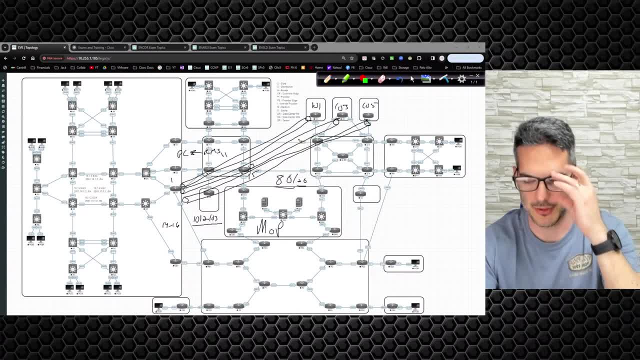 in GNS3 back before I started using anything else. I got it and I fully documented everything. I had all the things broken out and detailed out so that when people would question stuff I'd be like, yep, got that covered over here and I would go into the details. The intention was to have it so. 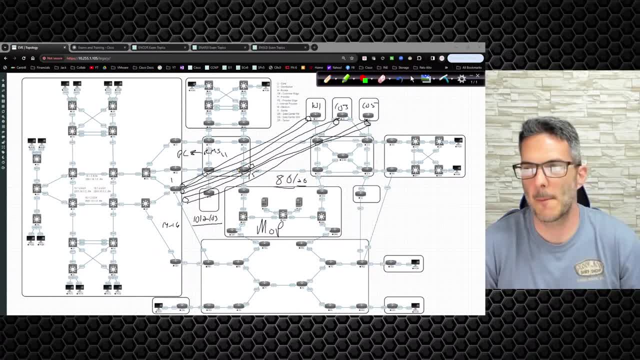 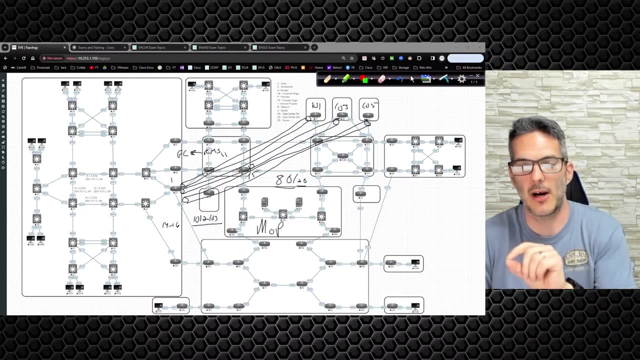 well laid out that, no matter who was asking, I was like, yep, I got a solution for that too. Now, early on, I would get some feedback And it would be like, oh well, maybe I okay, I hadn't thought of that, So I would note that down. 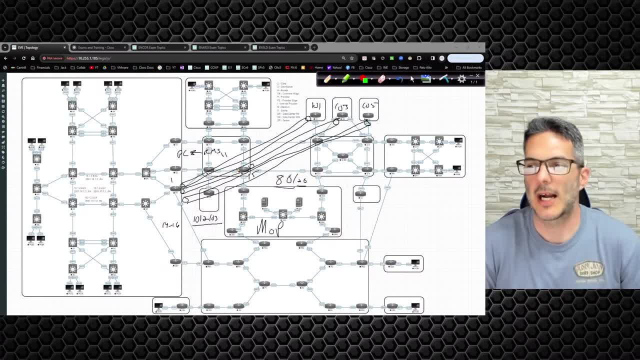 and I would go dig into it until I figured out the problem. So I got to the point where I had everyone in the room shaking their head up and down, just like this, like okay, anybody have any objections to what it is that I'm proposing? And I got they were like nope, we're good. And 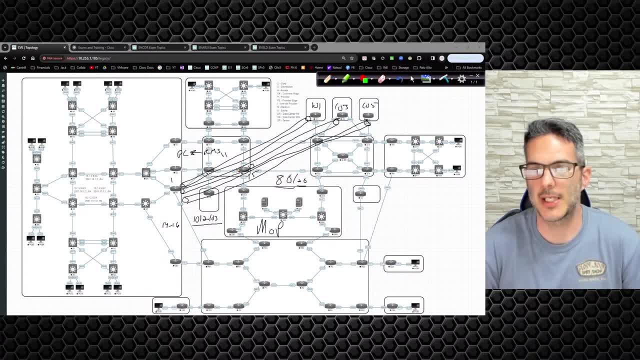 I had it all laid out and it was just a matter of time to get a change window to be able to do it. It took about five months And I can. I'm not, I don't have, actually I don't have time in the next 35 minutes to break it all down to you, But 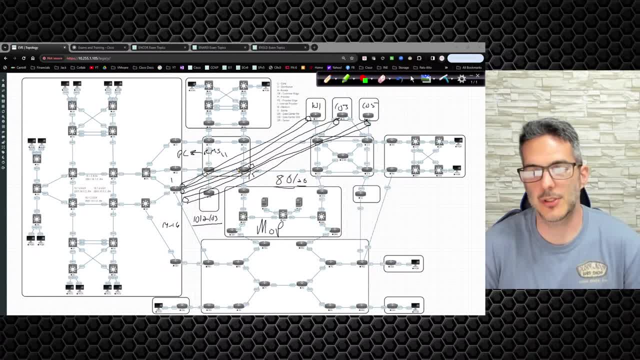 essentially we went through the process and it took us a month and a half of every week, for two days, Tuesday and Thursday- to do a migration. It was Tuesday would stand up the new location and get it where we needed to go, And then Thursday was the cutover And there 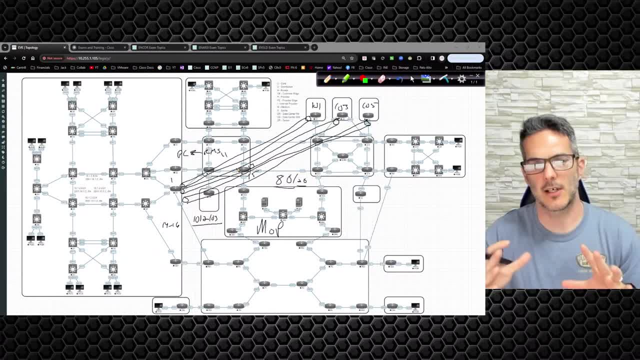 was some routing that we had to do And we did it: a couple small sites where it wasn't going to be as impactful, just to have that warm, fuzzy feeling that things were going to work out the way that we wanted them to. And we eventually 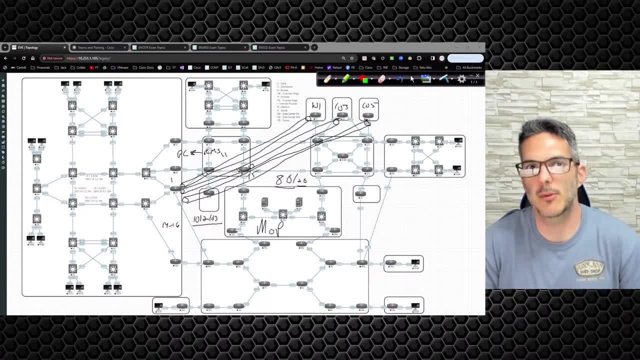 ended up moving everybody over all the sites somewhere in the neighborhood of 400, if I remember correctly, 400,, 420, something like that of getting them all migrated, And once we had a locked in and validated method, we were able to get them all migrated And we were able to get. 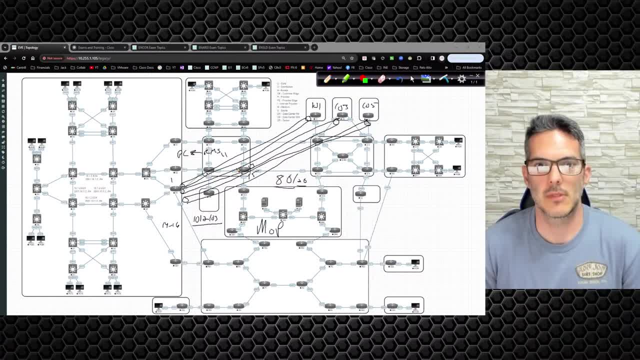 them where we wanted to go. We were able to do 30, 40 sites a night. It wasn't hard. It was more time consuming logging into these devices and standing up to config. And then we had notepad docs. It was me and a few other engineers that were working on this To log into these devices. 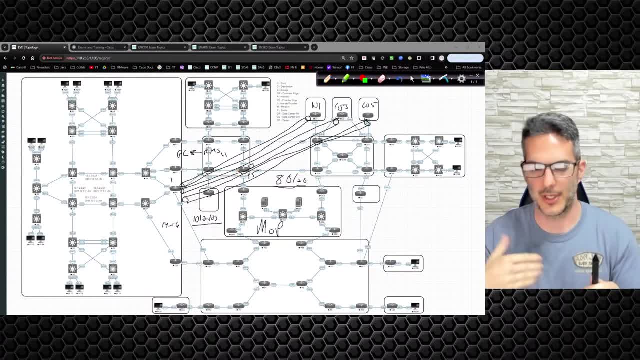 it was like a divide and conquer: You handle 10, you handle 10,, you handle 10,, I'll handle 10.. And we had a little lockdown And we were all on the same conference bridge. a WebEx like okay. 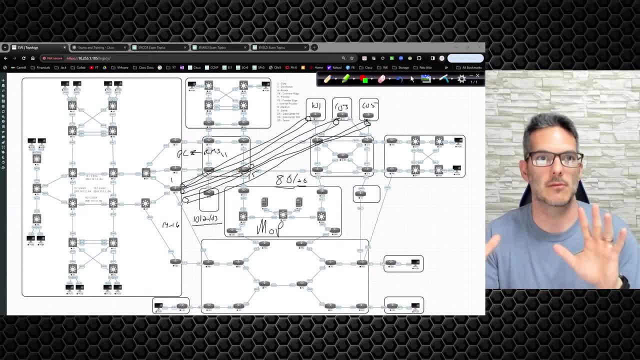 I'm doing this Like okay, cool. So you know, we were able to do 30, 40 sites a night, And we were able to do 30, 40 sites a night. And we were able to do 30, 40 sites a night. It was a communication. 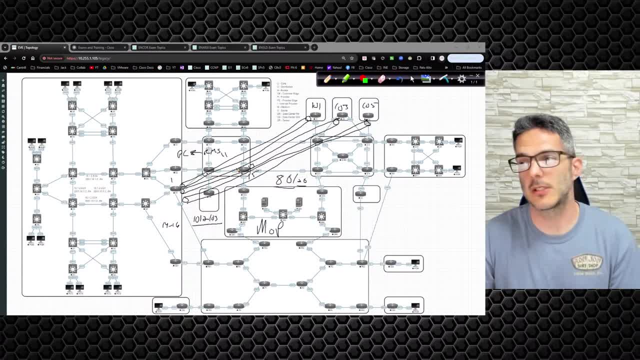 orchestra, if you will. But by the time we got it all said and done, we had migrated 40 sites in the course of a couple of hours And that was the, and we were validating the routing. You know, we'd make our change and we'd have an app person or we'd have somebody on the phone system verify. 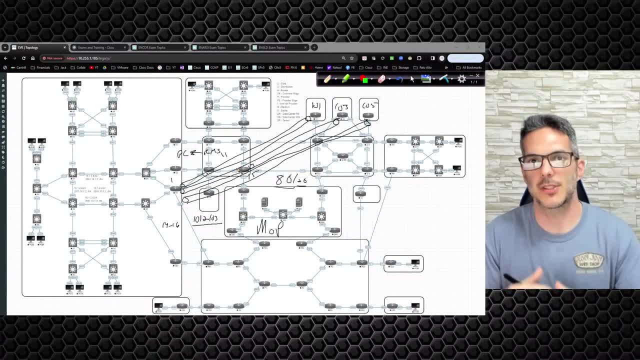 the phones were registering whatever it is on the back end that was necessary, And those are the things that you had to take into consideration is spoke to spoke communication, So it took a little bit to get it there, But once we got it all done we were able to do 30, 40 sites a night And we 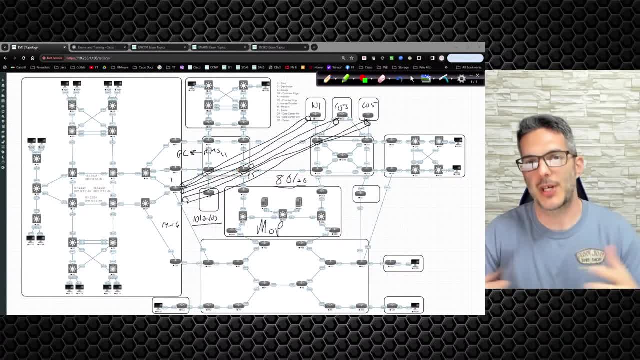 were able to do 30, 40 sites a night And once we did the work kind of built on itself And it was in. it was a pretty solid migration. And there's a comment in the chat, Let me go grab that real. 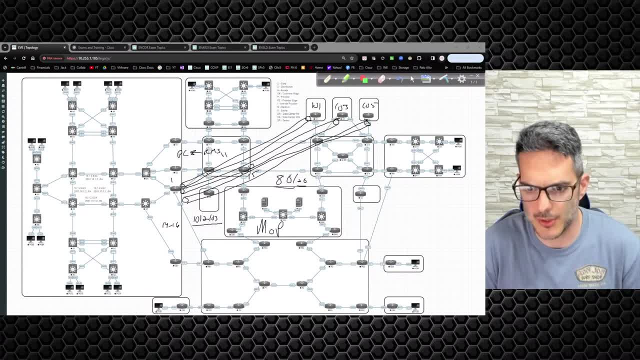 quick. I just noticed it. Hi, Rob, keep up the good work. I know this meant to be Encore and Narcy Focus. Is it possible to add firewalls, SD-WAN? It's also could be real world network. So yeah, we're gonna do that in the, so that's something that I'm planning on doing as well. 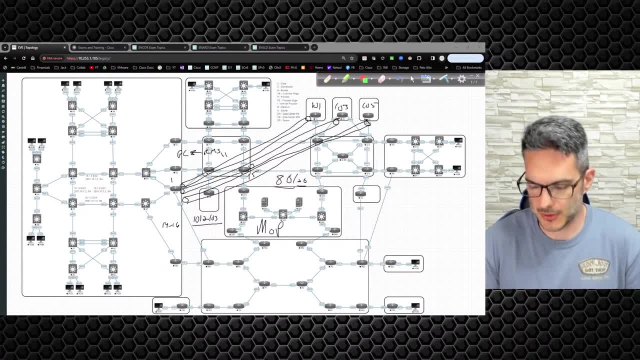 Real world networking is going to be its own focus. The topology you see right now in the live stream is going to be specifically for Encore and Narcy, like you said, but I have another topology on another server that's going to be specific to real world networking And I'm actually thinking 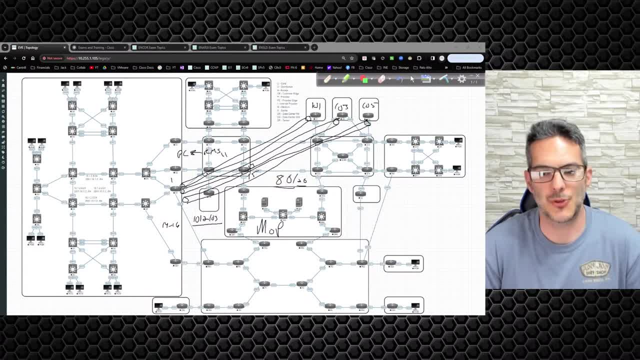 about making it a live stream, kind of thing. I still have some stuff that I have to work out, but I'm kicking around, I'm going to do a little bit of work on that. So I'm going to do a little bit of work around some ideas. So that one here. actually, let me see if I can't pull that one up. 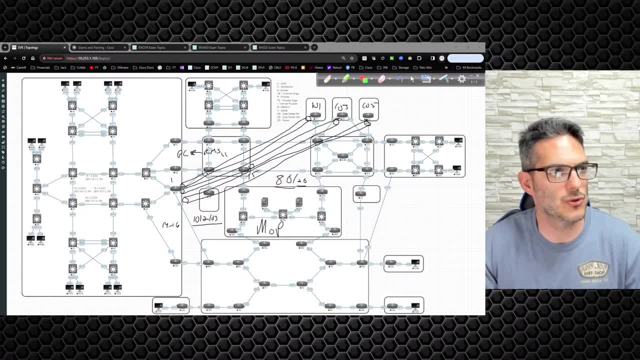 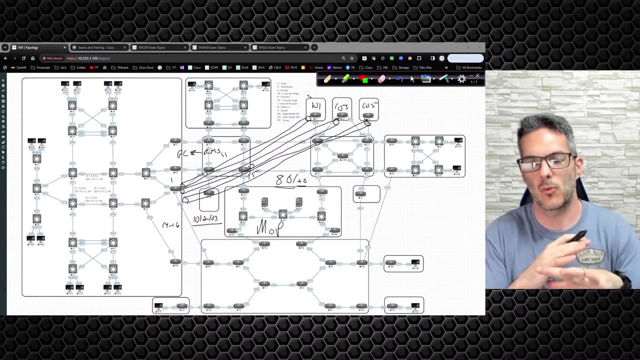 real quick, Just so you guys have a visual. So, but before I do that, let me just finish up my point here. The cool thing about it was when the addressing scheme was. by the time we got everything migrated, we had one big subnet for everything. Well, I'm sorry, not one big subnet. 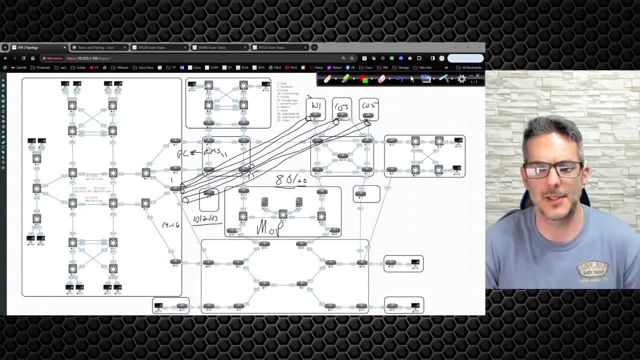 It was because we had a slash 23.. And the cool thing about it was, if we needed to grow that out, it was easy to migrate to another tunnel, And that was another thing that I had worked out. So we had 400-ish sites. So I 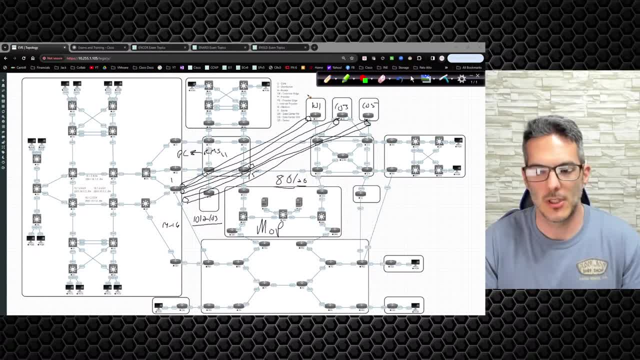 automatically needed a slash 23 to get the job done. So if you need to go at five, six, 700 sites, you would just need to have your addressing size done appropriately, So you'd have to figure out your subnetting. So a slash 23,. 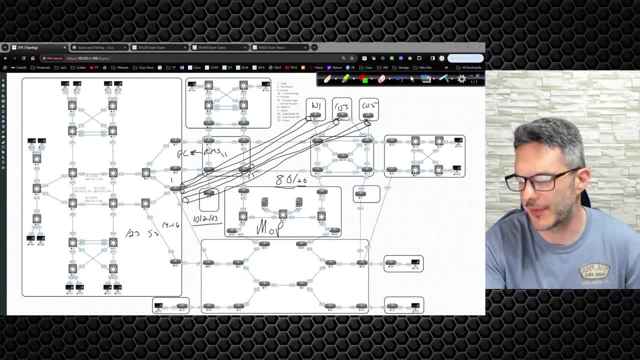 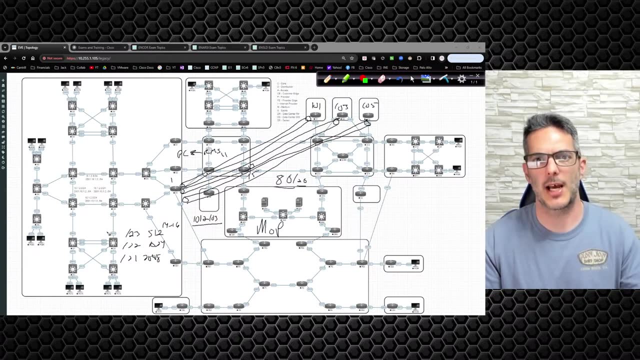 is 512, I think, Minus you know three or four, And a slash 22 is 1024.. Slash 21 is 2048.. So you would just have to do your figure out how many spokes you're going to have on your DMBPN. 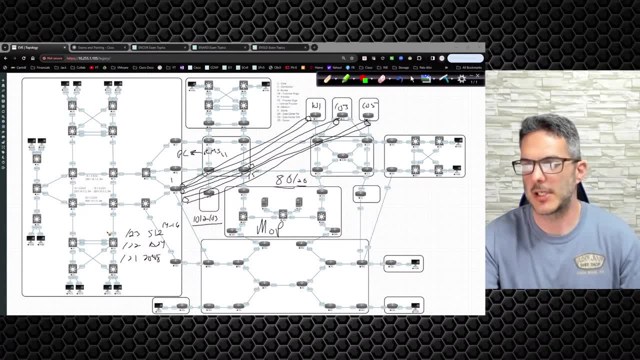 deployment and then build out your size. And when you get to this size and below or smaller subnet sizes, or should I say shorter masks, shorter mask sizes, you're definitely going to be doing BGP. You're not going to be rolling out EIGRP for a deployment of that size. So now, one of the reasons why you 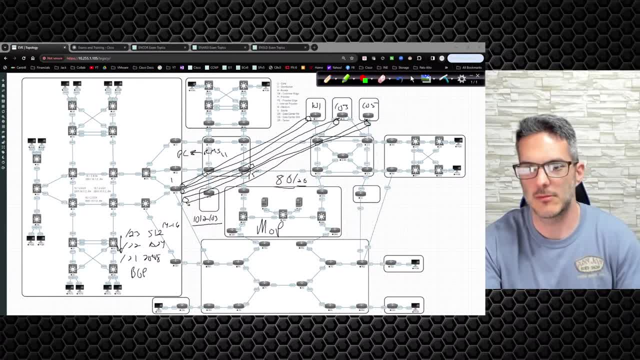 would want to do. that is because, when you're looking at it from an addressing scheme perspective, these are typically going to be something you're going to lay out in the spreadsheet, detail out what site's going to have what, and you become kind of a wizard, if you will, of. 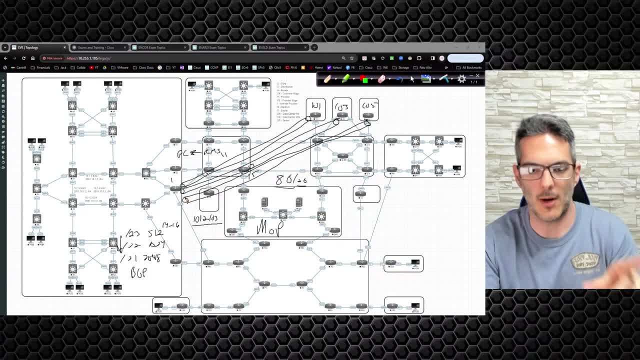 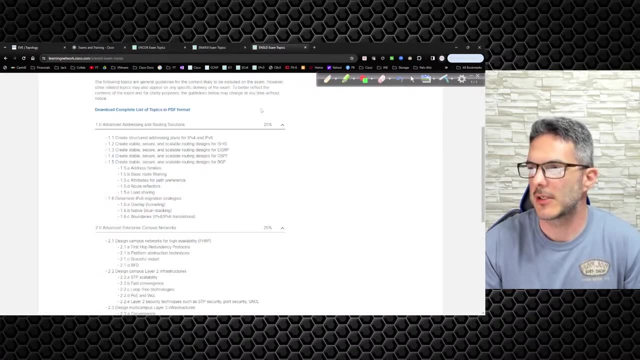 Excel spreadsheets because you're spending so much time doing the dot one, the dot two, the dot three, the dot four, you know, so on and so forth. So that's where that comes into play. Now, if we look at we go back over here to let me clear the screen off- If we go back to the design structured, 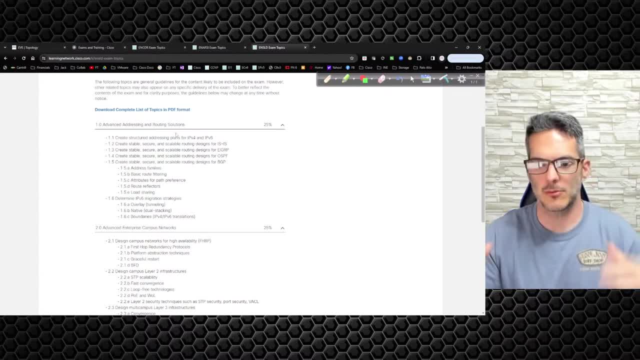 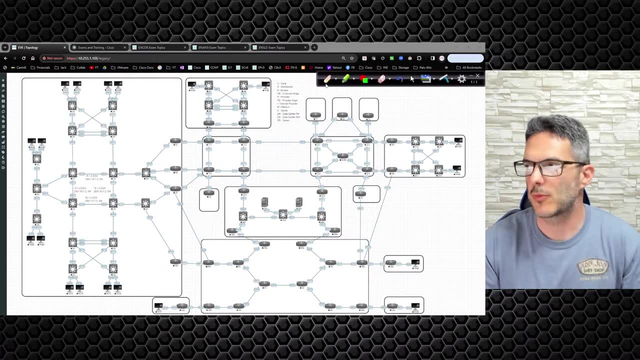 addressing plans. So if you're looking at it from the at a high level, you want to keep in mind that a addressing scheme should always start with your biggest first and then work its way down to your smallest. So I did see one scenario where a guy had done an addressing scheme. I think it was a 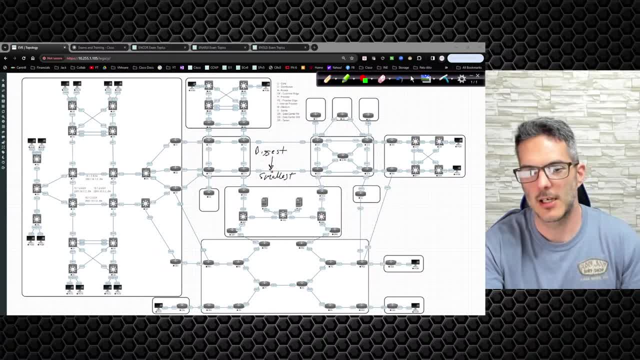 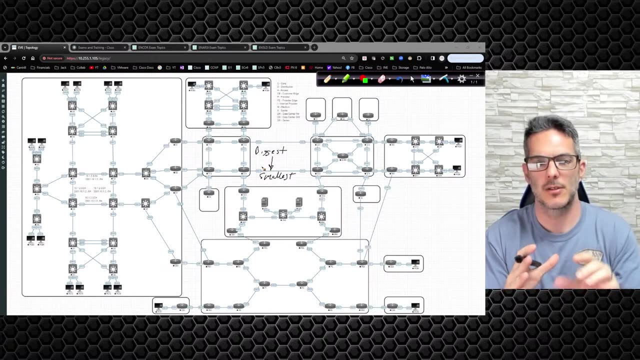 slash 16, and somehow he ended up picking on the. he ended up picking one slash 24 that was smack dab in the middle, that he had to like break out to one big supernet, into two smaller supernets, And then to peel out that one slash 24 that he used. 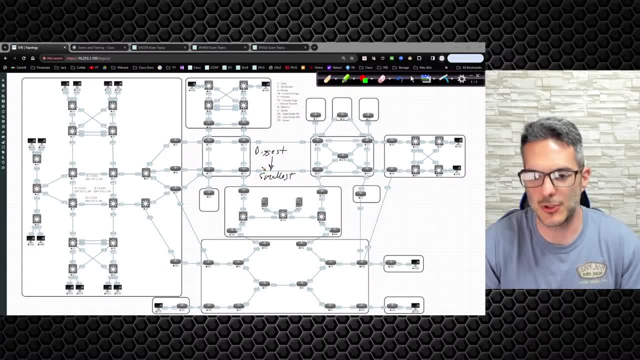 because of the fact that he had overlooked the fact that you couldn't use that specific IP address or subnet range in that particular use case. But that was. it was a definitely a day of looking at subnet masks and trying to figure out the bit placements and stuff like that, and 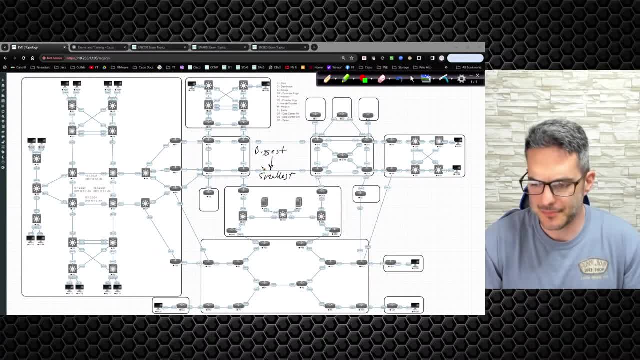 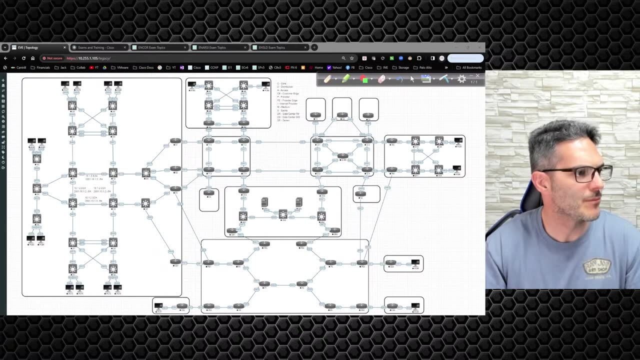 taking me back to the CCNA days, But that's where that really comes into play. So, when you go ahead and knock out this thing real quick, I think it's this guy right here. Let me log into the server real quick. I think it's the server, Yeah, right here. So the real world networking topology that you guys have basically just downloaded from Microsoft is going to be in that third page right here. From there, you're going to be able to come out and you're going to be able to see something that and it's going to show you the 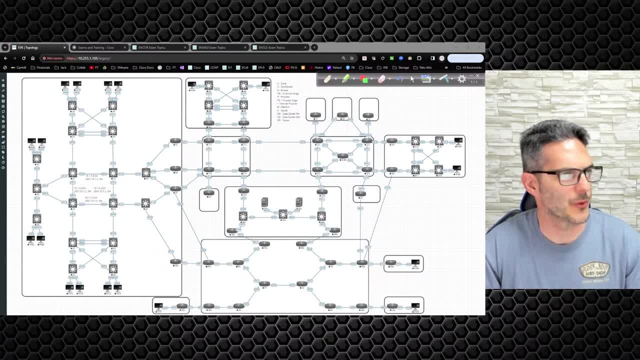 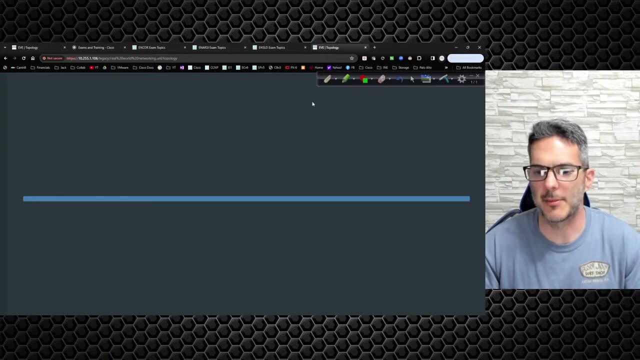 So the real world networking topology that you guys have seen, I'll go ahead and open it and I'll bring it over, because this thing is kind of ridiculous, Just like that And it's going to take a minute for it to load because it's so big. 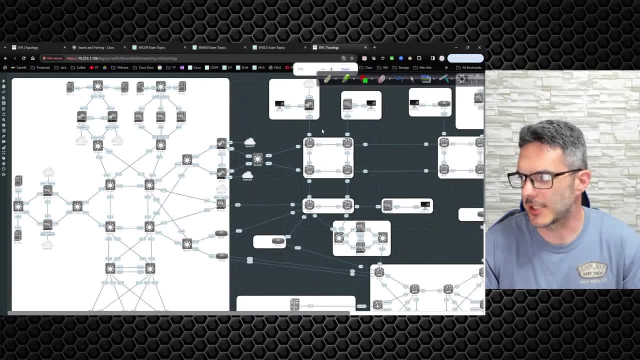 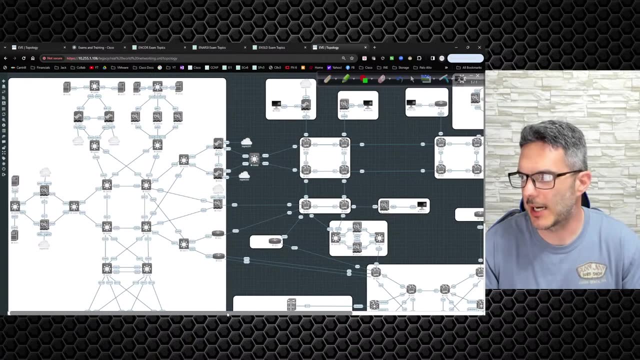 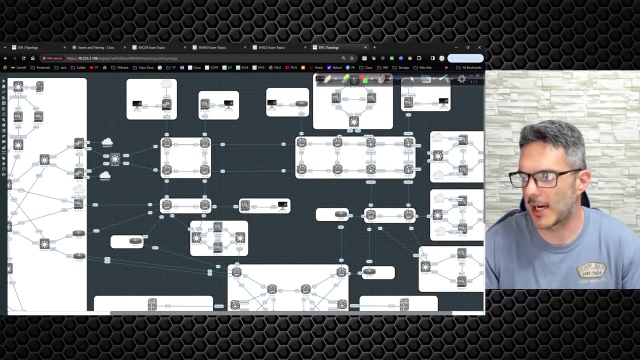 So the intention behind the size of this thing is to mimic what you would potentially see in a real world design. So we have our HQ location, and then we have our internet sites that are a combination of iOS and XR and a bunch of other stuff. 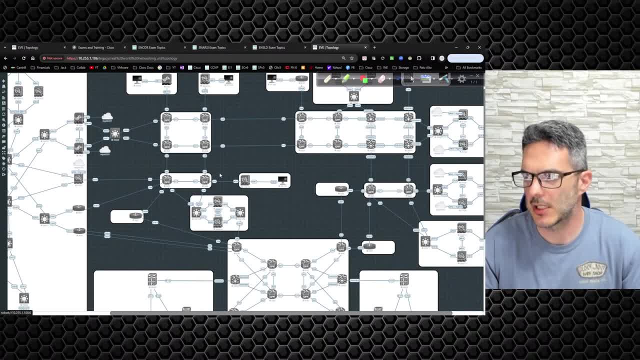 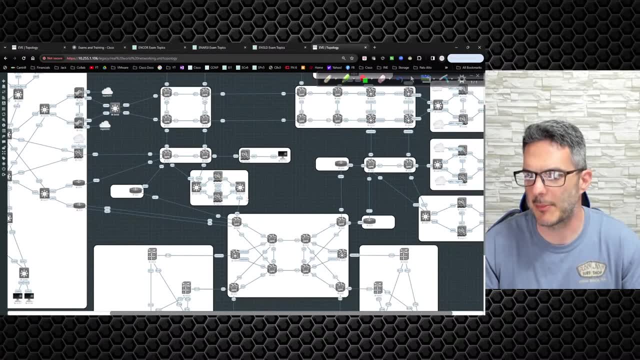 And then down here I happen to have a colo facility that if you had a user working at home they'd be able to SSL, VPN to the firewall and then they would be able to hop in and to the MPLS core and then be able to go wherever they want to do from there. 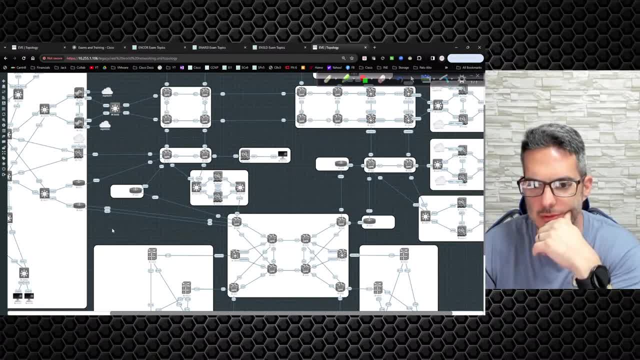 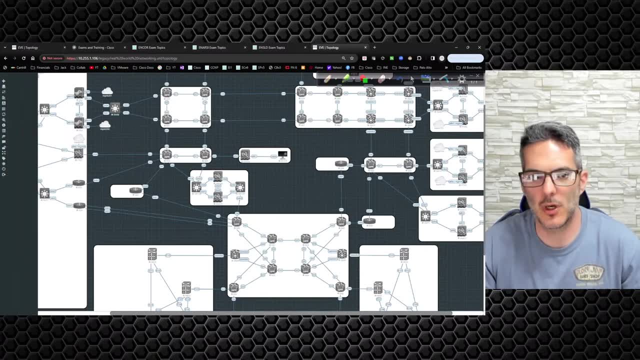 Teams versus YouTube. I'm pretty sure that. Oh, no worries, Tex-Mex appreciate that. man, If you are interested and you want to get a more reactive time- I'm not sharing my screen through Teams- but if you want to jump into Teams, maybe that's you, Dave, I don't know. 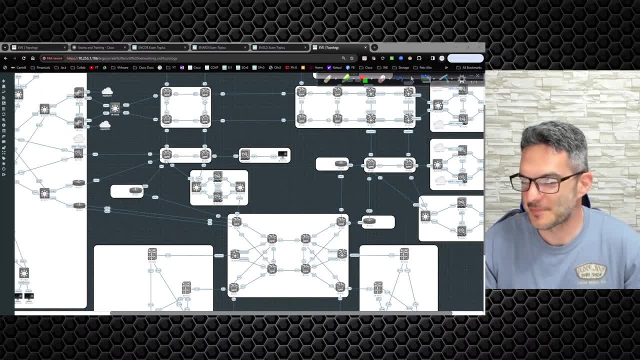 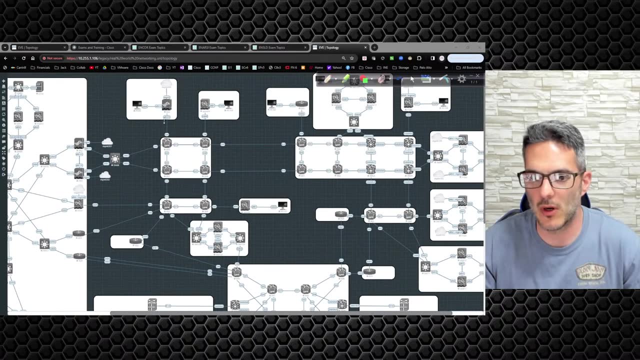 I don't know, I don't know. But yeah, it's a little bit slow. if you're on YouTube live, there's a little bit of lag, for sure. But to your question, Musab, I definitely do have a lot of firewall in here. 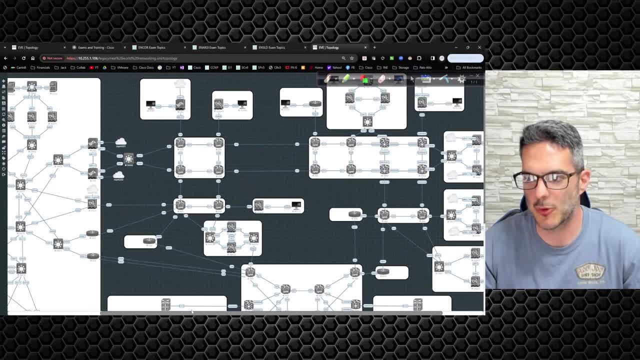 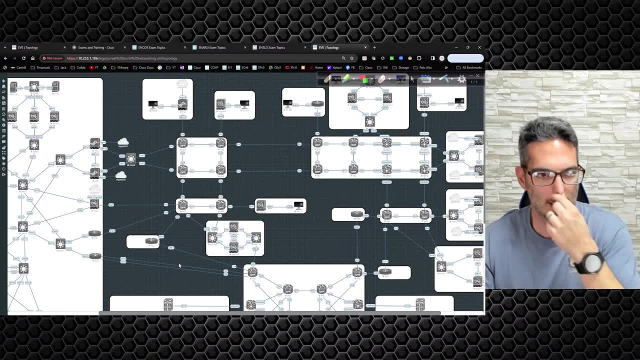 I hadn't thought about doing SD-WAN- though It's one thing I hadn't brought in and nothing says I couldn't try- but that would require me to ingest all of the catalyst SD-WAN. Okay, And the reason why I would do the catalyst SD-WAN is if you look at the CCIE version, 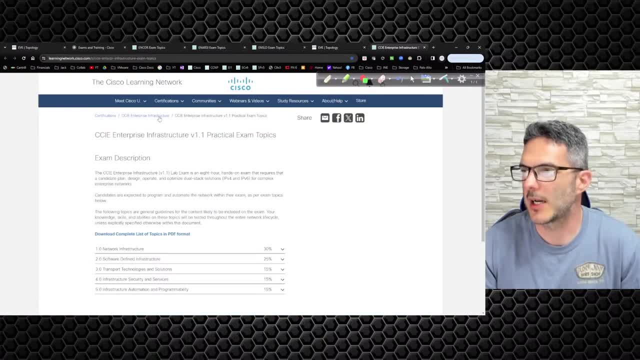 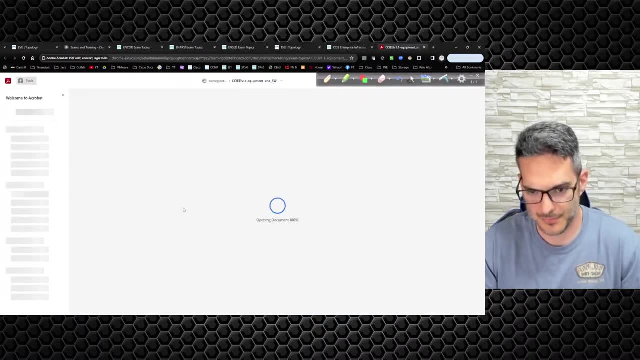 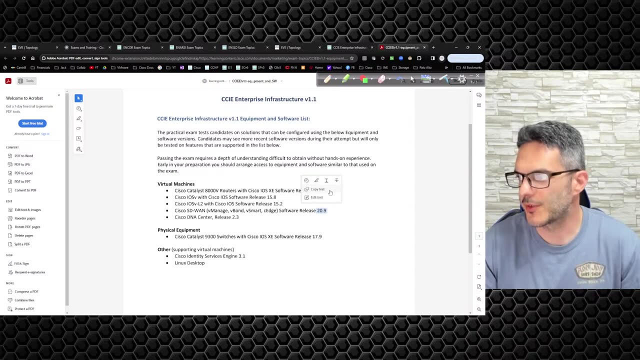 1.1,. let me go ahead and pull that up real quick and then look at the additional resources and the equipment. in the software list we have 20.9.. So as far as I know it, that is going to be catalyst SD-WAN, I believe. 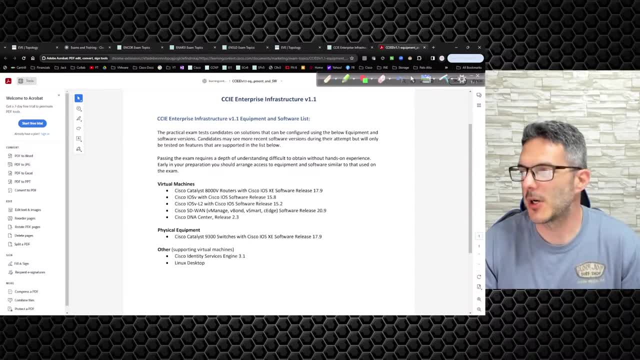 Don't quote me on that. Maybe I'm wrong, but that's the version of code that I would. I did 18.4 on the SD-WAN series that I did the first time, So I would just do the update on that. 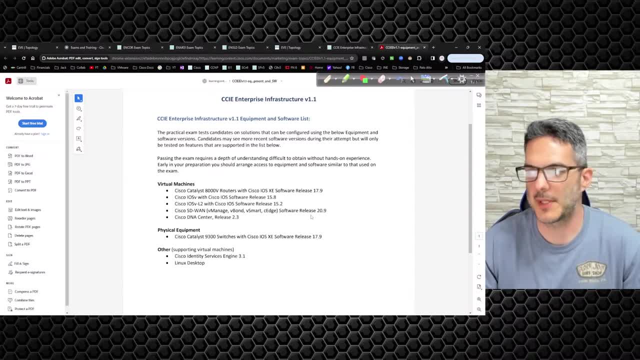 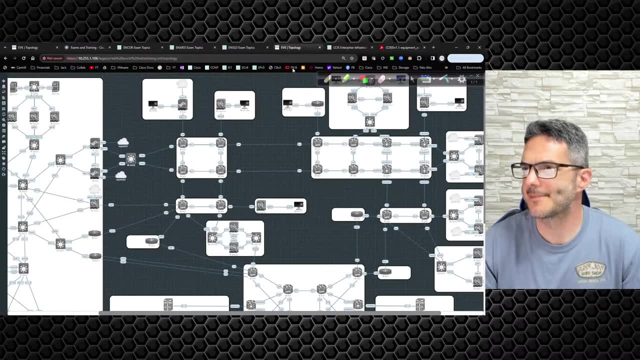 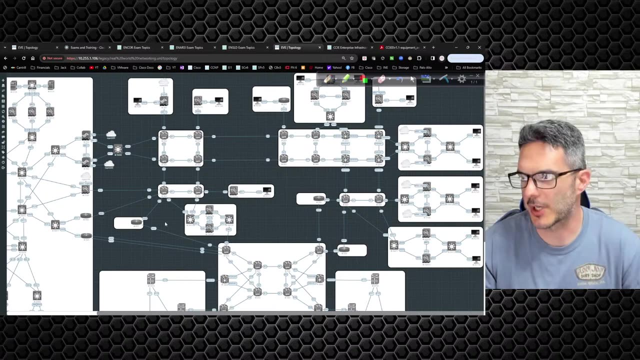 I haven't had a chance to go through the details on it, but that's where I would probably spend my time- going through and spending my time there. But the topology is built intentionally big And we could use this topology too for reference If we were looking at the capability. let me go ahead and go to light mode. 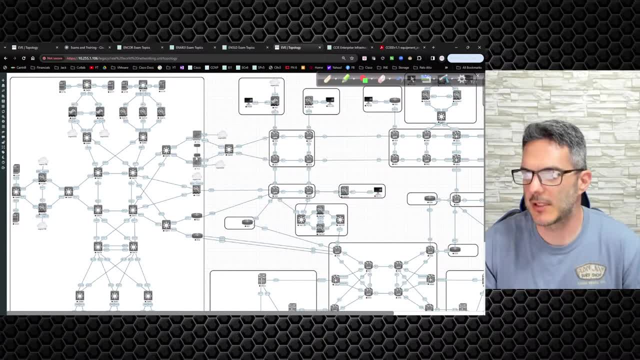 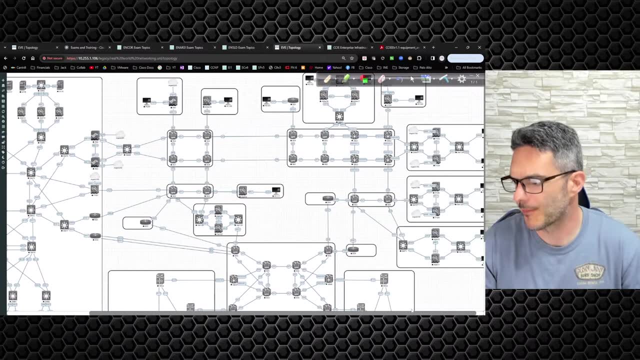 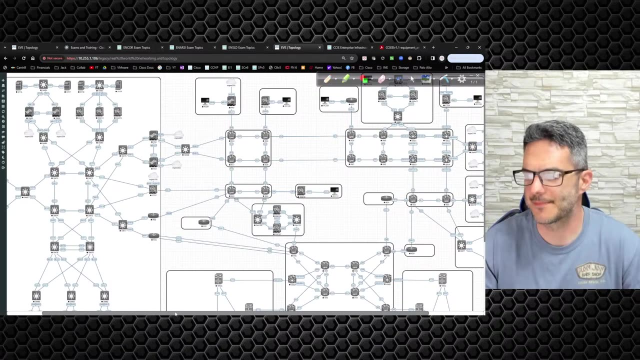 So this one was built out with FTD Palo Alto- regular ASA. I got ASA somewhere else in here- Regular ASA. actually I think it's over here The ASA that's meant to allow clustering. and then ASAV does your typical SSL VPN and any. 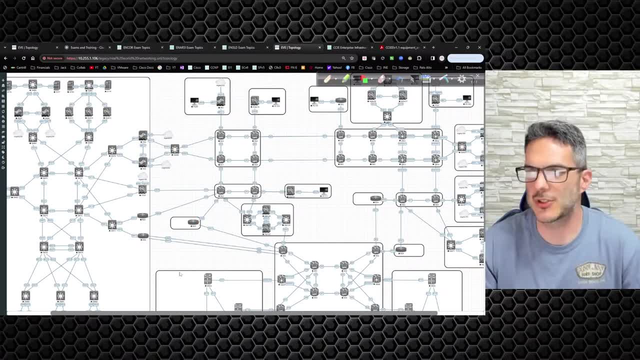 connect and things like that. So that was the intention behind that, because part of what I want to go do is be able to develop a bunch of workbooks and things like that. That'll be A. I'll be able to learn a bunch of different firewall platforms, a bunch of 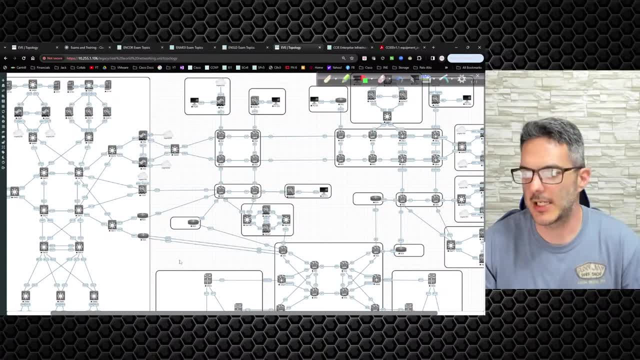 different operating systems and things like that, And it'll just make me that much more efficient as an engineer. So that's really the goal with how that comes into play. So the, If you see, like a switch 73, that's actually not going to be called switch 73.. 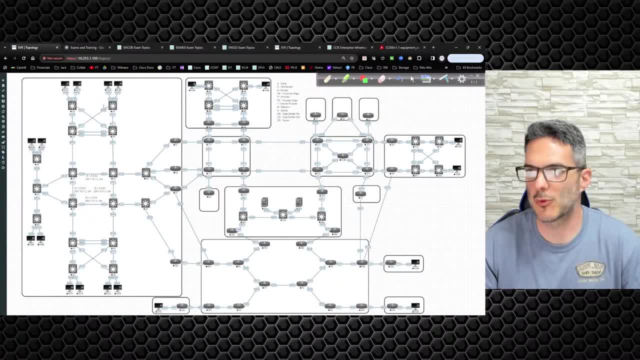 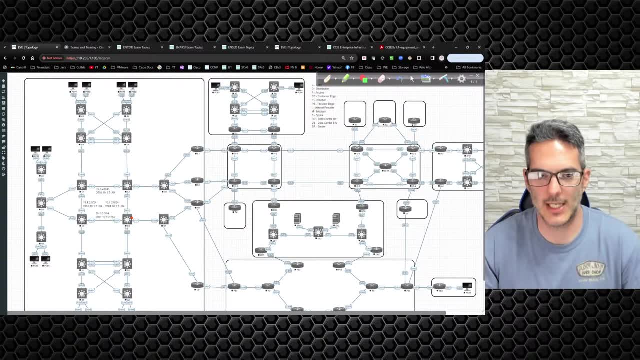 I'm going to rename all this stuff to have much more of a closer addressing or designed to be like this: core one, core two, core three, core four, things like that. So it's much more. It's easier to follow if you're. 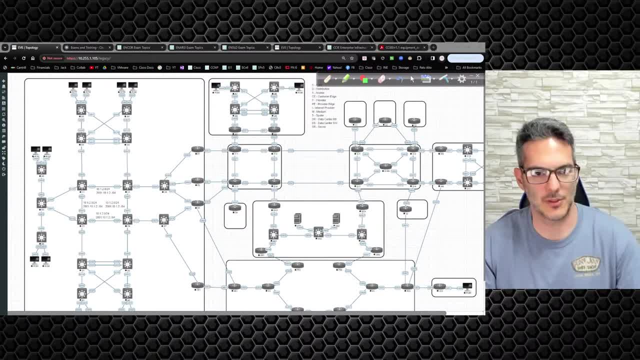 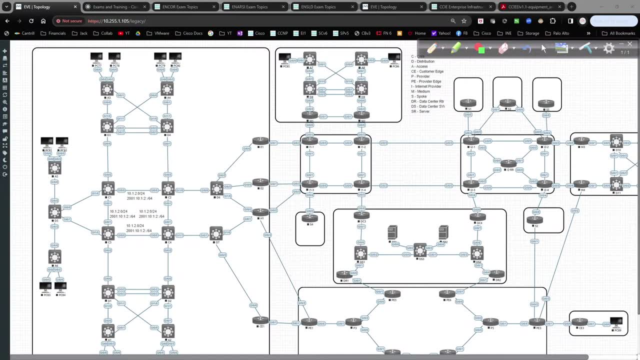 My video is getting all goofy. Let me go ahead and turn that off real quick. as far as escape, there we go, So hopefully that'll. There's a little bit of lag and then the video on my camera is starting to act up. 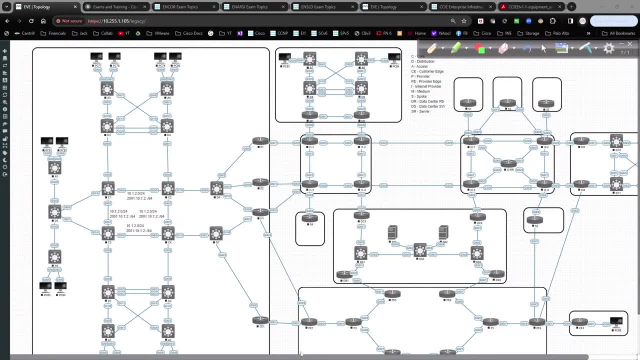 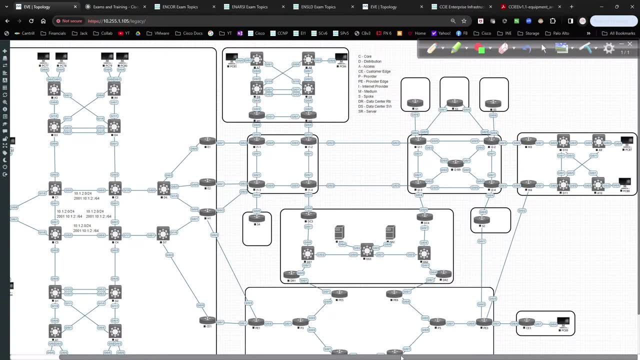 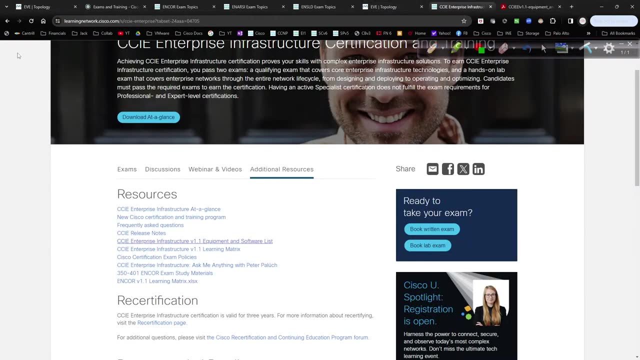 So that's really the driver for that. So we're looking at this topology. how do I come up with an addressing scheme for a lab that I'm working on? That's just something I also get a lot of questions on, And so the simple answer to that is because of the fact that the EI blueprint- if we go, 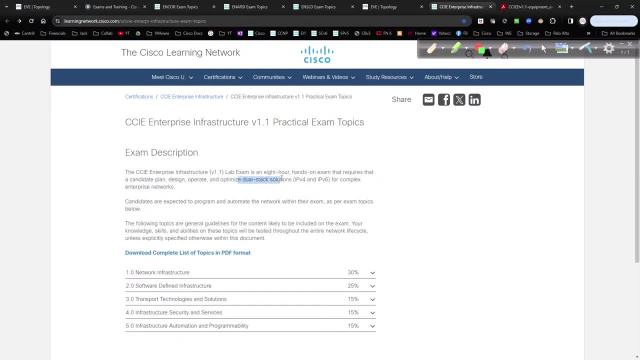 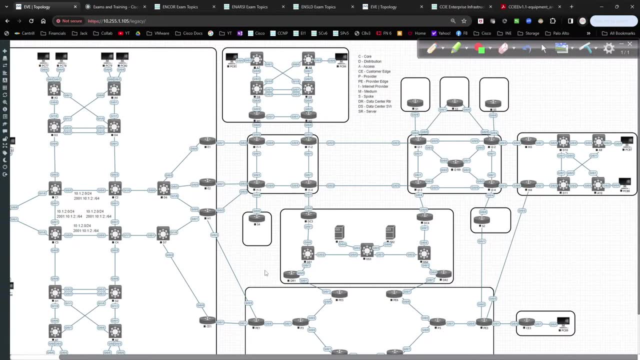 back one here, Okay Okay. So I'm going to go back to stack solutions V4 and V6.. So because of that I automatically look at doing IPV4 and IPV6 addressing schemes. So what I ended up doing is I go through and I text box here and then I break it out. so 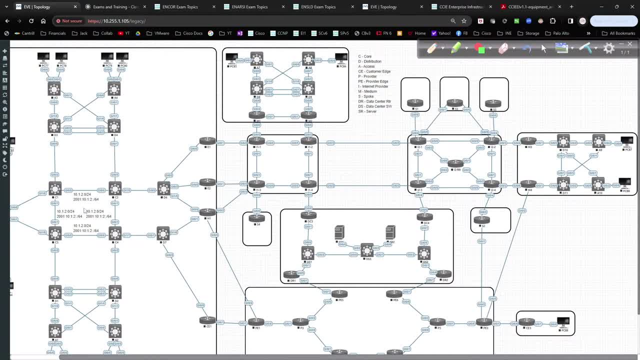 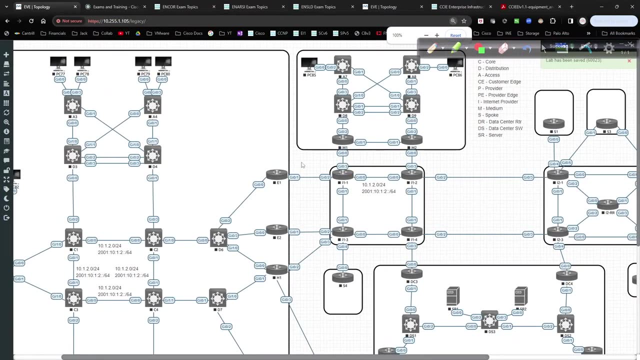 that I have a IPV4 and an IPV6 address on a per link basis And then I do that everywhere. So I'll give you an example If I duplicate this guy here And bring this over here. So one of the things, and I'll go ahead and zoom in just so that it's easier for you guys. 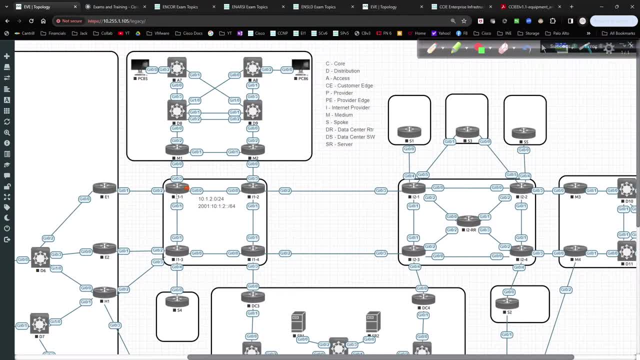 to see that are at home is: I did ISP1 and I've got routers 1,, 2,, 3, and 4, and I've got ISP2 routers 1,, 2,, 3,, 4, and then I have a route reflector, because the blueprint specifically 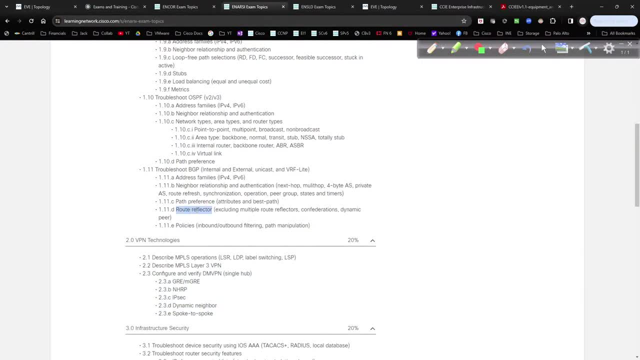 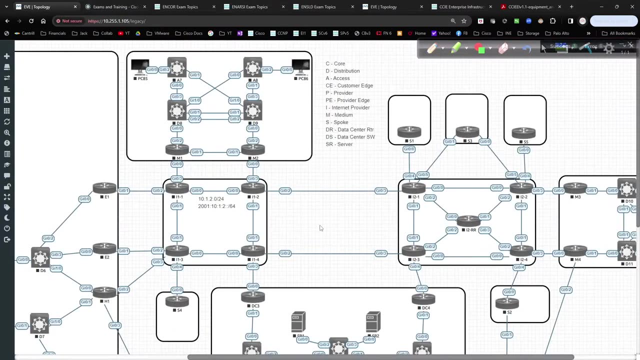 for an RC for BGP calls out a route reflector design. So I was using this exam breakdown to be Right To be able to use for how the topology was built, And so what I would do is I'd click inside of here and I would eliminate the zero and 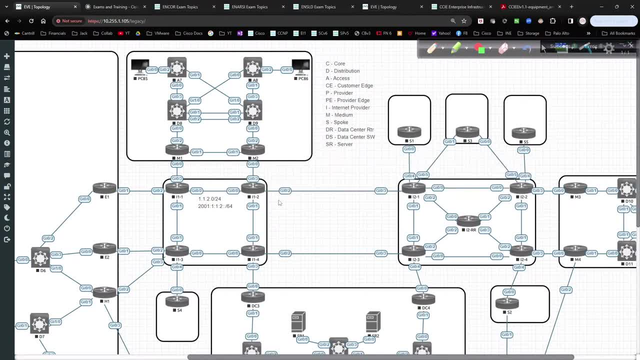 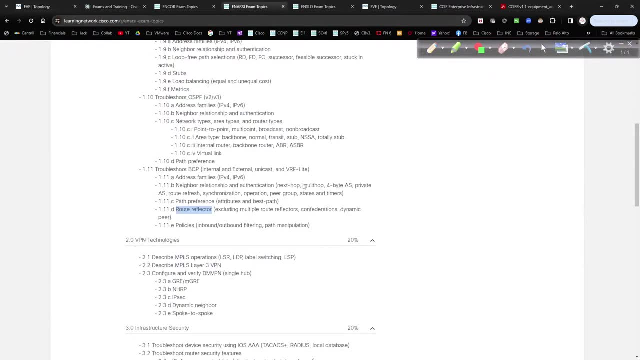 I would have something like this, So that would be my addressing structure as I'm going around, So I'd use public IP addressing anywhere in the lab that I could. Now there was a. Somebody left a comment about using AAA to do because in the NRC exam it does talk about. 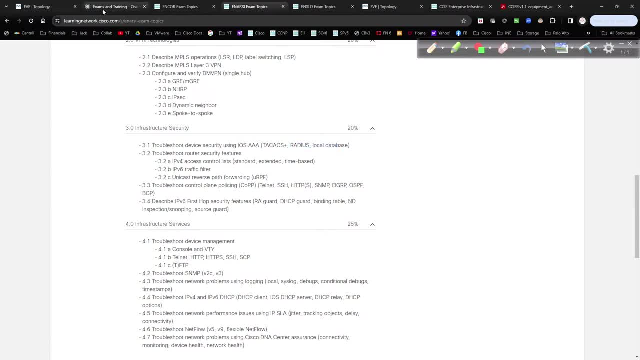 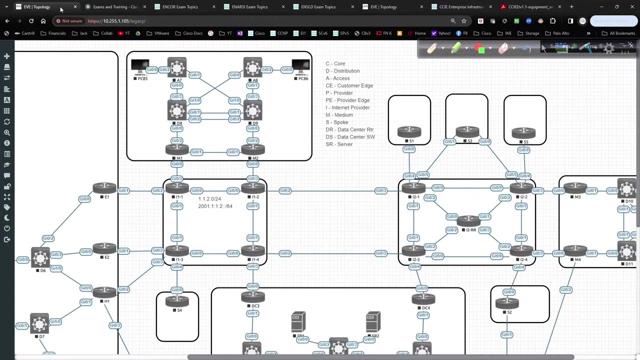 AAA, It's a TACX radius local database and it's a great idea. I do have an ICE VM that I could deploy in my ESXi host and go through that, So I don't see a reason why we wouldn't be able to do that. 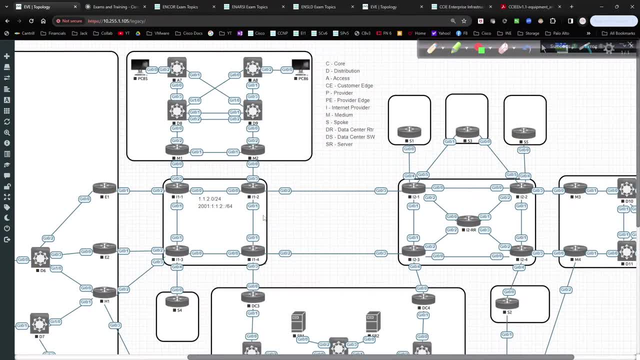 So I more than likely will be able to do that and use that for doing that type of stuff. It'll. I'll use the- What do you call it? The workbook to figure out how to do all that stuff, So the video series that follows it'll be that much easier to work with. 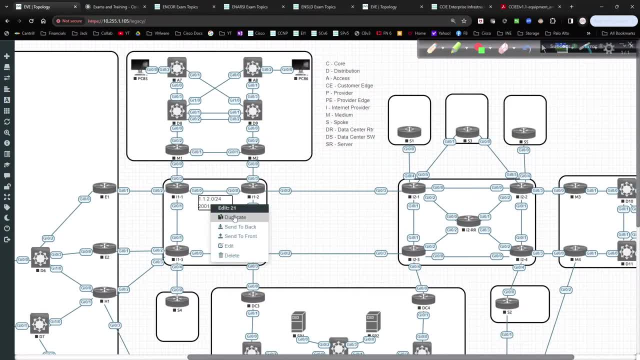 The videos will flow much nicer. So what I would do here with the duplication is I would just mimic this on all these links so that we have the setup like that. So it's a little tedious and time consuming to do it like this, but what it gives me is 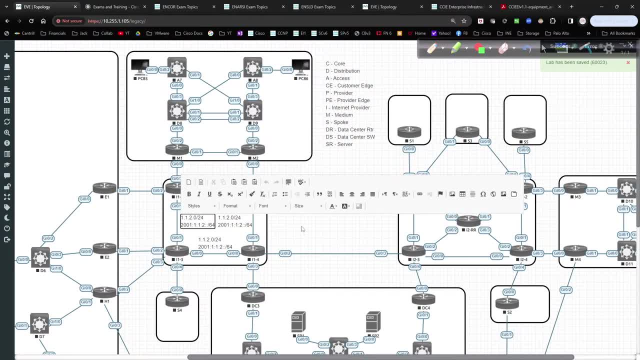 it's an easy to follow along format. So I'd come in here and this is going to be 1.3 and like so, And then, once I have the addressing scheme broken down, it would be in your example. would it be easier to break your addressing by region, country, site, branch depending? 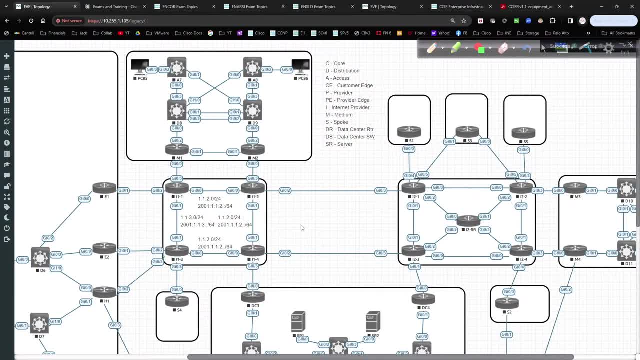 on company size: ie America's get a slash 12, Asia gets a slash 16. Then further break down further for DCs. Yeah, Mario, that's pretty much exactly what you would do on a global scale, is you would? 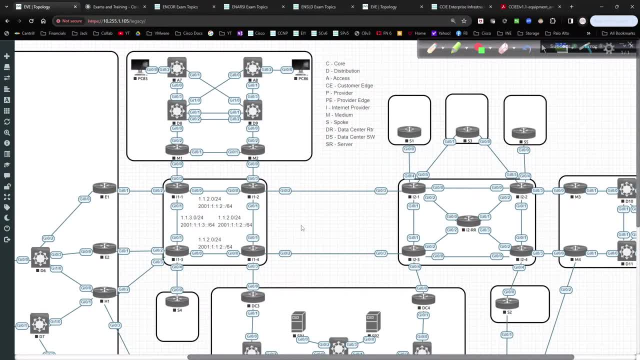 break it out like that: You would give huge chunks to where they need to be, and then it would be up to the admins or engineers at those specific geographic locations to further break down what they've been given access to, So that, by the time you're said and done, you've got a global architecture that makes 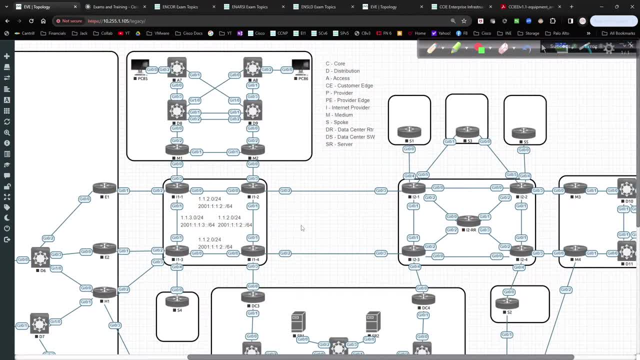 sense, If you have an IP address or you're trying to trace route through something and you have a high level overview, understanding of how the addressing scheme works for your environment, then you'll know where something's heading to or coming from. So yeah, that's exactly what I would end up doing. 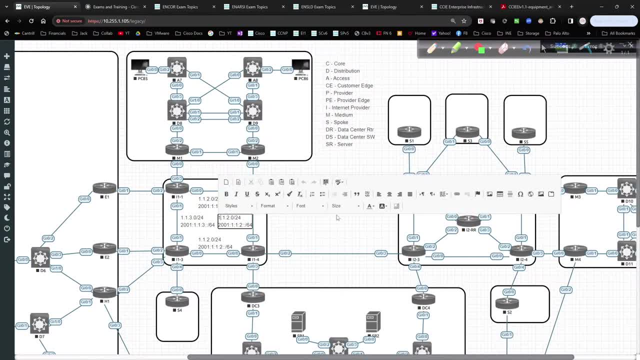 So when we look at this, it is a little time consuming, but by the time I'm done and I get all this laid out, the cool thing about it is that once that's done and I have it, it's done Yeah. 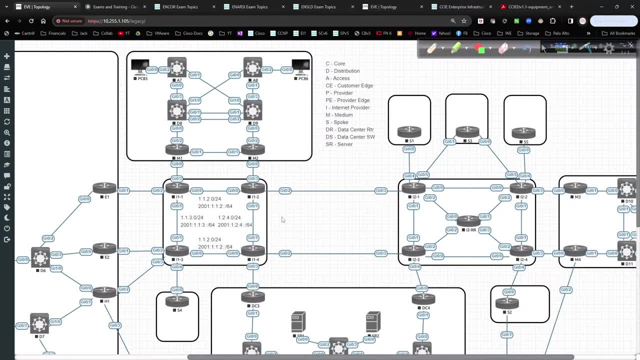 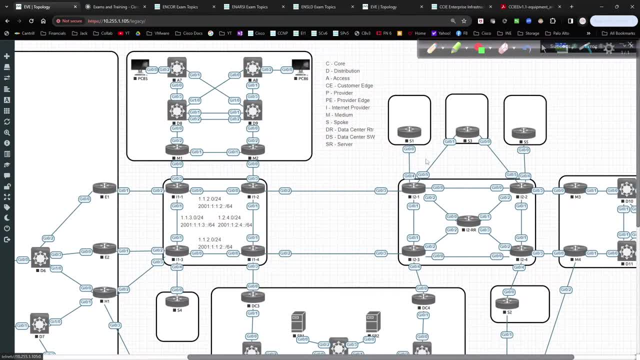 trace route, for example, from, say, edge one out to spoke one, I follow a particular path. or if I'm natting on E1 and traffic comes in on E1 and goes where it's got to go for internet reachability testing and things like that, then the capability becomes evident. 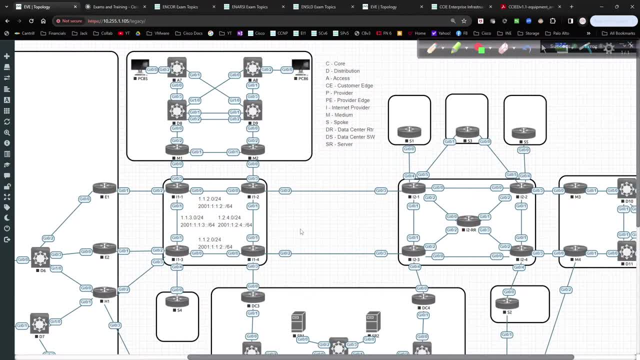 where the traffic is flowing. So that's essentially what I would end up doing Now. funny enough- I don't know if the video Nope, the video is still goofy. Funny enough when I built out- I'm not sure if it's on this one here- 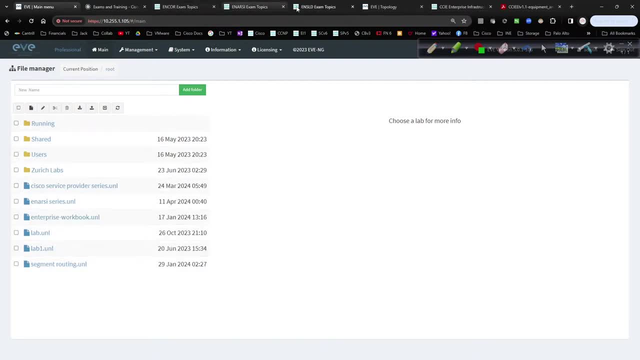 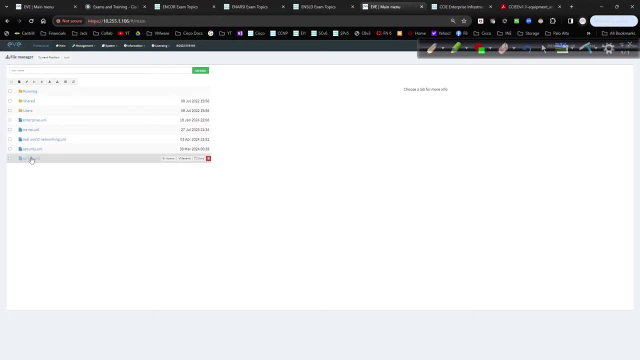 No, It is not. It's on this guy. I have a lot of labs that I've been working on Nope. you know what My mistake? I accidentally deleted it. Or I didn't say accidentally, I deleted it because it was improperly built. 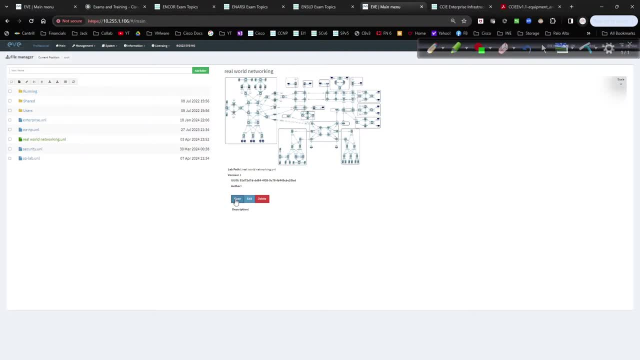 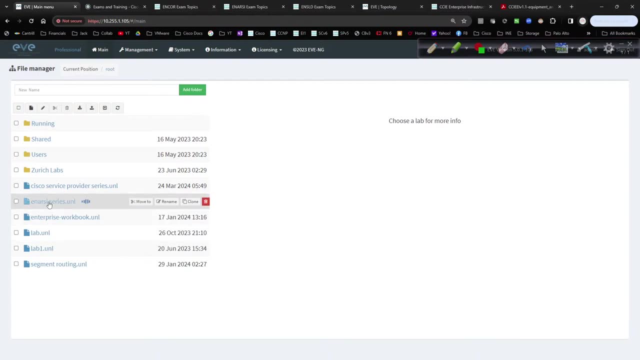 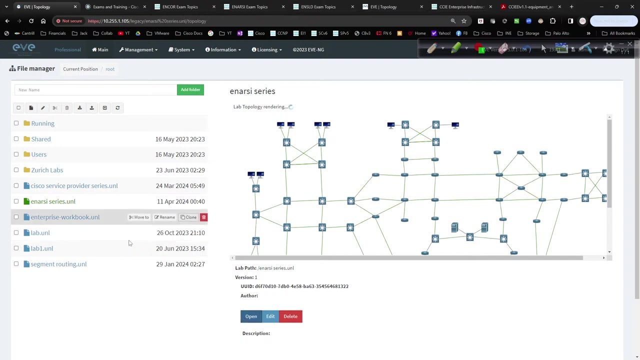 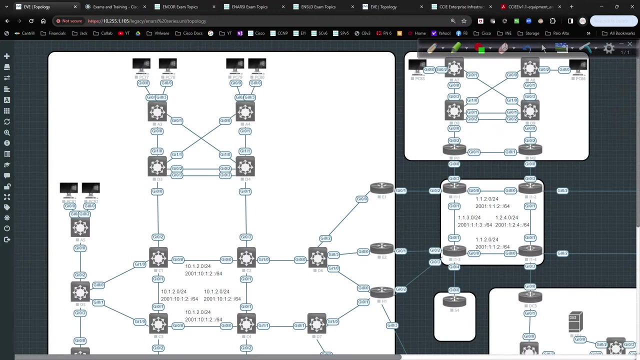 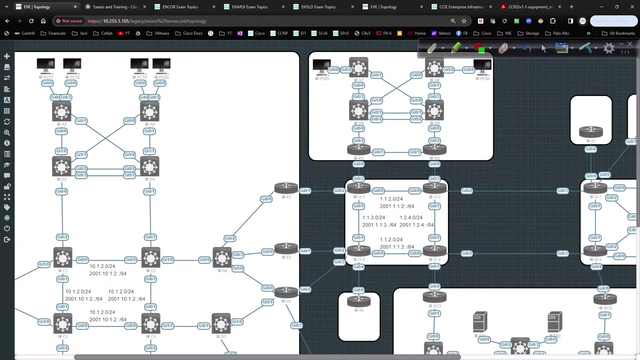 So I was just going to go ahead and rebuild it. So I built a topology that. Let me go back into NRC. So I built a topology for the service provider series that I was working on And when I, When I was working through that, I intentionally built it wrong in a couple of ways as a way to highlight the correct way to go about doing design and your routing architecture for BGP. 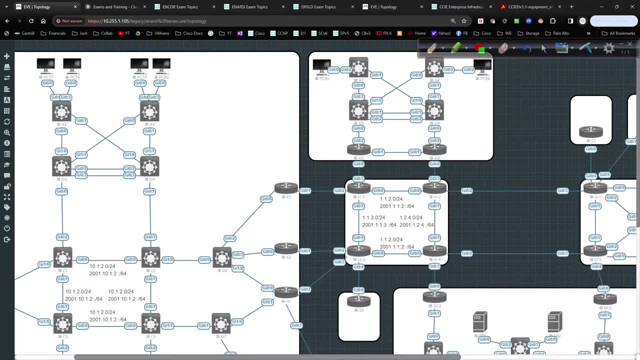 And I got about partway through and I was like: man, this is The intention, was there right To do things the right way, and things like that. But then I got to a certain point where I just was like: eh, 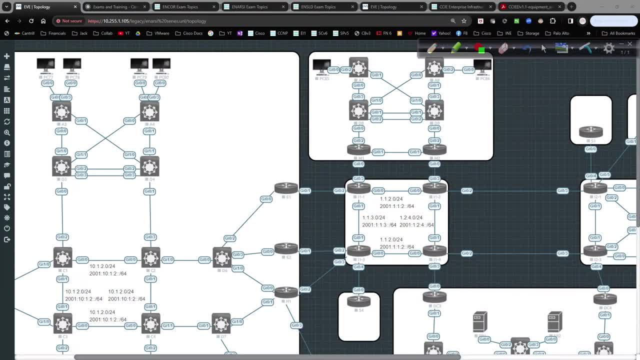 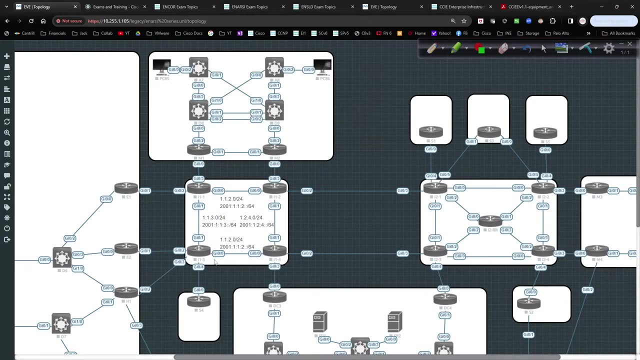 This is becoming more. It felt like I was leading you guys the wrong direction, Meaning that if, for example, I was trying to get traffic to go a particular direction and when it wasn't working the way I intended it to, and then there was RFC 1918 address space on the public internet, I'm like um, you know if I'm 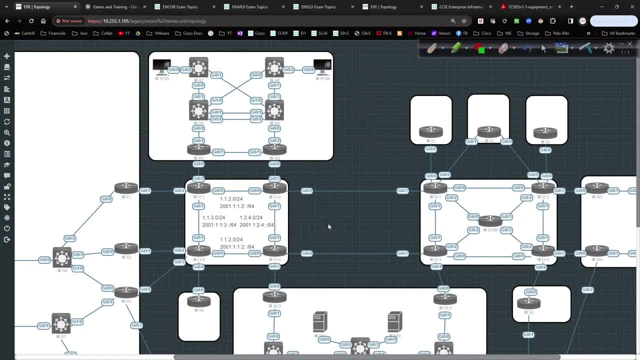 If I'm a CCNA and I'm working my way towards Towards CCNP, and I know that you can't use RFC 1918 address space on the public internet, but yet I see a workbook that's written by a CCIE who should know better. 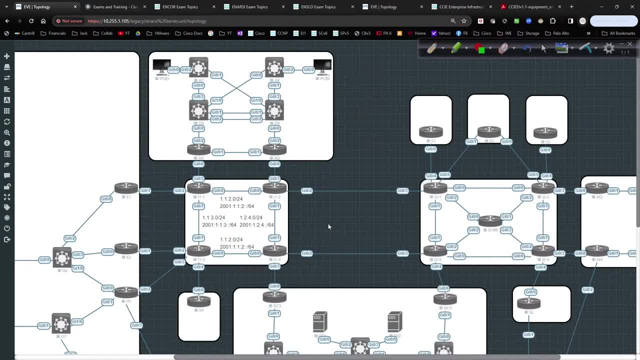 and I see that this configuration is done incorrectly and I see RFC 1918 address space on the public internet. What gives This guy should know better. So I was rethinking the end goal of the workbook And so I decided to reassess that, and so I'm working through those details. 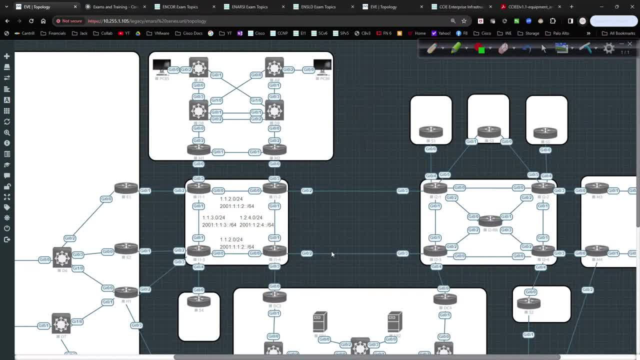 But it's one of those things where, if you're going to be doing anything with technical training, you should be doing it in a manner that's going to benefit the end user and not put them in a position where they're like, oh, this isn't working. 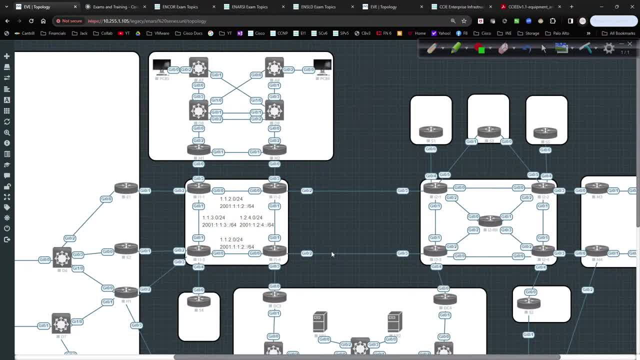 But then there's a you know two or three page- I'm sorry, two or three paragraph breakdown, And so why it won't work and then how to fix it. But if you're taught how to do it right the first time, 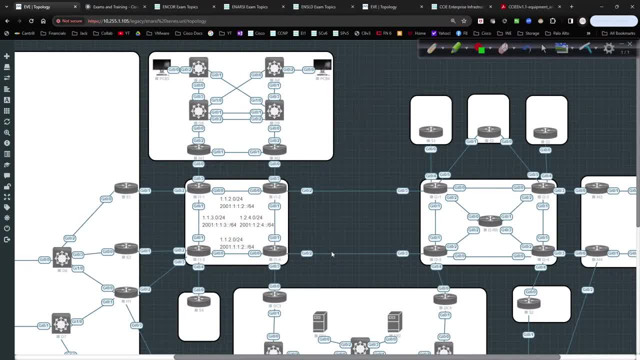 you won't make that mistake the first time, At least that's the intention. Hopefully that makes sense. But so the I'll go ahead. Since I'm literally right here, I might as well just do this one here, But this is the. 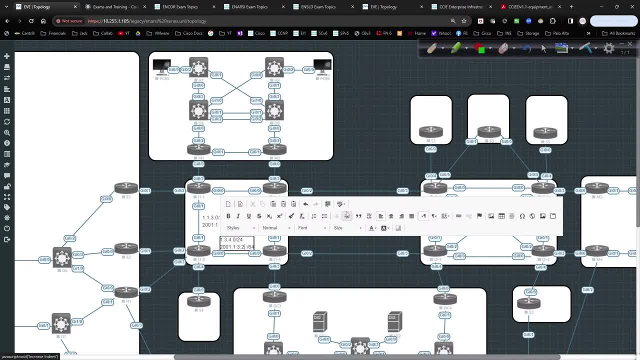 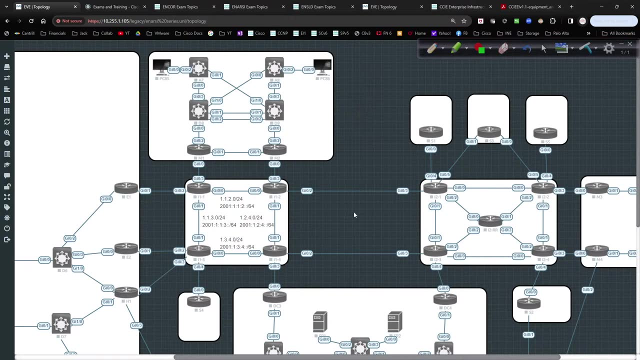 Oops. The goal with this is having it very evident where the traffic is flowing, based off the IP address. I'll sit here for a little while, I'll do a bunch of copies to wherever they've got to go, And then I will use that when I go to configure all the devices. 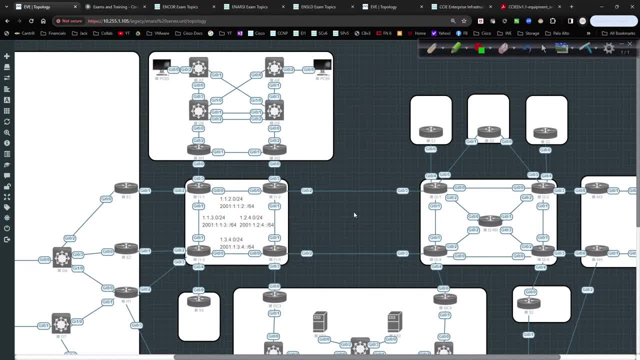 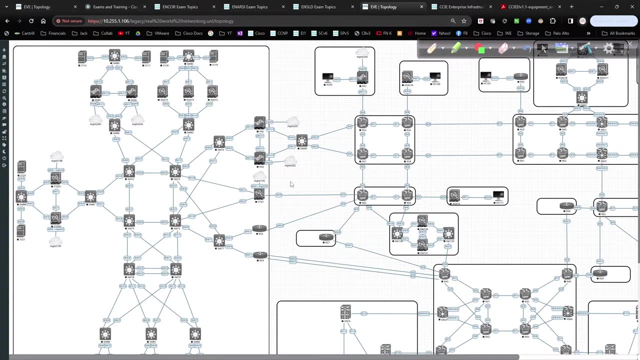 So it's multiple rounds to get where I need it to be. Now, going back to Musab's comment about SD-WAN, that is probably something that I will do in the real world networking topology, Now that you've brought it up. I hadn't thought about doing. 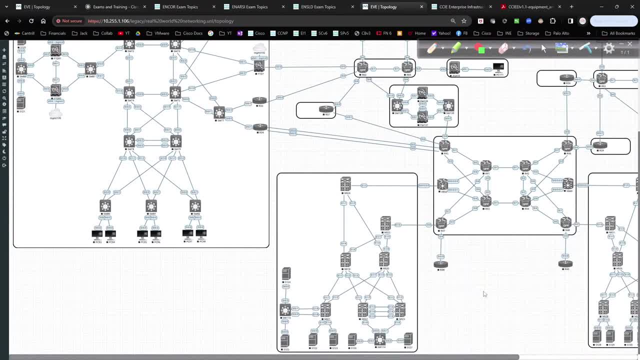 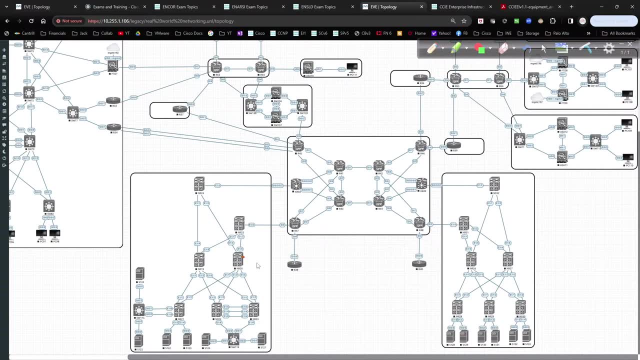 SD-WAN, but now that you bring it up it probably wouldn't be such a bad idea. I went so far as to do a large-scale VXLAN deployment where I'll have multiple 9Ks border switches or border devices. 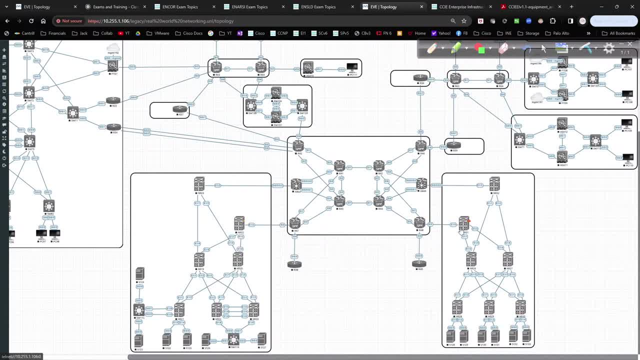 Well, this would actually be a border gateway where we'll have a layer 2 VPN configured in the service provider so that I can have connectivity between them and do stretch VLANs and things like that, because I've done a lot of VXLAN multisites. 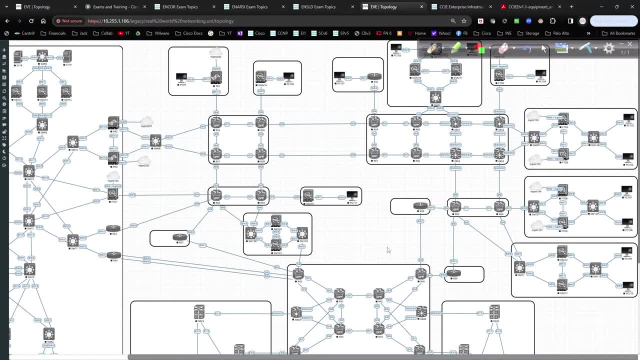 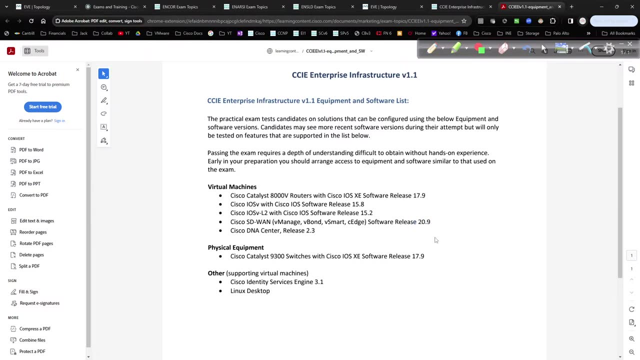 I've done a lot of VXLAN multisites with a lot of customers, So I could probably take the real-world networking and I can probably expand upon it. but I would need to get the appropriate version of code for SD-WAN and then we'd have to go through and stand up all of that. 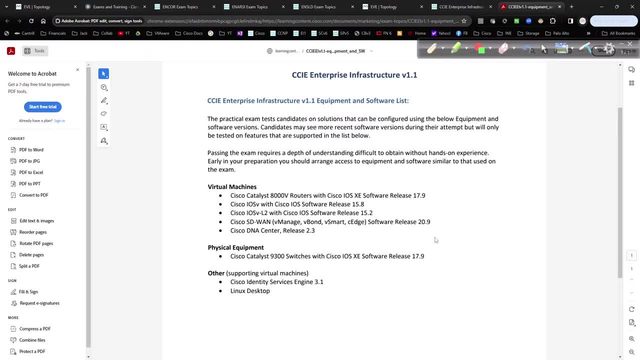 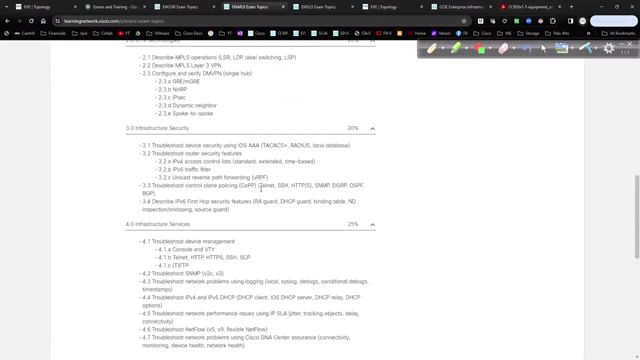 How are you coming up with topologies? Are you thinking about it for a few days and then putting it on paper? To a certain extent, yes, You can't see the whiteboard that is behind the camera, but a lot of it comes down to when I'm looking at the exam blueprint. 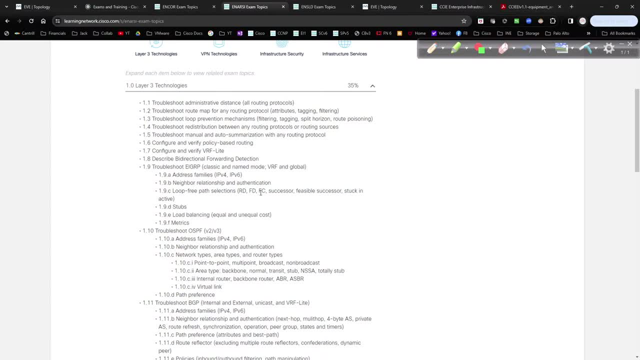 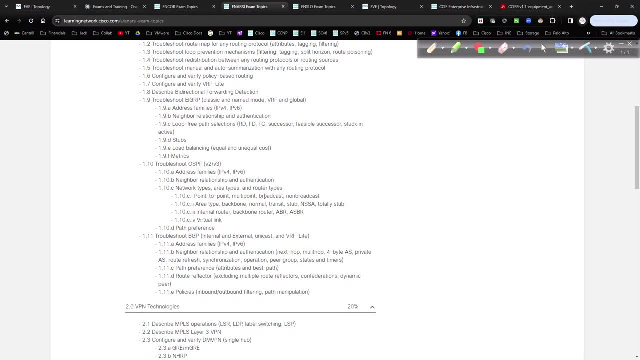 I can visualize what this stuff would look like. It's not very difficult to come up with a general idea and put together a topology that would be large enough for it to make sense in the respects that it needs to be done in. So that's essentially what I ended up doing. 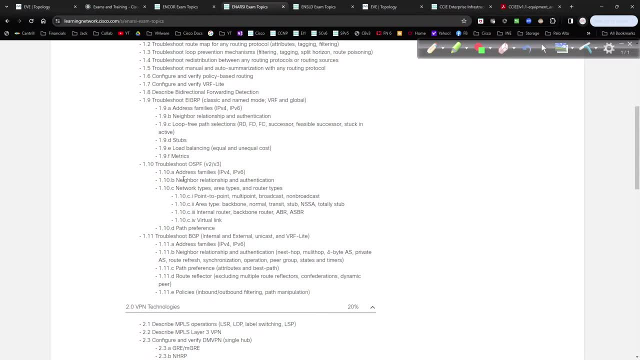 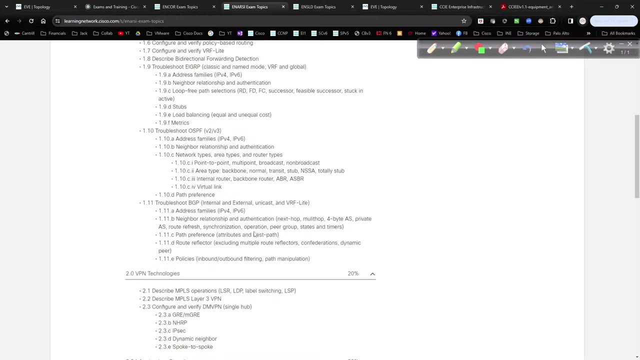 As I take the blueprint. so it says virtual links. how would I be able to do that and make it easy for whoever's following along to be able to do it? So that's essentially what I do. So I just take the exam blueprint and I'm like 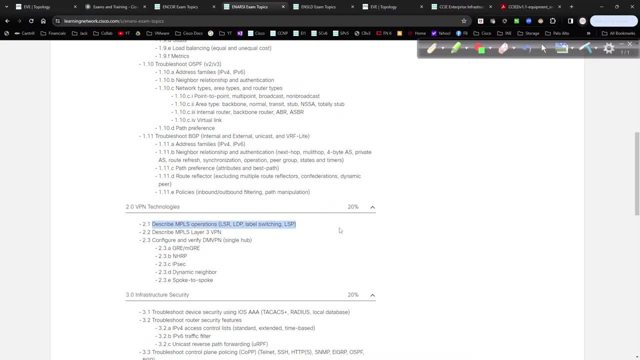 okay, if I've got MPLS, I know I need to build out a Layer 3 VPN, So I'm going to need an MPLS core provider edge routers connectivity to a customer edge. I'm going to do more likely BGP with that. 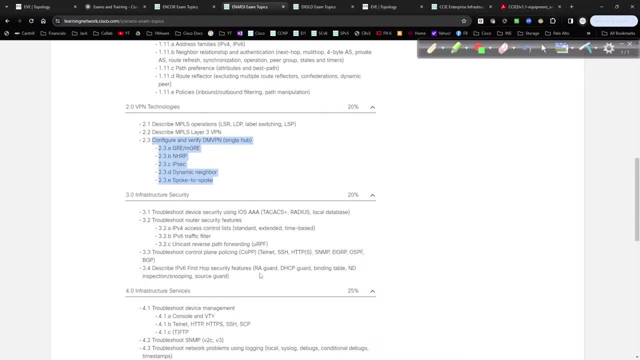 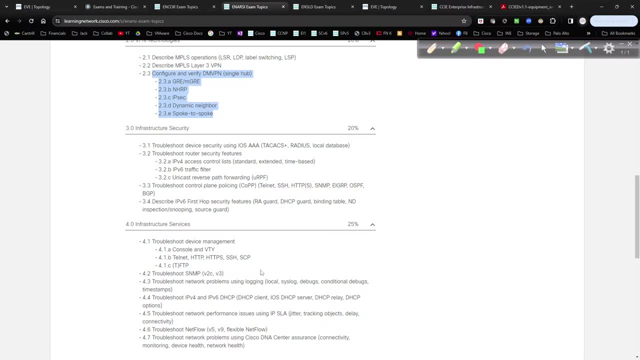 I'm going to do a DMVP and single hub and stuff like that. So a lot of it just comes down to knowing how to configure that stuff already, what the architecture looks like and being able to take what I already know about it and then basically building something out like this: 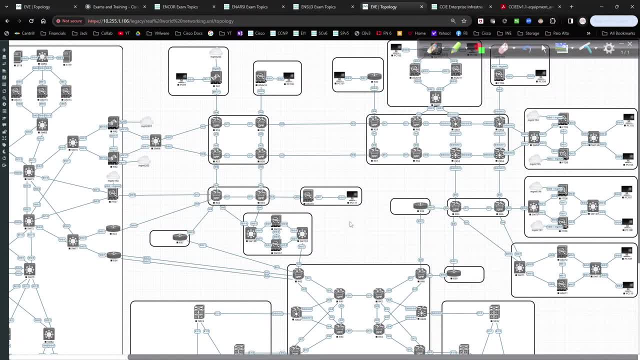 Is it big and kind of just ridiculous It is, And I don't necessarily put it on paper per se, but I will take. I'll take the exam blueprint over to my whiteboard and I'll draw something out Like: okay, how would I do this? 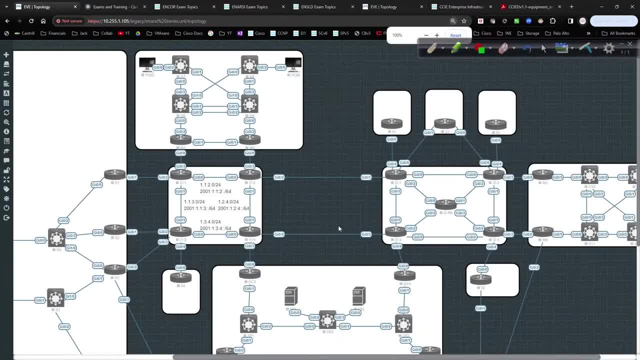 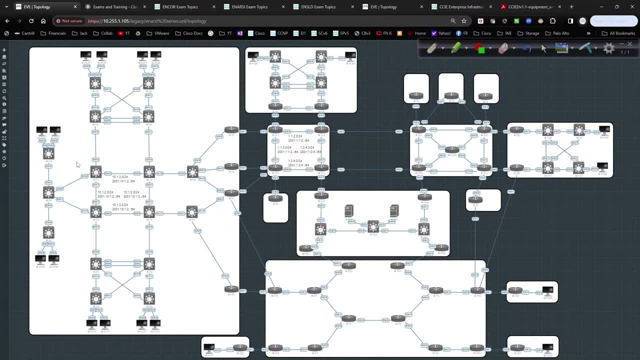 And that's where stuff like this topology here for an RC is kind of built from. It gives us a lot of flexibility. We have an HQ site here with a big OSPF deployment. We have a couple of smaller sites with EIGRP. 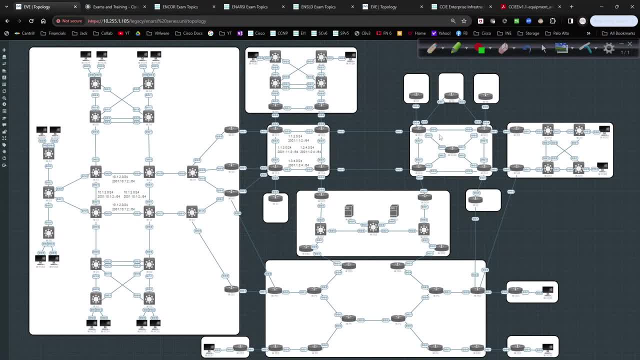 We have some spoke sites for DMVPN, We have a couple of big, some internet routing for doing BGP and path selection, and then we have a colo, because i can't tell you just about every customer that i work with has some sort of cloud presence, whether it's using software as a service like office 365. 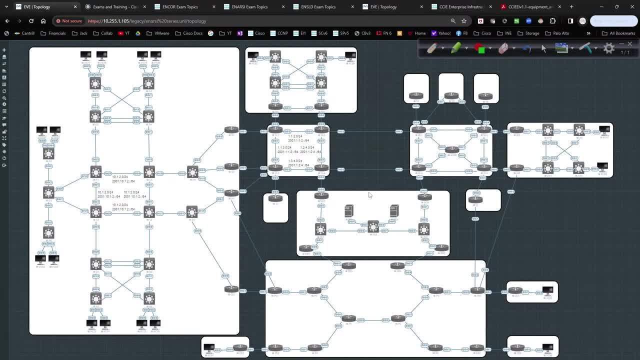 or google, um, google the g suite, or take your pick right. there's all kinds of cloud initiatives out there, and so i take the knowledge that i have from that and i'm able to just like mimic a lot of this stuff. i mean, is it getting down to the point where we need to go through, and do you know? 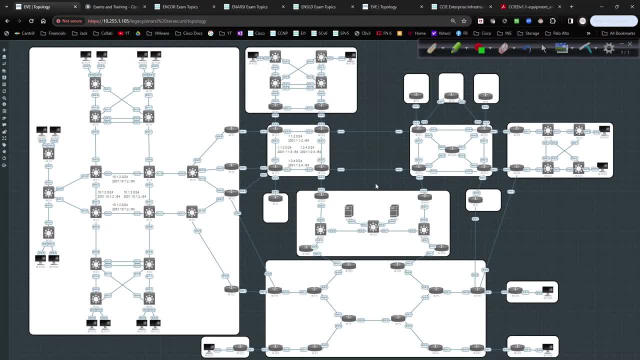 i'm not trying to like rebuild or recreate, to like make it look like aws, but what i am making it do is, uh, what it was like the, the mechanics of it. so if you're going to be connecting to a colo, you're more than likely, or going to aws or azure, you're more than. 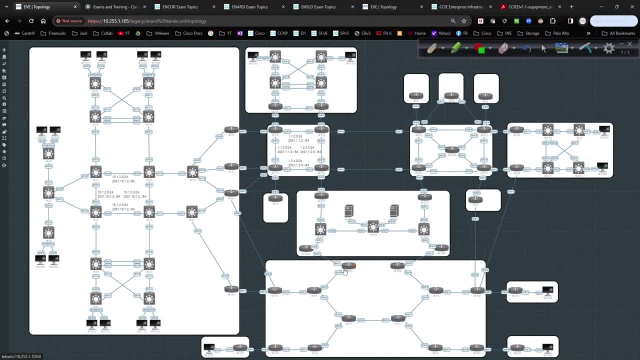 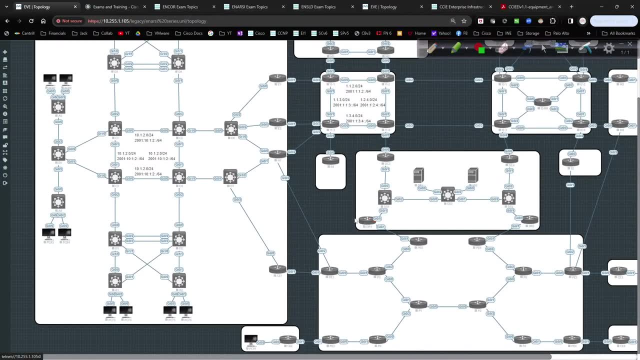 likely going to be standing up a bgb peering with them. so we're going to do the exact same thing. we're going to configure pe5 to form a p appearing with data center router one and go ahead and turn the turn that light off. uh, get that peering stood up um. 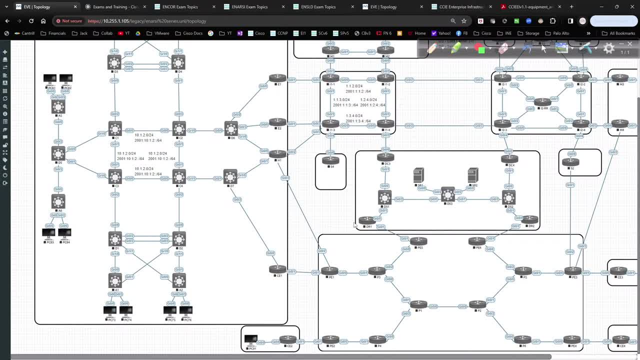 oh, youtube live has ads. oh, i did not know that. uh, i will have to fix that, my mistake. uh, edit, can i edit the monetization save? okay, i just turned, turned it down on the youtube ads. hopefully that'll be easier for you guys. so, um is nothing much. so i hope you enjoyed that video and i will talk to you guys next week. bye. 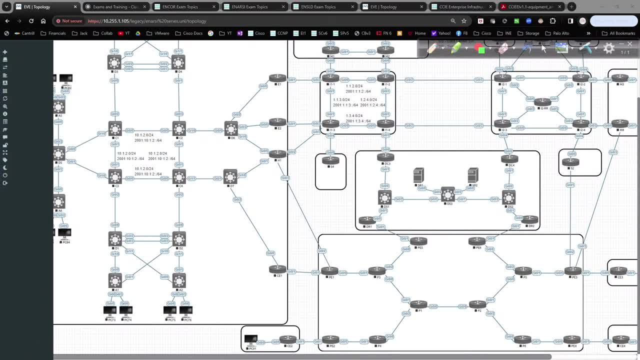 bye. Um, actually you know what. I'll turn it off. Monetization off. Done All right. So I just turned the monetization off on the live stream and I'll turn it back on once the it's in been recorded. Yeah, I can turn monetization on or off on the. I just didn't know it played ads during. 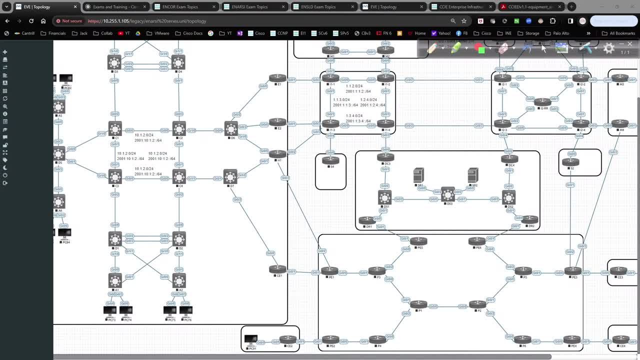 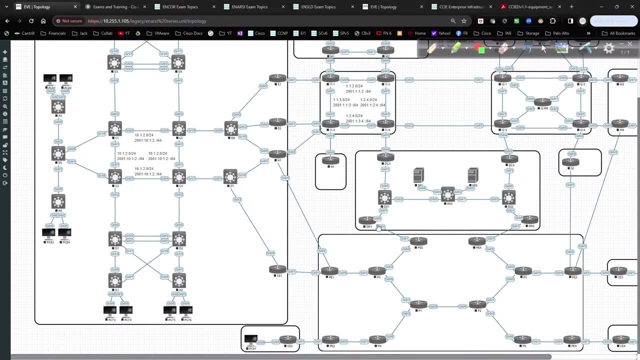 the live stream that I don't like that. I'm going to turn that off. So I turned it off on this one here. So, um, that's where this really comes into play, And then the addressing structure that goes along with that. we'll figure out something from that in that, uh, in that perspective. So 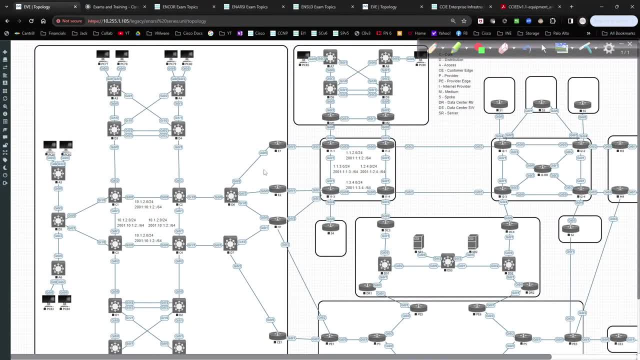 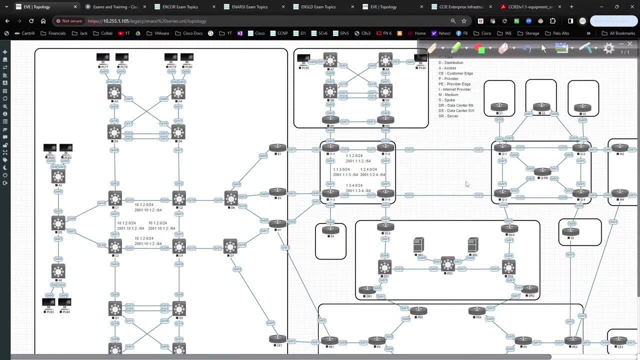 the um. so the edge here, edge one, edge two, this would be, uh, internet edge redundancy, right? So we'll have multiple ways of getting out to the internet and all that good stuff that goes along with that. Um, uh, this is still a work in progress, but I have a high level overview of what 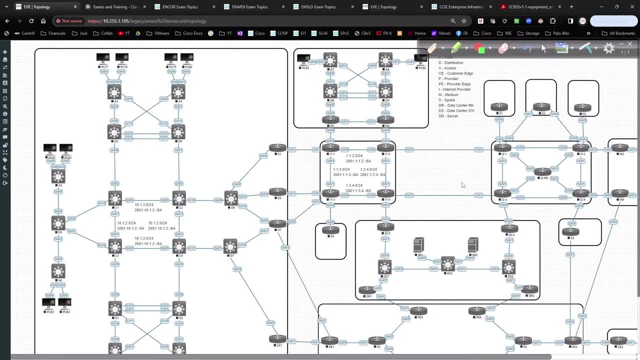 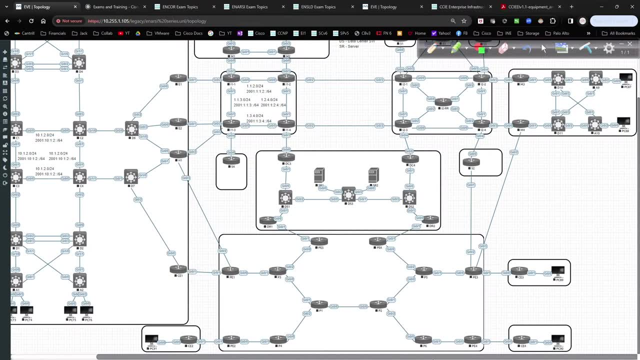 I know I want to uh, to go through and break down, But that's where you know, as the further you get into the networking world- and I know, Irfan, you've been doing it for a while too- Uh, you and I have known. 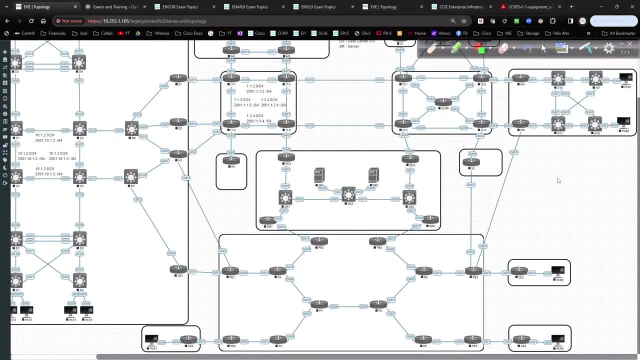 each other for a while. Um, we're, yeah, as long as you've gone down the deep dive of how the technology works and things like that, um, it's not very difficult to kind of visualize what it is that you're trying to accomplish and how you're going to get it there. So 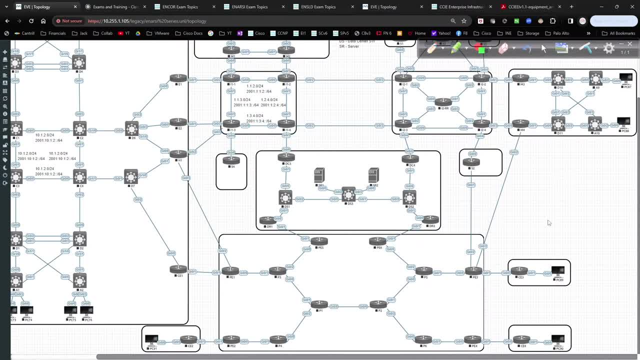 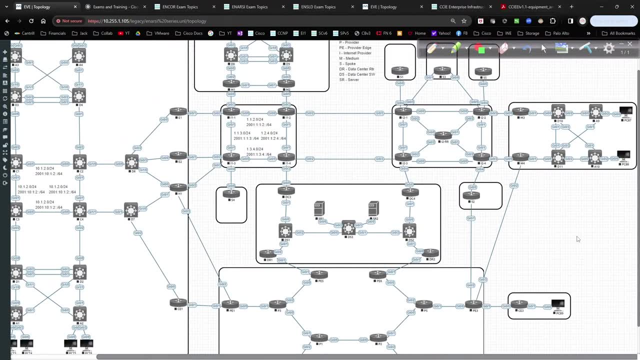 you know it's just one of those things where there's some trial and error and you figure it out as you go And you know, sometimes it makes a lot of sense. Some of the times you're just like you're scratching your head trying to make it make sense, if you know what I mean. 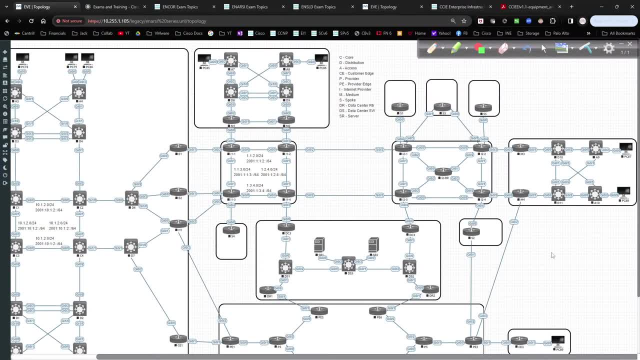 So, um, that's pretty much where that comes into play. So it's a lot of- uh, you know, trying to make the training as real world as you can, because at the end of the day, you know, most of the, if you go to a, a traditional training provider, you know, insert whatever. 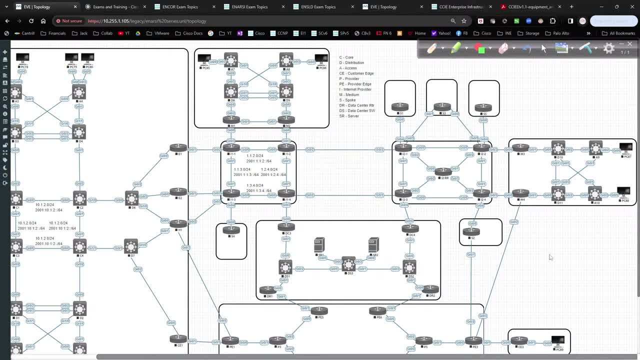 name you want. they're going to have certification based training, right It's going to. their goal is to help you pass your CCNA or your CCNP or your VCP or whatever, And that's all well and great. but you've the moment you get outside of your cushy little certification learning environment. 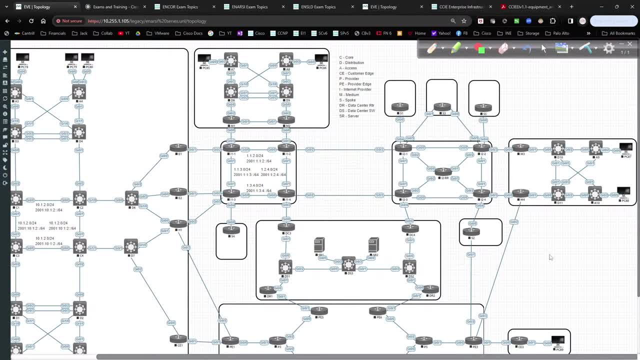 where you're not afraid to break anything. you can break the network and all that type of stuff. The moment you disconnect from that and then you go back into a production network. you're back in now, you're back in the wild, And this is where I feel like if you spend more time, 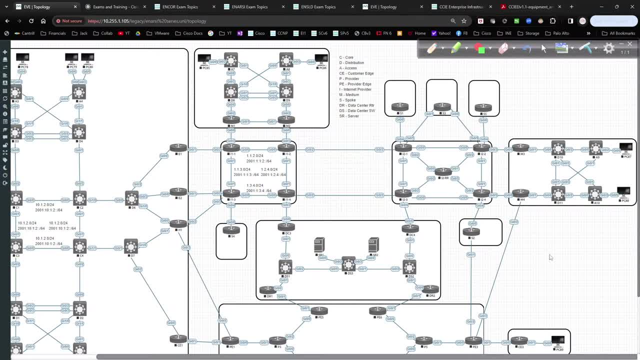 in a lab intentionally trying to figure out how to make something work, and you're putting the time and effort into it. this is the type of stuff where I think really makes you the better, better engineer you know, and there's- uh, there's something to be said for somebody that 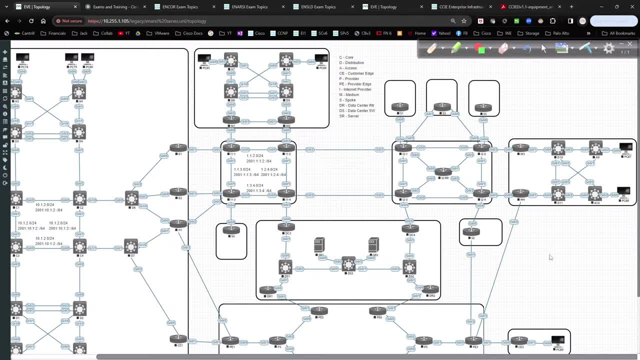 spent a lot of time labbing Stuff up and making sure that it's going to work out. You know, it's one of those things where I got a lot more credibility out of from my customers that knew that I had spent hours putting together a lab to make sure that everything was going to go swimmingly. So 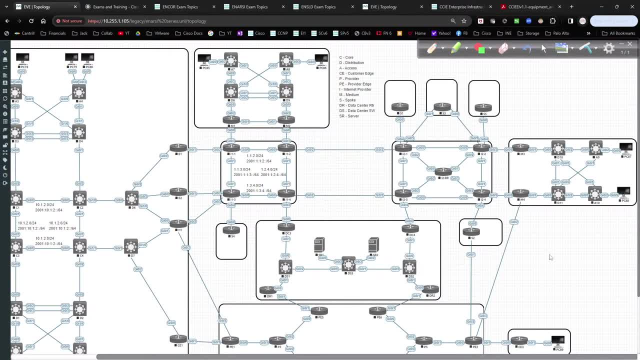 that by the time that the design was put together, the configurations were all laid out and all that type of stuff, that the, the change window and the migration or the deployment was just a formality, right, You're, you know, it's more like you know, uh, um, yeah, it's, you know how. 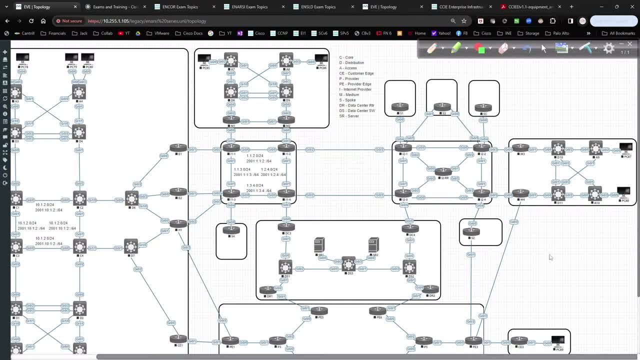 it goes, though. It's one of those things where you spend a lot of time digging into the technology, but the moment you get out of your cushy little certification world, you uh, and you get back in the real world. uh, that's when you tend to overthink and double check everything, because 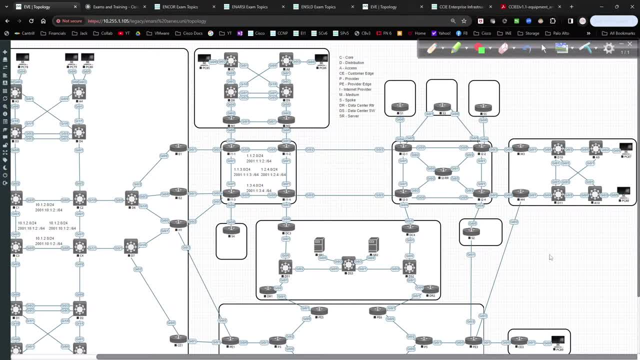 you don't want to break anything. You don't want to be the reason why you're not going to be the reason why the network went down. So, but if you put the time, the the correct amount of time in and you've got all those things figured out, um, I always felt way more comfortable doing it that. 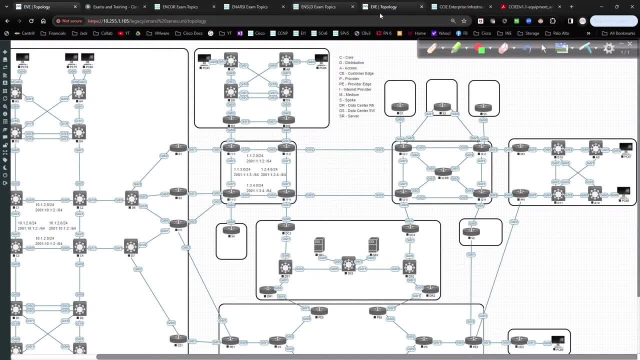 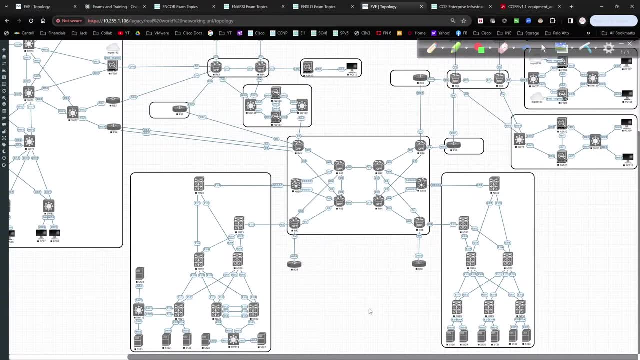 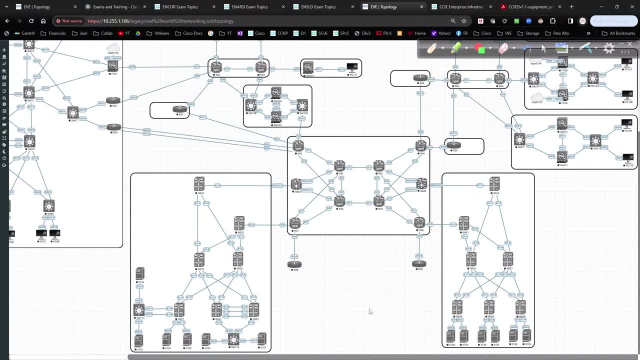 stuff that I had to work on every day. So I was the one that took and built out. sir, I took servers, deployed Eve to them and roll, basically built out customer environments on the servers So that by the time we got to that point there was no guesswork. 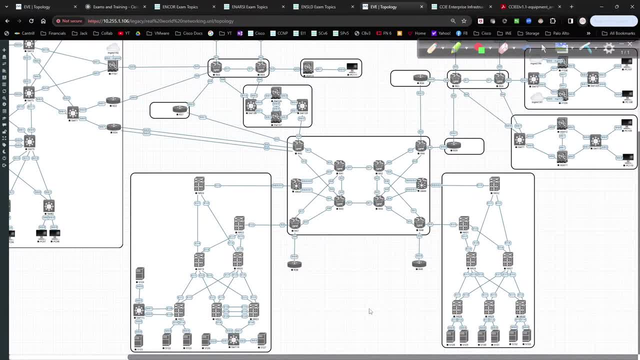 Like I knew for sure I could pull it, I could pull up the topology and I could have the CLI in front of me and I could break down: okay, this is how it's going to work. And unequivocally, and have the confidence that you know, the customer basically relied on me to provide. 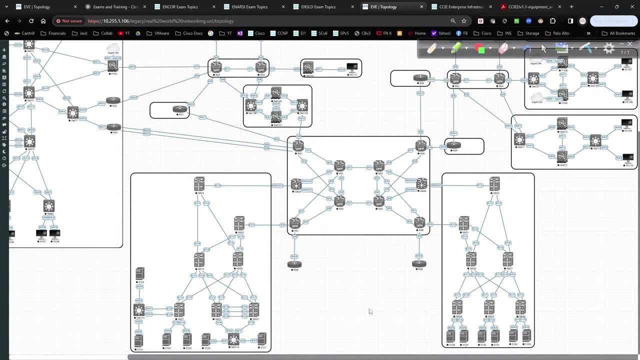 And that's one of the things that I think gave us a lot of credibility was I was putting that time and effort in and the documentation that was produced from that I was able to give to the customer and then they were able to take that to their leadership and things worked. 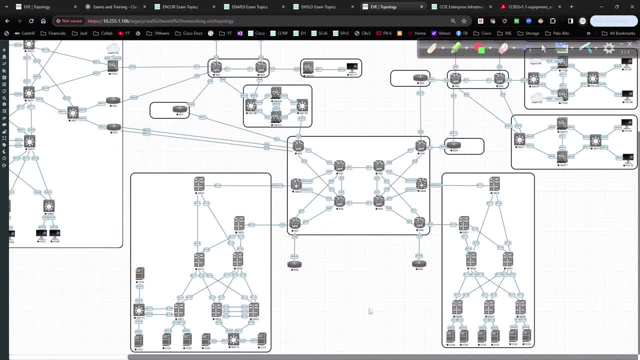 You know, we didn't have to sit there and to guess at the end of the night. So you know, and if something didn't work, it was either A- we hit a bug- or B- there was something about what we were doing that I just wasn't aware of. 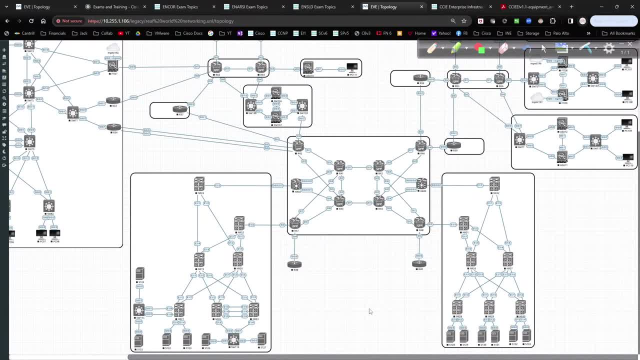 And is it possible? Yeah, stuff happens. But I'd say, out of the one customer I'm thinking about, we did probably a good 30 or 40 projects, different efforts, And then eventually I got to the point where I was like 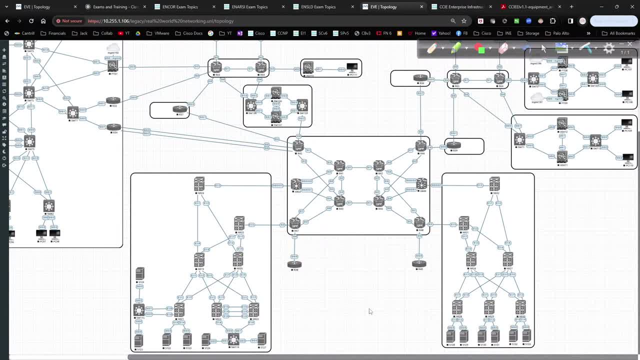 we ran into one or two issues but I was like, wow, like you learned something from the corner case stuff. Rob, do you recommend working for a VAR early in one's career to gain the most exposure versus working in an enterprise? That's a good question, man. 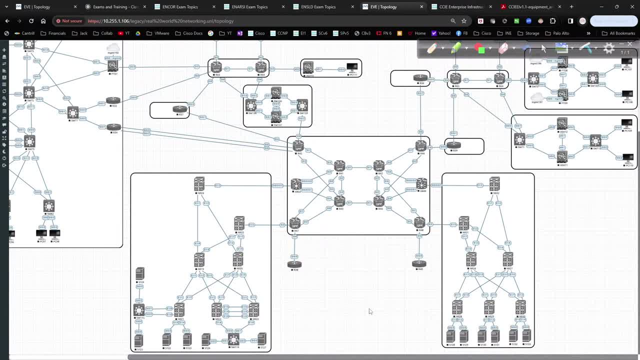 I honestly would say it makes more sense to me to work for a VAR. For those of you that don't know that's a value added reseller. I would more or less recommend working for a VAR, And I wonder if the video is any better. 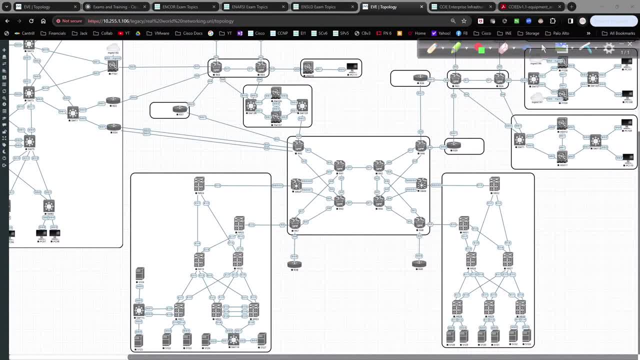 No, it's still jumpy. I would recommend working for a VAR because especially if- at least for me- I don't like the slow moving train, The glacier style moves that some big organizations make. they just take forever to get from point A to point B. 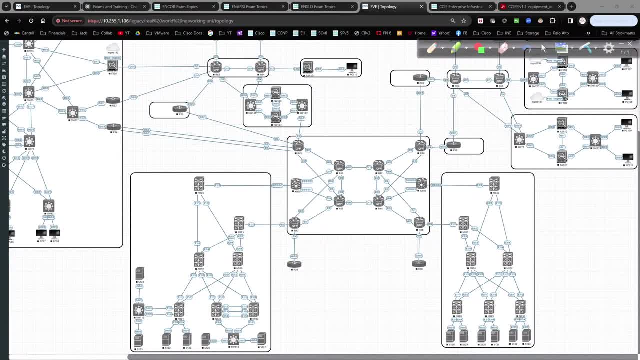 I like to be a mover and shaker, I like getting stuff done And I like a little bit more fast paced. you know where you're fast, You're forced to do your challenge and things like that. But that's one of those things is, you know, it's not for everybody. 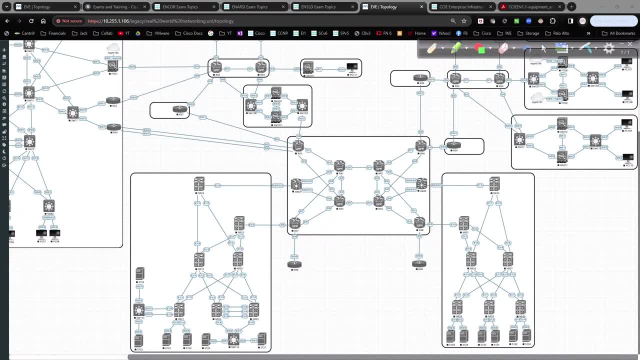 I've seen some people just literally just fall apart when they're presented with a problem and it seems to be untenable for them. So I tend to take in the content, understand it, lab it, document it, But I'll never sit the. 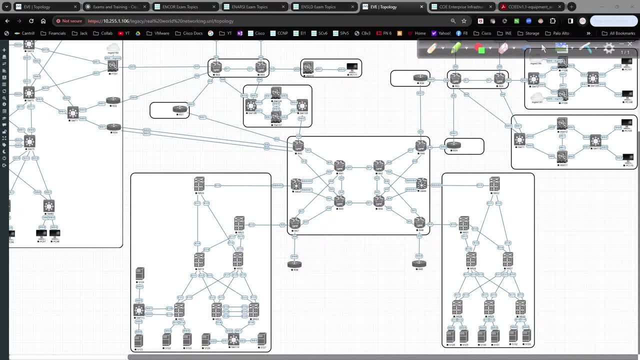 Exam, not a great test taker. Knowing the why is huge. I agree with you on that one. I think it is definitely something that, if you are, So, My bet, my advice to you, Mario, is this: If you have done all of the work up to the point of actually taking the test, 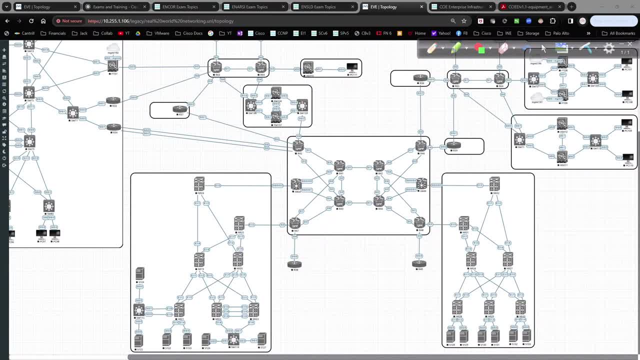 I'm the same way And I will take the test, because I don't know if you ever used or heard the term circle in the drain on something. but you spend all the time and effort to learn something. you want to have something to show for it, right? 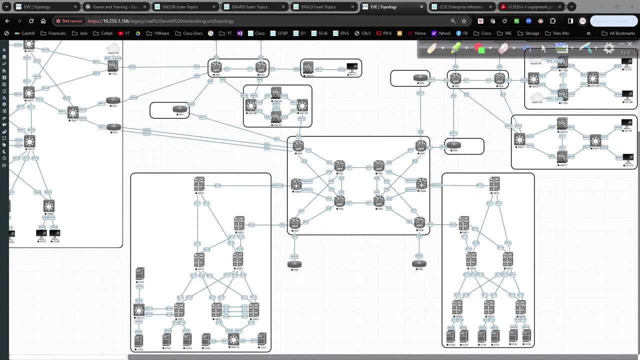 That's what I would do. So like I'm, I know, in the near future, when it comes to taking the service provider CCIE, taking the CCD, practical stuff like that- that I'm going to have to bite the bullet, I'm going to have to spend twenty five hundred dollars and go take the test. 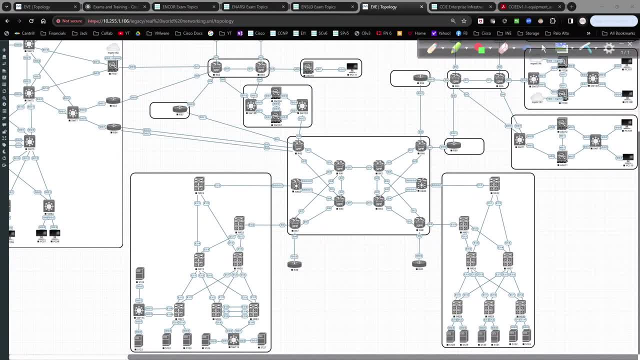 And there's really no practice test for CCIE, So you're kind of you do your best to learn all the material you can to your point, taking the content, understand it, lab it, document it and all the good stuff that goes along with that. 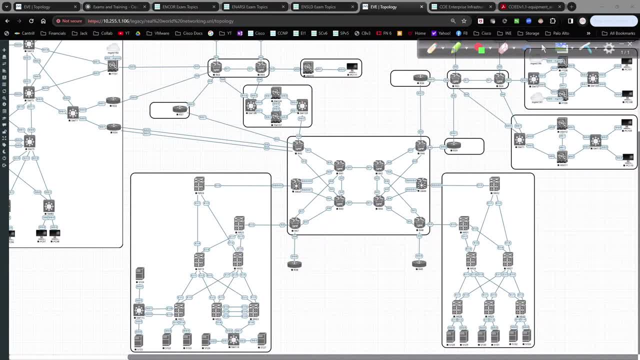 But you get to a certain point where you just have to bite the bullet and take the test- And I am not a great test taker either, Like I'll, I'll drink to that, Um, but you just have to, you know, bite the bullet. 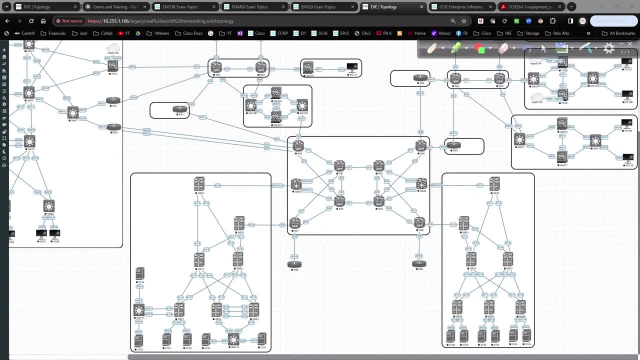 That's like the. that's what I tell people. So At some point can you talk about some real world scenario about migration from IPv4 to IPv6, both from a design perspective and technical, just for curiosity's sake? Yeah, actually that's one of the things that I like about the community that I've built here is that there's something you would like to see in the real world scenarios piece. 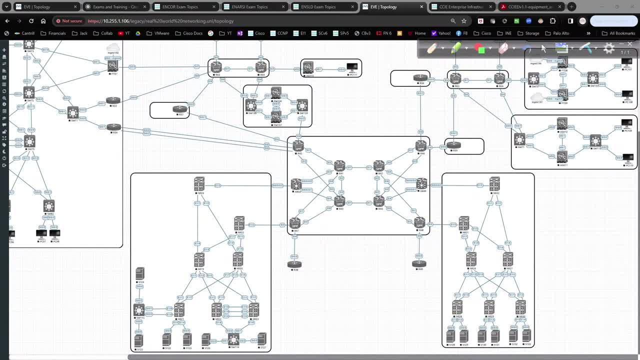 Don't be afraid to just comment on the videos. So I'm putting together. there's a. there's one comment that was left earlier- I think it was earlier today- where somebody put out there: Uh uh, where is it? They literally gave me a list of things that they would like to see in their real life networking course. 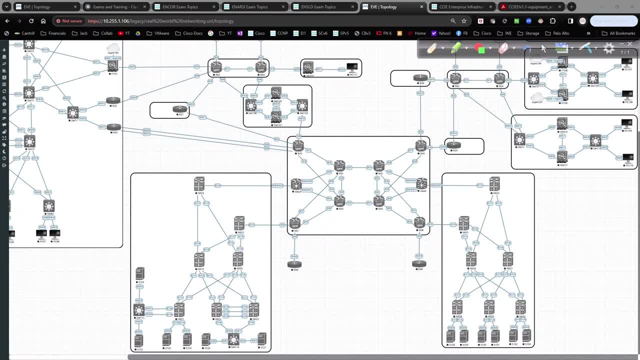 Real world, Real world, Real world, Real real life, whatever you want to call it- and great ideas, but it's just one of those things where that is specifically going to take some time to to go through. So, um, but yeah, I totally can put something together for that, or fans. 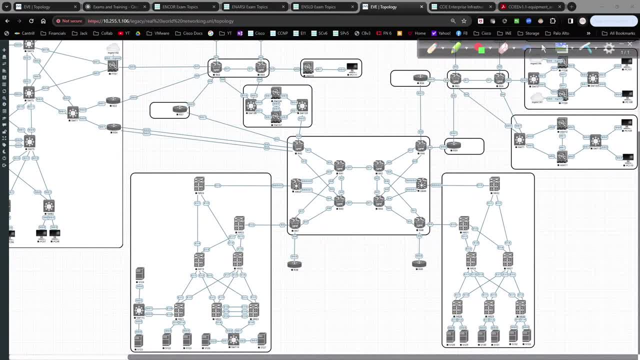 Just one of those things where I'm, uh, one step at a time, but, yeah, uh, I have actually have to learn a little bit more about V4 to V6, um, and then the implementation piece to it, So that's a great scenario. 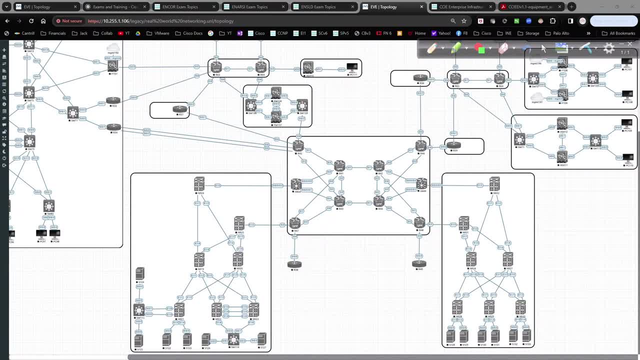 So I know we're at the top of the hour here so I'm I don't want to. I know some of you are probably going to drop off at the eight o'clock hour or wherever you're at, because we're one hour in. but, um, one of the things that, um, I'm planning on doing or I'm thinking might be beneficial anyway for real world course is, excuse me, is, uh, doing it more of a live stream type of uh, uh, live stream type of thing? 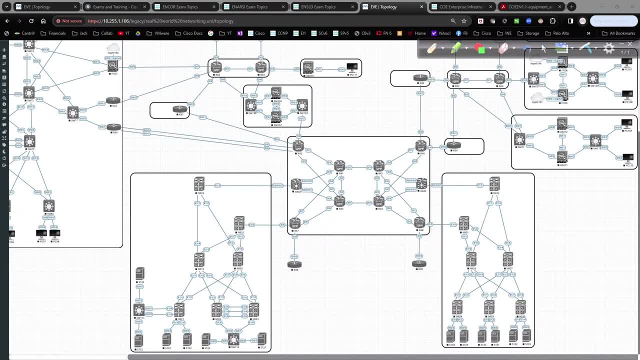 Of way of doing it, where you guys will come in live and then in the chat, or we launch a um, a Microsoft teams call. uh, a handful of you jump on the team's call and we can talk through whatever Um. so, yeah, I, that's, that's the goal. 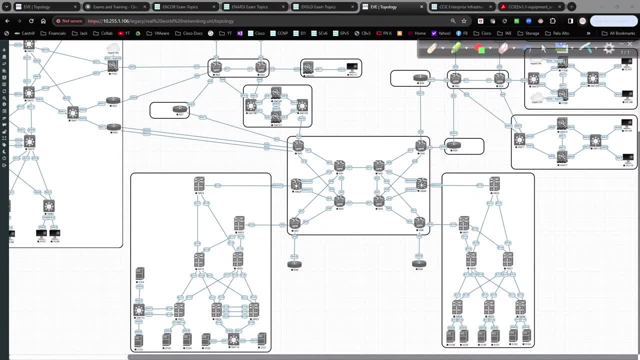 I'm, I'm, uh, when the real world networking becomes more of a reality, to to roll out and do. It's going to take me some time to figure out all the moving parts to it, Cause there's a lot of really good ideas out there, but, um, that would be, um, something I would, I think a lot of people would benefit from- is being able to go through that. 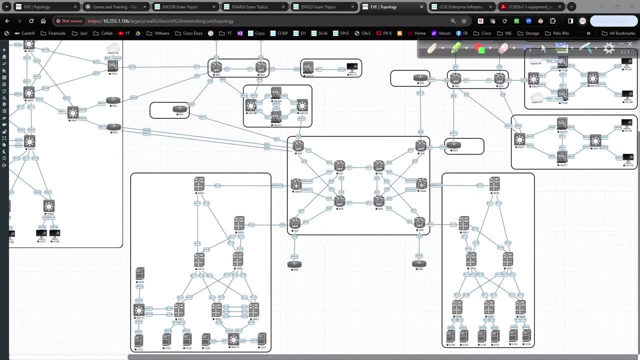 So at least that's the idea that I have in the back of my head. So I think it would be kind of cool to see that come to fruition and things like that. So, but, uh, I'm going to actually convert this over to um a. 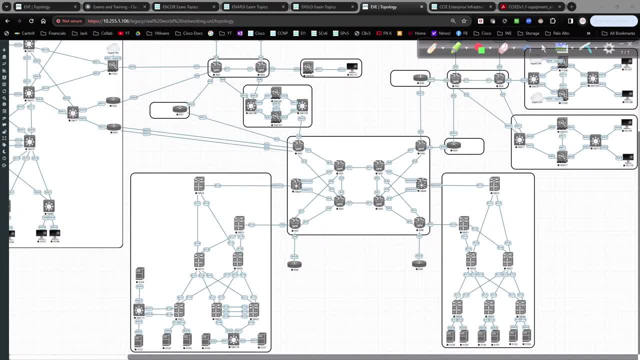 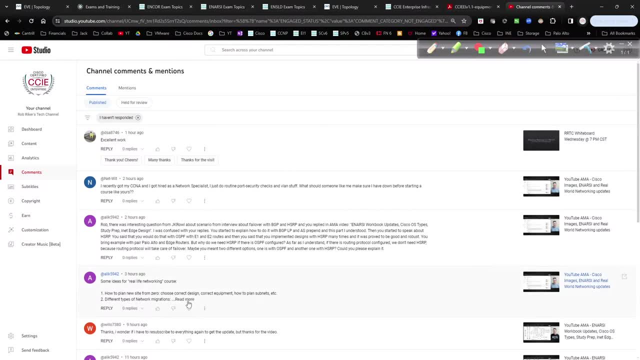 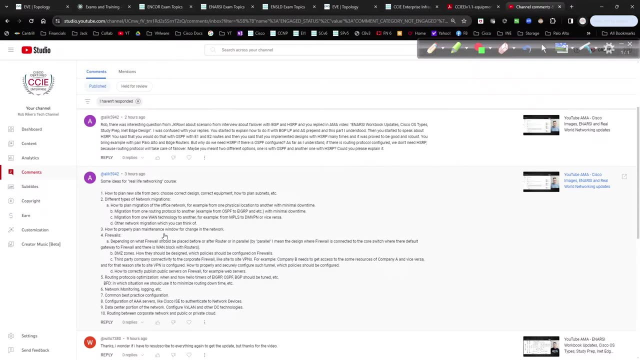 Live, ask me anything, because there's a couple of comments that came in recently and I want to just handle them. So this is the one I was just telling you about her fan. This is, uh, the guy laid out a whole dissertation, if you will, of what he likes to what he wants to see. 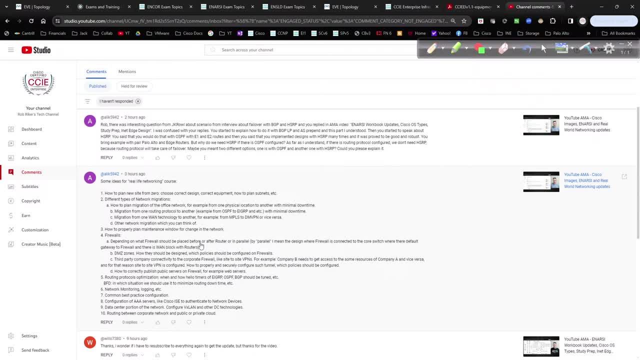 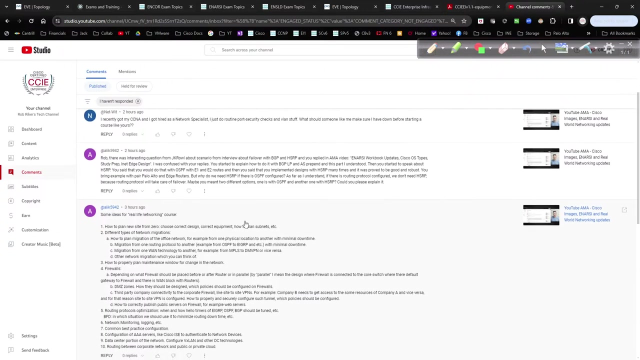 So it's actually quite a bit that uh, uh, a lot that goes in with that. So So, for those of you that are still watching, I'm going to convert this over to a live YouTube. ask me anything video. I'm actually waiting for the- um, the video to change over to that, but, um, so we're going to handle a couple of 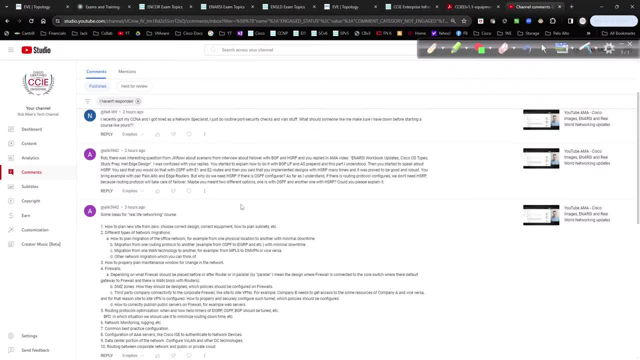 Yeah Right, I should have asked him to send me a steak, Um, so, yeah, So I'm going to. I'm going to handle this question real quick, um, or you know, semi, semi quick. Um, so there was an interesting question from JK Rob, but a scenario from interview, uh, about failover with BGP and HSRP. 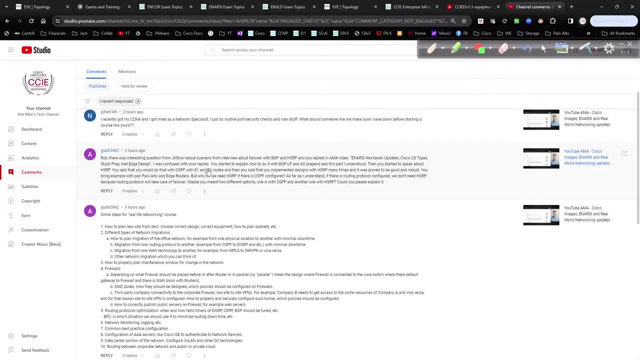 And you replied: uh, I was confused with your replies. You started to explain how to do it with BGP. Uh, no worries. uh, Tyler, Thank you too. Um, you started to explain why, with BGP, L local purpose and as prepend. 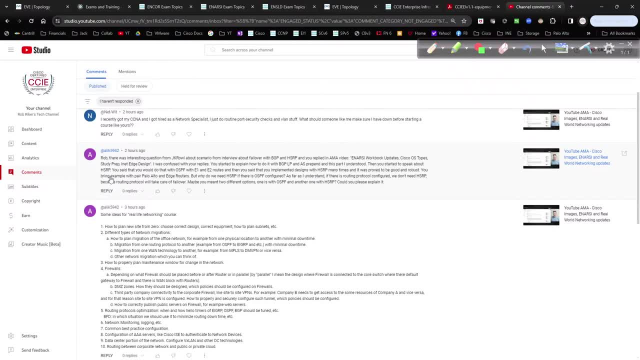 And this part I understood. then you started to speak about HSRP. you said that you would do that with OSPF, with E1 and E2 routes, And then you said you implemented this design with HSRP many times and it proved to be good and robust. 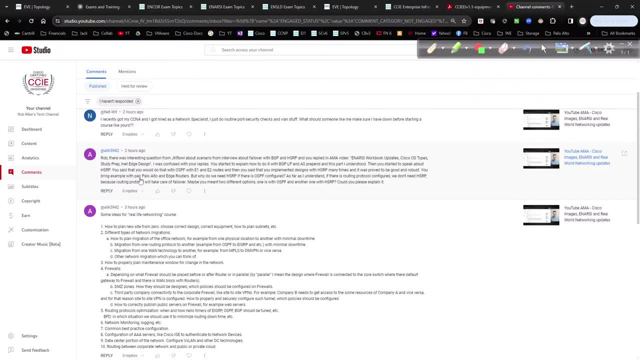 Um, you bring example with pair out uh, Palo Alto and edge routers. but why do we need HSRP if there's OSPF configured? as far as I understand, if there is writing protocol configured, we don't need HSRP. 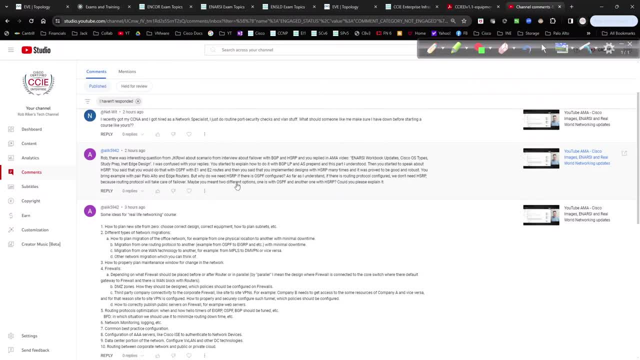 Because writing protocol will take care of failover. Maybe you want met two different options. One is OSPF, the other one HSRP. Can you please explain it? So this is why I like the community that I've built, because if people have questions, they're not afraid to throw it out there. 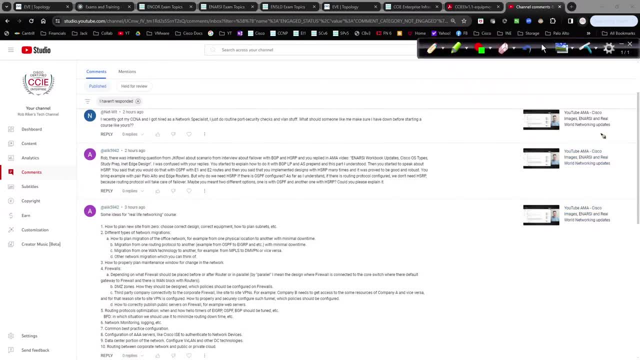 So let's, since we're here and we're alive, why not just, why not just handle it Right? So, um, so yeah, the the. let me break this down here, Let me pull up the topology that he. 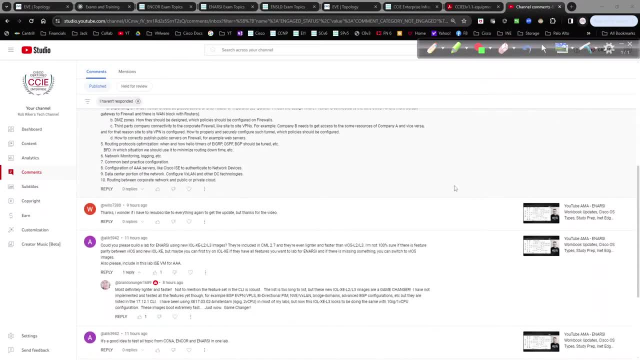 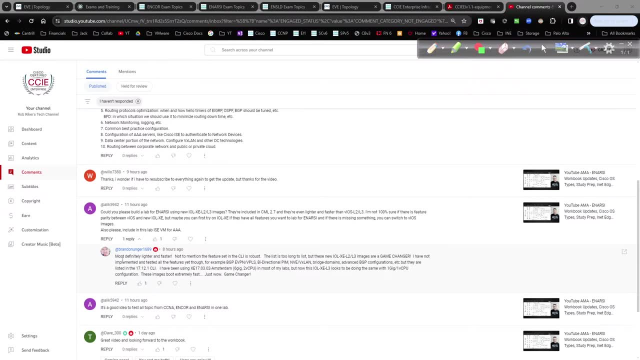 Yeah, Yeah, Used, it was. uh oh, there's a comment here about this. Okay, Uh, uh, so most definitely later and faster. not to mention the feature set, and the CLI is robust. This is too long of a list, but game changer. 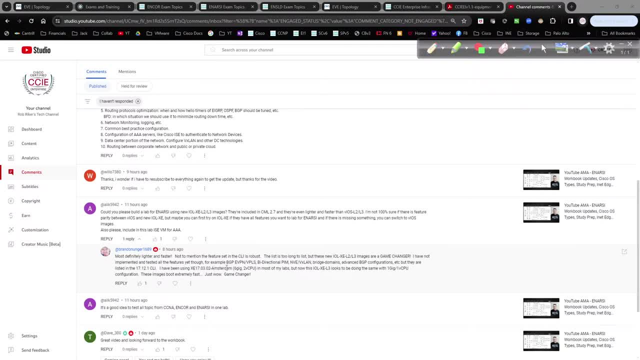 I have not implemented tests at all yet, but um, for example, VGB, EVV, VBLS, uh, directional PEM and VXLAN bridge domain, advanced PG, et cetera. They are listed in 1712 config. 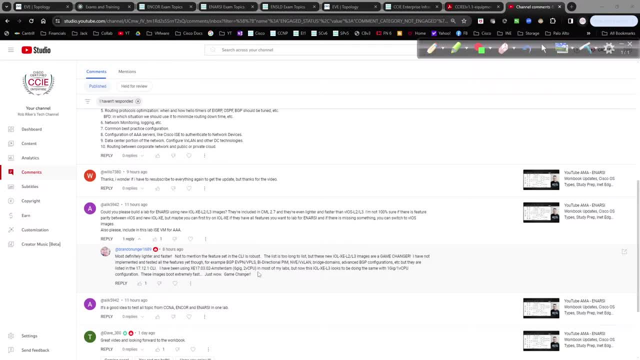 Um, look at the same one gig when we BCB configuration. Okay Well, Hey, you know what, Brandon, uh, Brandon Unger, you've might've converted me over to be a uh IOL fan, So I'll have to see about getting that. 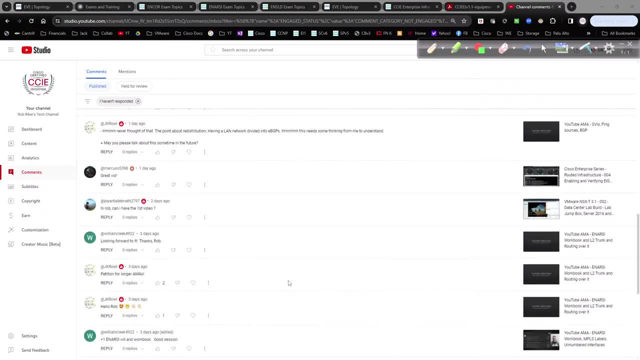 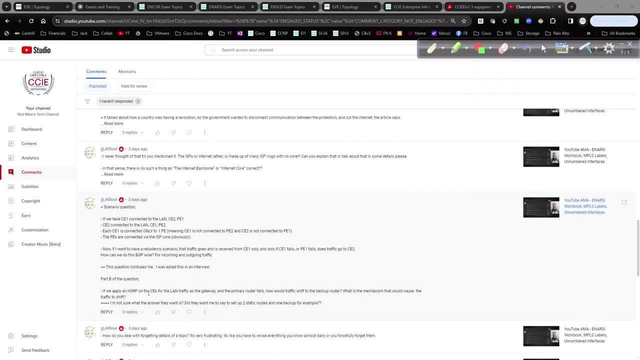 Um, so it's JK Rouse. Uh, where was it Right here? So Okay, So we have CE1 connected to LAN, And so CE1 is connected to PE1 and CEP. Okay, That's what it was. 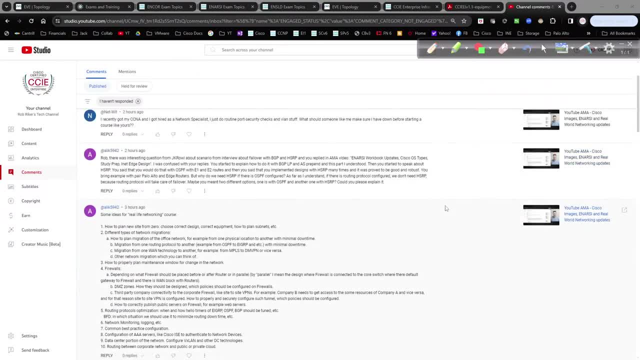 All right. So let's go back up here to your question and uh handle this. So we have PE1.. We have PE2.. We have uh CE1.. And we have CE2, CE2.. These guys are both peered to their providers and there's a link between the guys. uh, whether this is connected between a switch or if this is connected to each other directly doesn't matter. 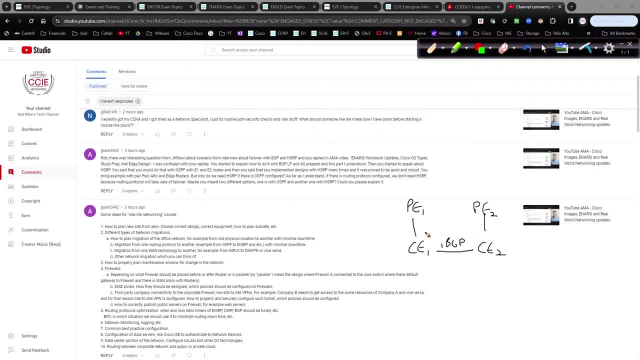 And there's an IBGP peering between the two. So we're get- we're going to assume we're only getting- a default route, So we get a default route this way. We get a default route this way, And what we do from this one here is we set the route map here, uh, for local preference of 200. 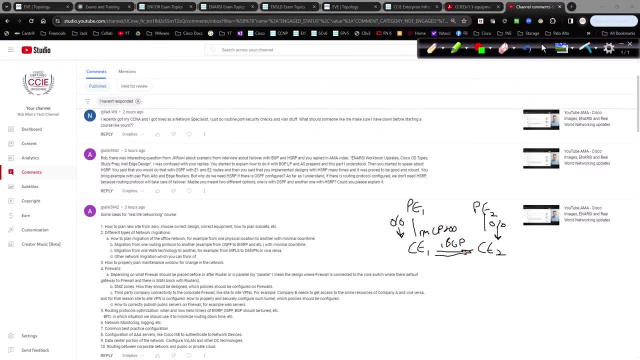 So when we get this in, he's going to advertise this guy to CE2.. He's going to get the default route two different ways, but he's going to choose the local preference 200 path this way. What we do here on this link is we do a route map here for ASPath. 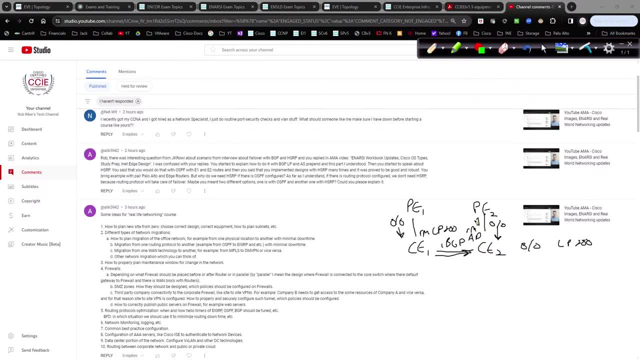 I'm going to put his AP for ASPath prepending And we set that out so that traffic will come in this way and also leave this way. Okay, Now specifically to the other piece that you were asking about is: Okay, Uh, Mario, I'll take your word for it. 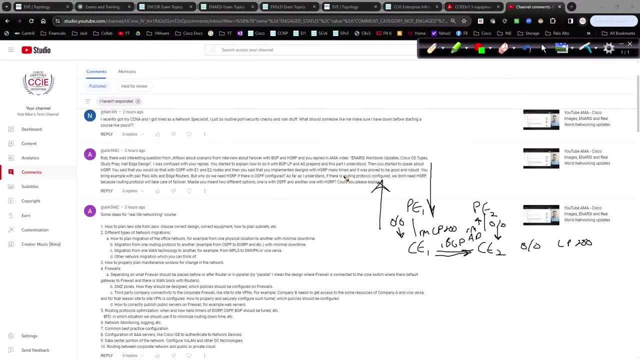 Are you? is FRR meaning free range routing? Is that what you mean? I think that's what you mean by FRR. uh, uh, free range routing. I'm sure you'll confirm that for me, though. So you take a scenario like this, where you go down to your distribution switch. 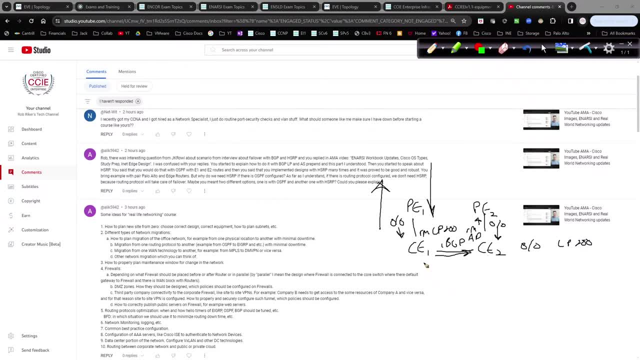 Now, the reality of it is, you're probably going to do something more like this, And this is my- probably my- mistake is you're going to have, uh, this connected like this: You're going to have DS one, You're going to have DS two. 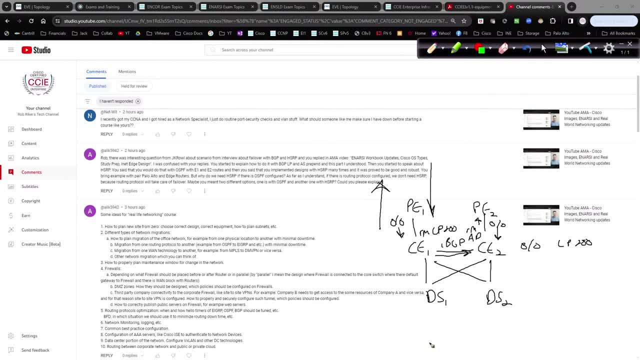 And then down here you're going to have something else, So you'll You'll have, say, access one and access two, and they'll be connected upstream respectively, like this. This would be more like uh, more than likely the design uh, cause you're going to want a redundancy everywhere. 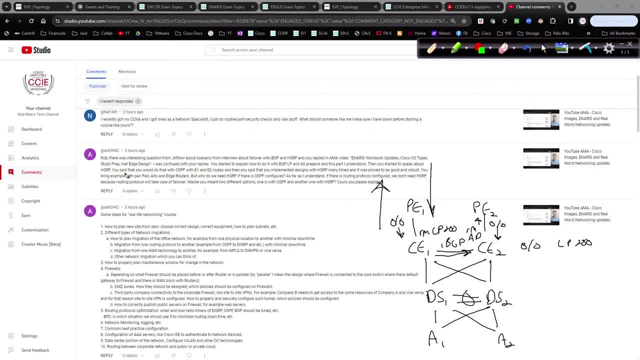 So you're. then you started to speak about HSRP. You said that you would. you, you would do OSPF, E1,, E2, um routes And then you said: okay, cool, Thanks, Mario. Um, you said you implemented designs with HSRP many times. 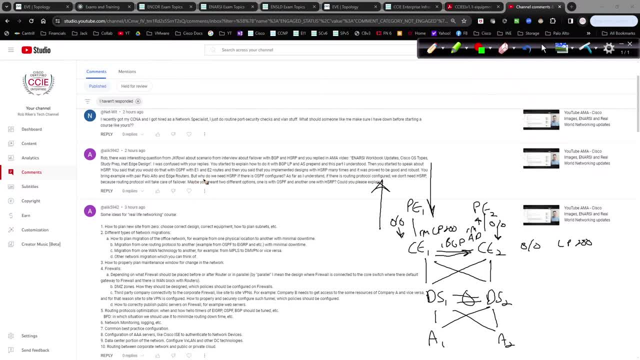 And it proved to be good and robust. uh, Palo Alto edge routers. Then why do we need OSPF? Okay, So why you would need that particular design? So what I would do is, when you're getting this via BGP, the default route via BGP, you're going to have a uh zero, a default route in the writing table of both. 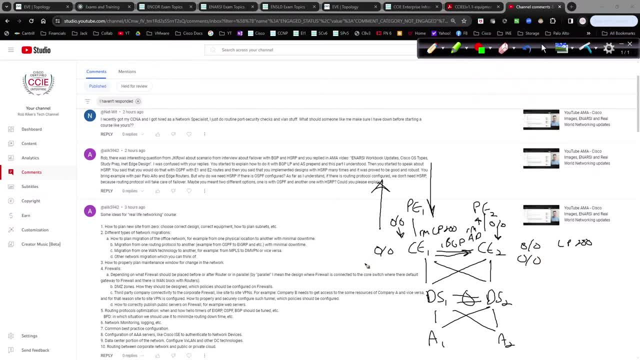 Right. So OSPF by default, when you do a default information originate, it's going to redirect, it's going to do a default information originate with, Okay, Okay, External type two on both. So if you want to prefer one CE over the other, then you're going to want to. based off of OSPF path selection, you have the, the finite state machine, I think is what they refer to it as. 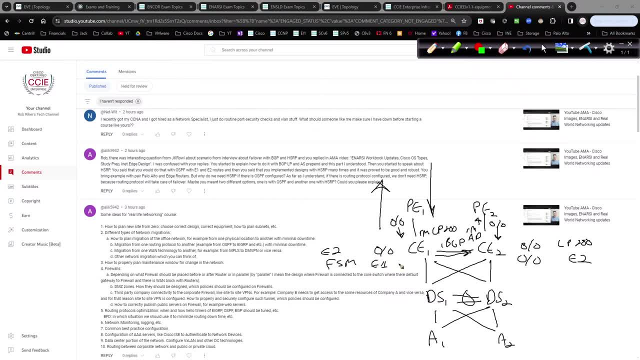 And E1 is preferred over E2.. So if you do a default information originate metric type one, it's going to propagate the district the default route down to DS1. As E1. And then this guy here I will do the same thing, but is E2. now they'll both get it right. 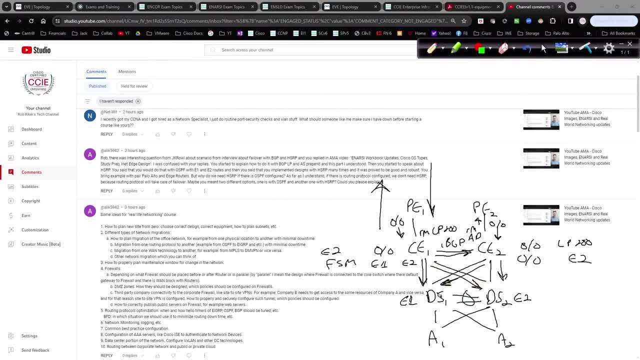 Cause it'll be propagated this way. It'll be propagated this way. So DS one, we'll get the route. DS one, DS two will also get the route, but this guy will be the preferred path outbound because his OCS metric type will be lower. 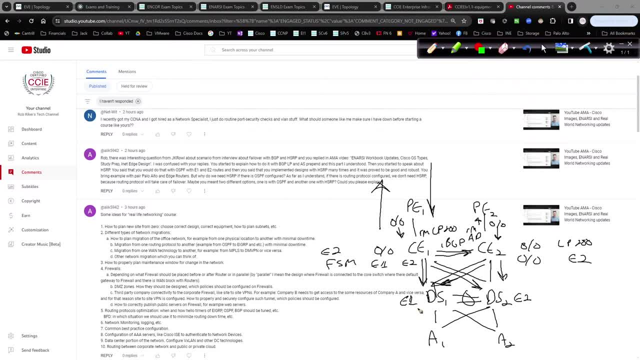 So anytime your metric is a metric type is lower, Does it matter The cost? The metric type is what's going to win. So now you've got a dedicated path from ds1 and ds2 going up from ds1 to east, ce1 to pe1. so 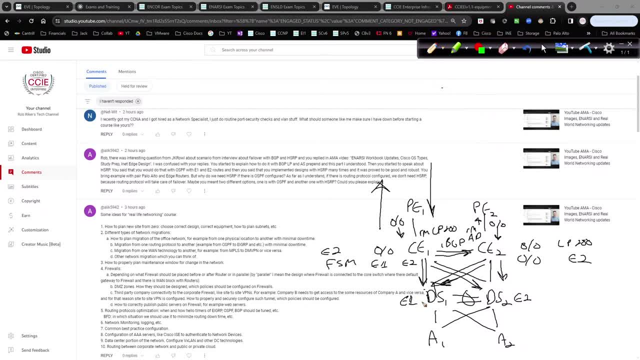 Let's go to. this is your, This is your egress path outbound. Hopefully, everybody's tracking so far. So now you have your. You have your first hop redundancy scenario come into play. So how do you handle this? So you have a couple different options. You have hsrp. 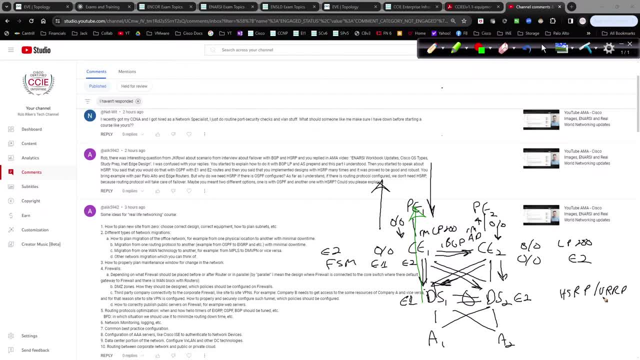 You have vrrp, So on and so forth. so I would probably go hsrp just because the fact you know it's, it's- unless you've got You know- a reason to go vrrp. They do the exact same thing, Just one cisco: proprietary. 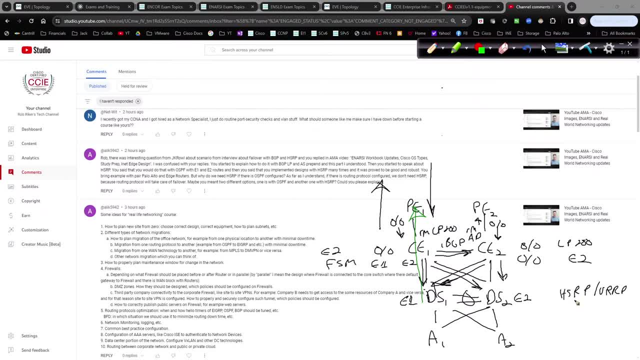 So, for the sake of argument, we'll say that you're going to go hsrp. So what you'll do is you'll configure the group on this one here to be. Let's say, for all your VLANs, We'll say: we grew up for VLAN 10.. We say: 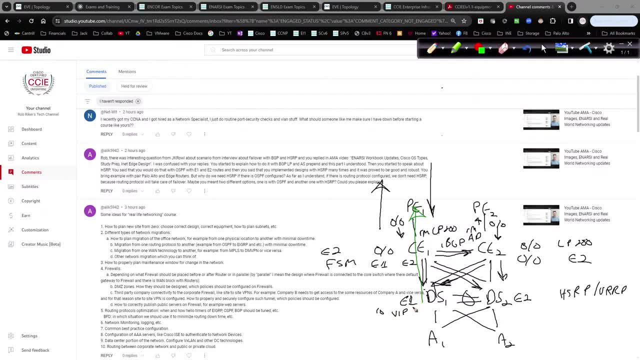 this will be the. you'll set your vip, and Then the, the Mac that goes along with that, and then you'll set your priority. Let's say you set your priority to be 150 and then this one over here is 100, so by default this guy will become your egress point and 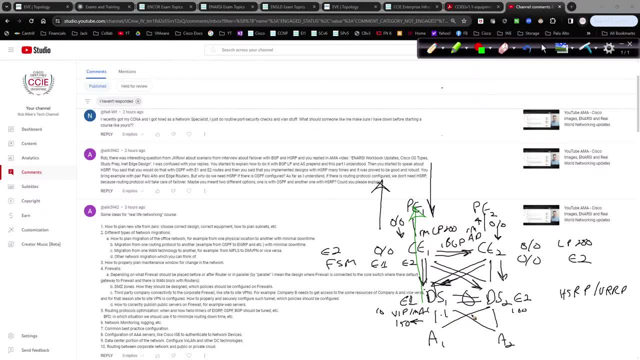 So your dot one will sit here, even though it's shared between the two, And your hsrp hellos will go back and forth and all that good stuff that goes along with that. so In the event that this, this pe, takes a dive, Let's say, for example, there's a, there's a fiber cut and that particular peering goes down bgp. 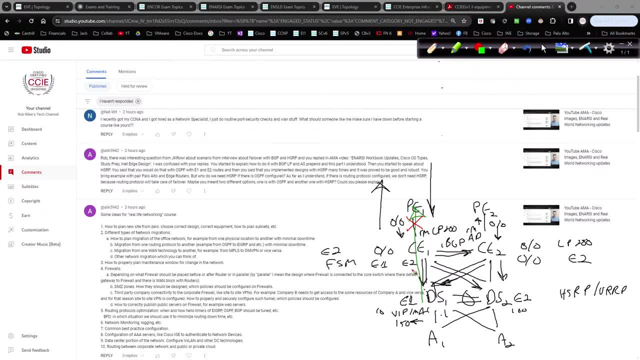 Route is lost And you're up up the creek without a paddle. Okay, cool, Guess what? the moment you no longer receive the default route dynamically, You no longer are going to receive it in the routing table. Therefore, OSPF is not going to see it in the routing table either and is going to yank it. 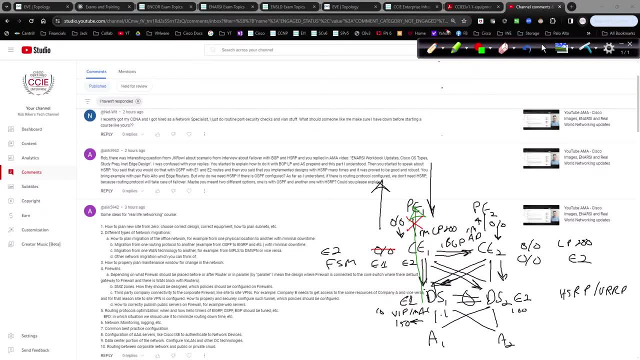 So you're no longer going to have that path. so now what will end up happening is your egress point will now be out here through ce2. That's where that'll come into play. But hsrp doesn't get touched. so by Advertising two different metric types, You can pin the traffic where you want it to go. 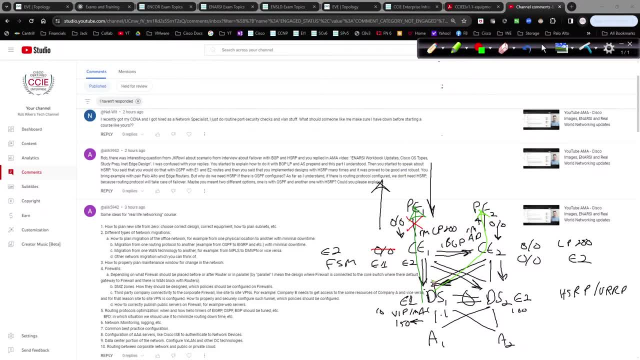 Now, one of the things that you could do Is by setting the metric, but the problem is- or, i'm sorry, not the metric, the cost. you could set the cost, but the problem is: is the cost is going to be? oh, when you do a default information originate, you can set the. 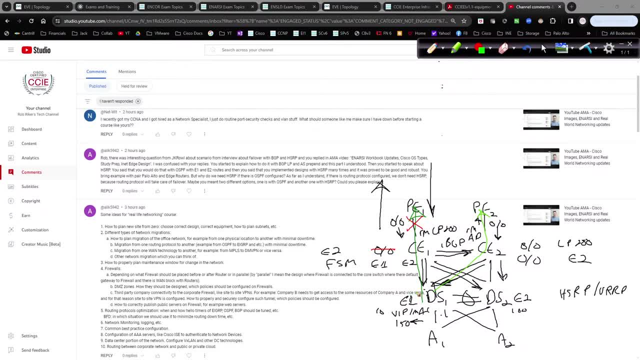 The cost value higher and do it that way too. That that's, that's a valid design as well. I prefer going the metric type because then it's a no, There's no guesswork, right? You know exactly where the traffic is going to go. 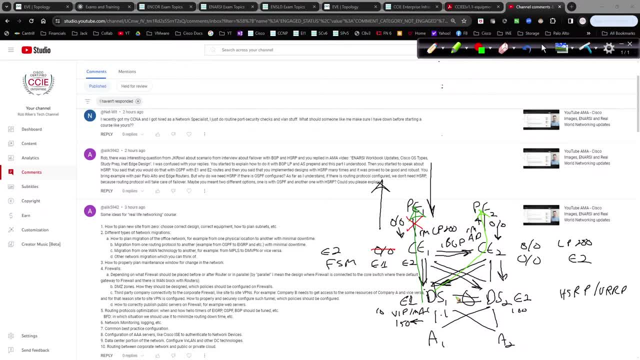 So that's where that would come into play. so In this particular design, this is what I would do. if a customer was talking about Edge redundancy and how the connectivity would come into play, This is what I would be suggesting. Are there other ways of doing it? There are. are they better? 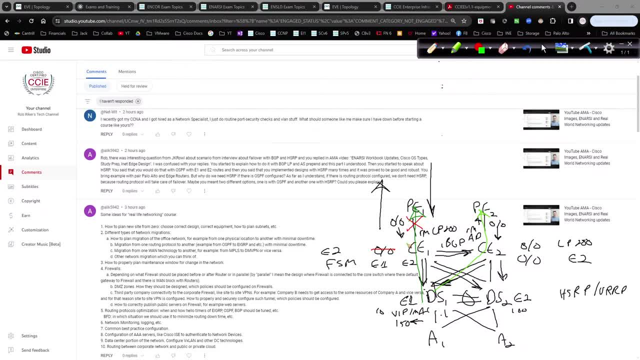 Yeah, It depends. you know you'd have to have a conversation with them about what they're trying to accomplish and things like that. So Hopefully that answers your question, But that's what I would end up accomplishing. So hsrp vrp. 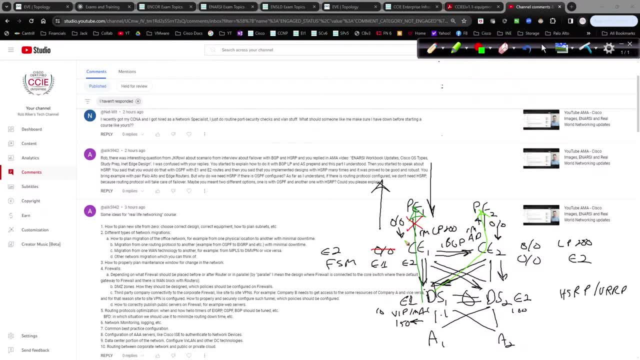 and then you set the, The priority level, and then you can do your preemption. if you wanted to do so, fail back over all that type of stuff, but That's what a typically a lot of customers are going to want to see Is no matter what part of the network you're in, you have high availability now. could you run. 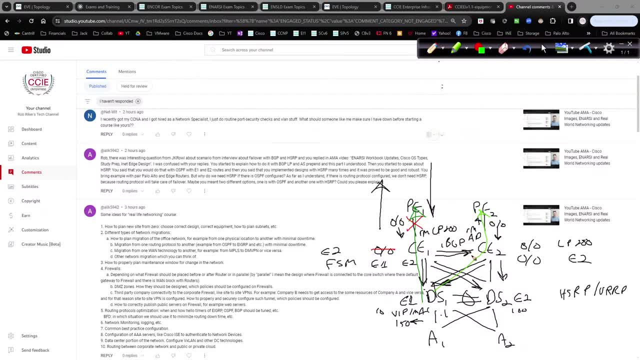 ospf down here, we could flip back over to black. Could you run ospf down here? You could. yes, the drawback to it is you never want to enable a dynamic writing protocol on your land facing interfaces to toward your access switches for the unlikely event that somebody takes and plugs in their own little box. 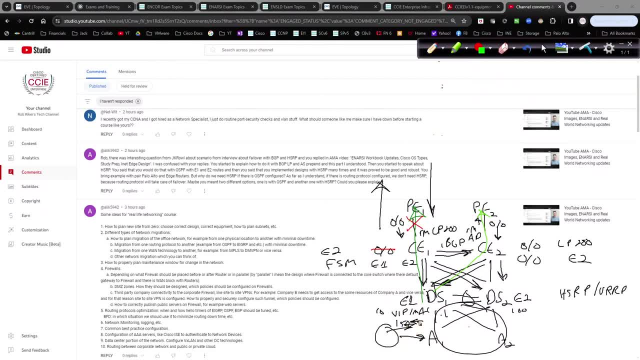 And then starts doing their routing, and then they advertise a default route and then your writing gets hosed. so You never want to do that. what you want to do is for all of the Svis That are sitting on your distribution layer switches. What you would do is for those particular subnets. you would just do: 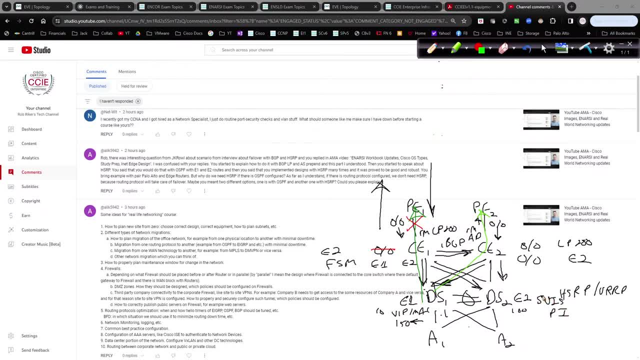 an interface at the ospf or eigrp process level and you would not send Hellos out or receive hellos in, but you would still advertise those subnets into igp's database And then propagate them wherever they got to go. That's what I would end up doing. So then ce1 and ce2 would receive those routes and then 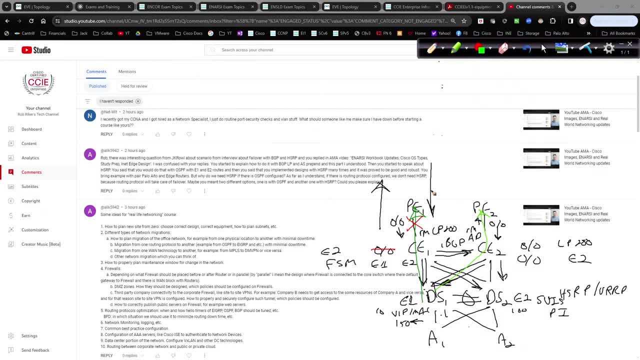 You'd be able to do your gnats or whatever's going on here. So that's essentially what You would do. So let's see here: you bring example with uh, palo and edge routers. But why do we need it? Okay, so just making sure that I didn't miss anything, any part of this question. 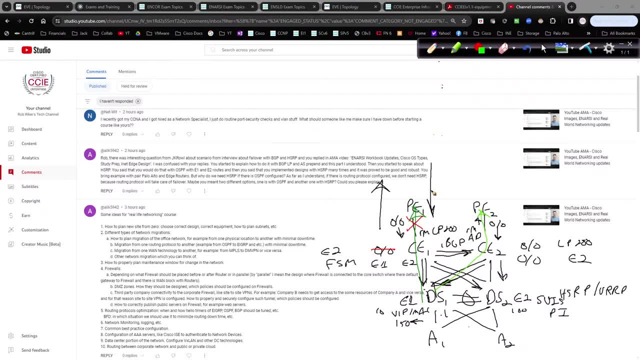 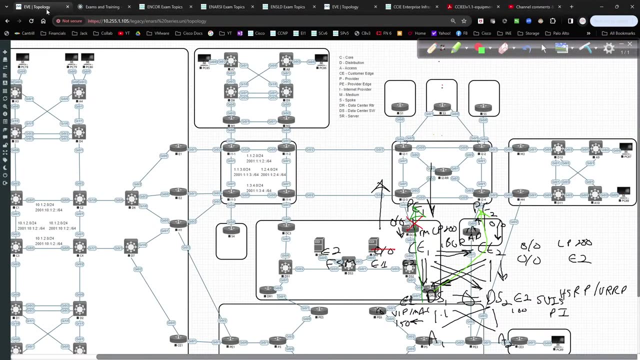 hopefully that answers your question and uh, stuff like that. so, um, It's a fairly straightforward design and it's actually now that you bring that up, i'm going to go ahead, and I think what i'm probably going to do Is I think I need to build out a 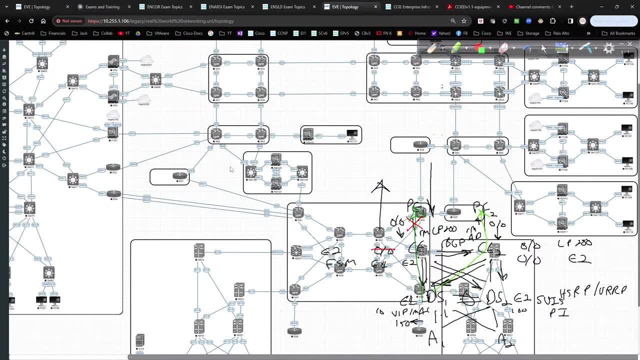 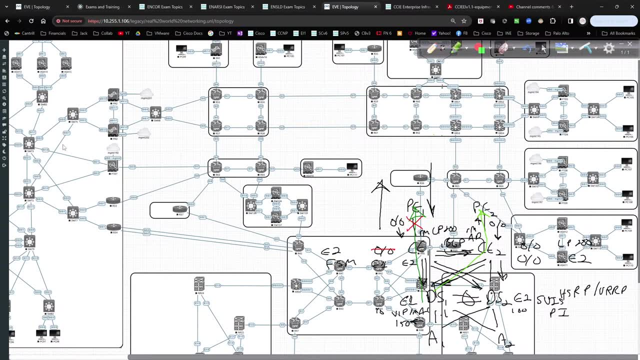 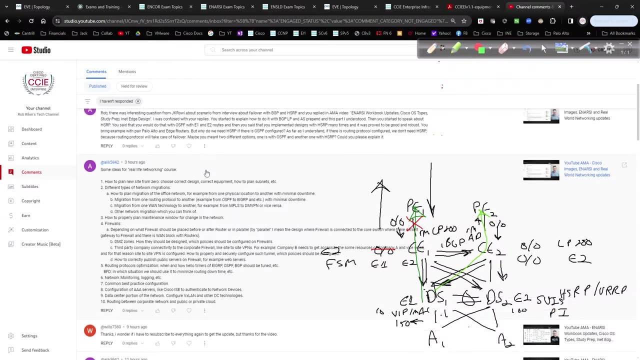 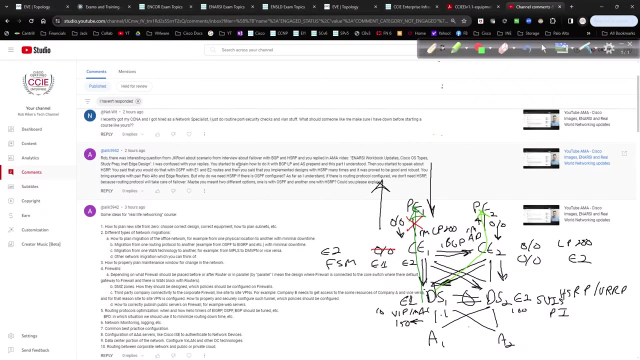 yeah. so for the Yeah, this is what i'm going to do. i'm going to make some adjustments to To this lab to include this specific example, Because it's not the first time that's been brought up. So I will go through and build out this exact same example and we're going to lab test it in the real world networking. 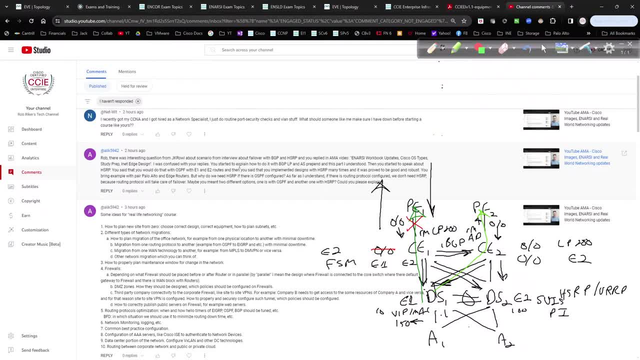 So that we make sure we cover it, because it seems to be a point of contention and I'll go from there because I think that would be beneficial to all of you to see something like that, And I will take what I did for that one customer that I talked about. 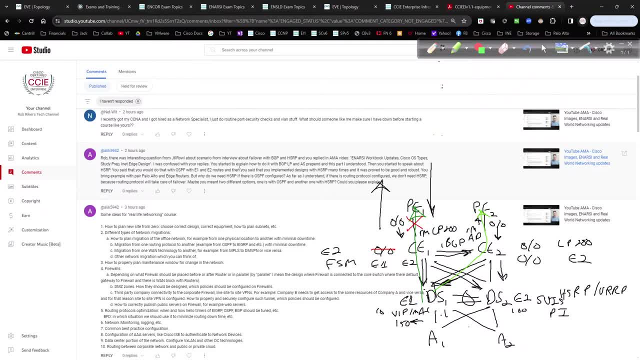 um, Today, no, the other, the other day, Uh, I think it was yesterday. I covered that I will have a couple of additional internet edge redundancy designs that we'll go through, and then we'll Go through and configure them and get them all stood up, including the palo firewalls. 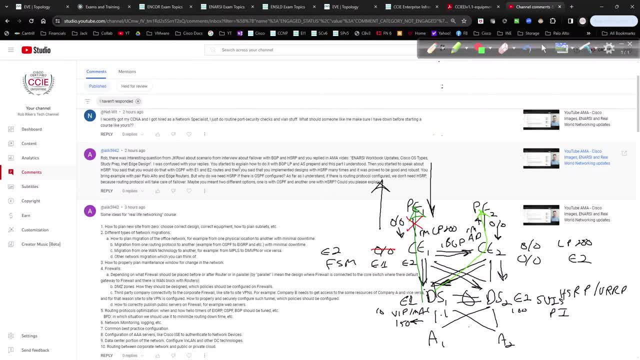 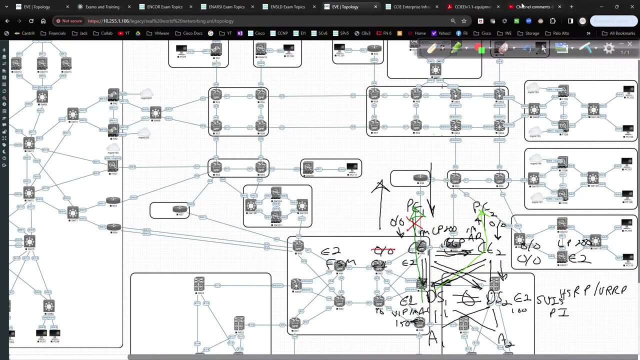 And the internet edge connectivity and go through what it is that was done in those particular examples, because I think that would be good for you guys to see. um, it's gonna take a little bit of uh rejiggering of my Topology in my lab, but it's it's doable. Let me go ahead and clear the screen off. 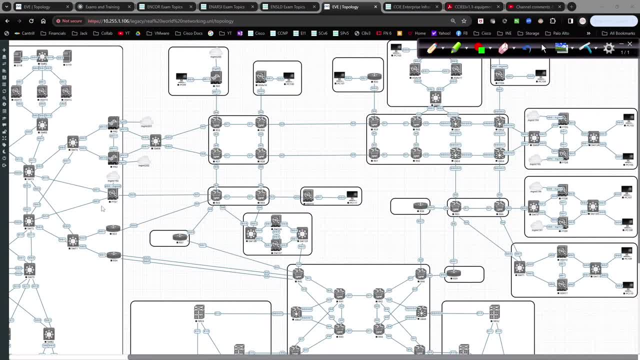 Um, it's doable. I was trying to make things a little bit more easy to work with, but, Um, I can totally make that happen. That wouldn't be hard at all to do. so, um, But yeah, other than that, that's pretty much what. 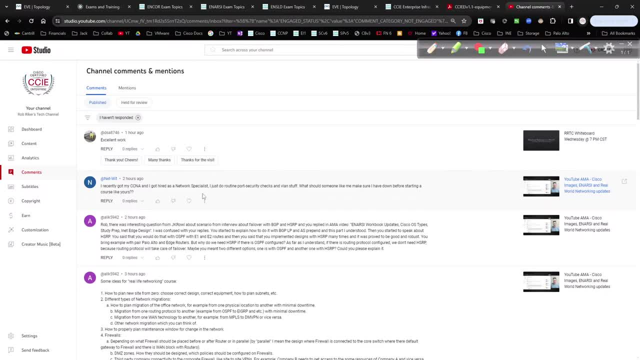 I wanted to cover. Uh recently got my cc and I got hired as a network specialist. I just Do routine port security checks and be that stuff. Why should someone like me make sure I have Sure I have down before starting a course like yours? That is a good question, Um. 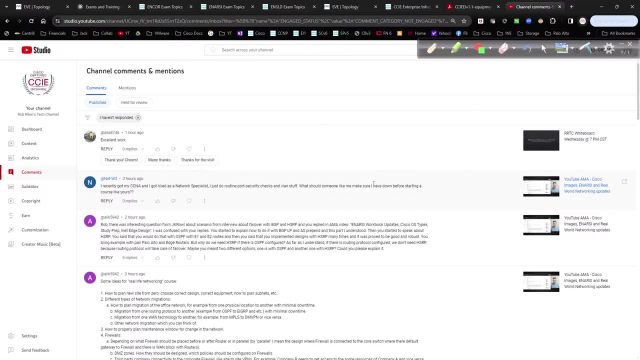 I will come back to this tomorrow. Well, The fundamentals, for sure. um, You got your ccna And you've got your your network specialist today, so You're just getting started. So This would be a good time for you to start digging in the documentation. 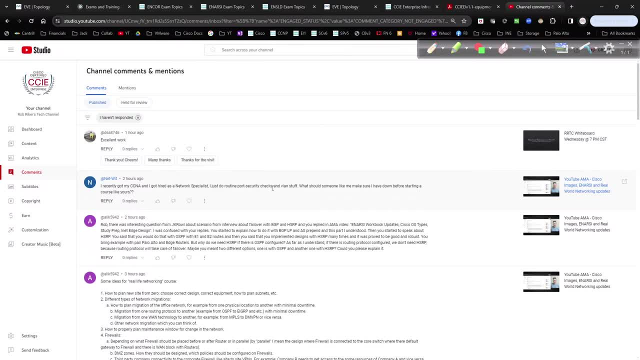 But i'll answer this in my own uh ama, tomorrow on during tech support thursday. so um, with that being said, I know i'm actually surprised There's still as many of you as there are, But uh, i'm gonna go ahead and cut you guys loose for the evening. It is already quarter after eight. 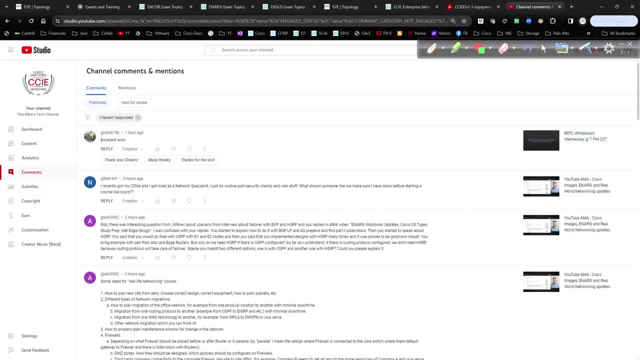 How are you going out over 15 minutes? So I want to thank you guys for stopping by and hanging out with me And all that good stuff that goes along with that. um, we will. I'll put out another video tomorrow for tech support thursday and um. 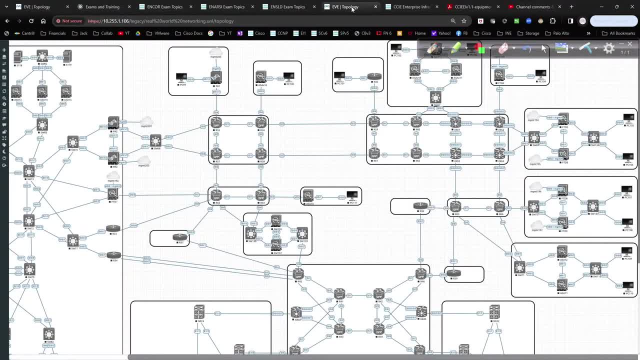 Go from there. Maybe i'll have an update for This topology with doing that. What time do you get online tomorrow? um, In general, i'm usually online probably about nine o'clock in the morning for work. but um, no worries, texmex happy to help. 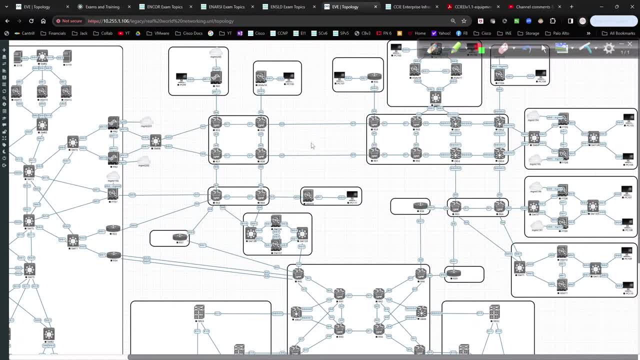 um, but if you're like, You have to clarify what you mean, or fan. I'm not exactly sure how to answer that, But i'm i'm typically online all day, So if, like you, had a Comment or something, i'm probably going to see it throughout the day. I check youtube probably five or six times a day. 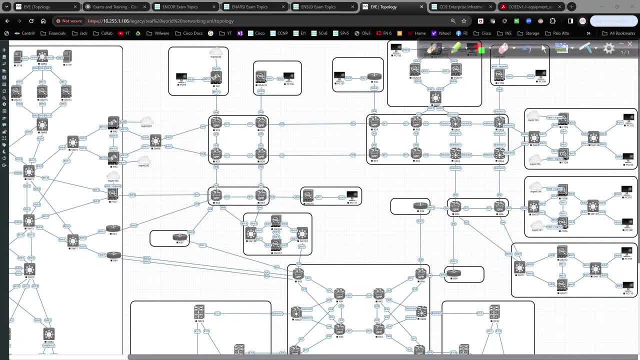 But go ahead and move that back over Your greatest pleasure. you're funny, mario, you're real funny. Oh, youtube live. um, tomorrow, Tomorrow i'm not doing one, Um, i'm. you know, I have a The friday coaching session. Uh, friday at 7 pm Central. 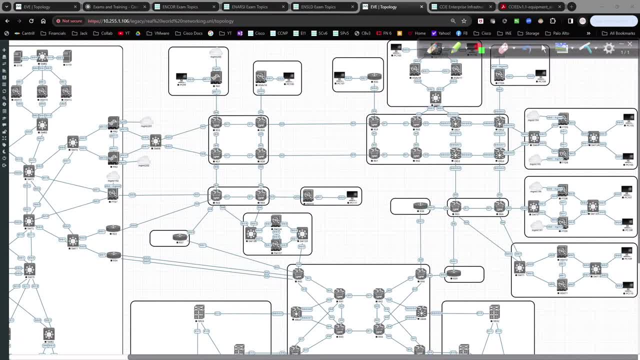 So if you want to join that, I think you're a member. if i'm not mistaken Members i'm mostly sure you remember. Yeah, I think you remember. yeah, you remember. so tomorrow at uh, i'm sorry, Yeah, you're. you're good man, uh. 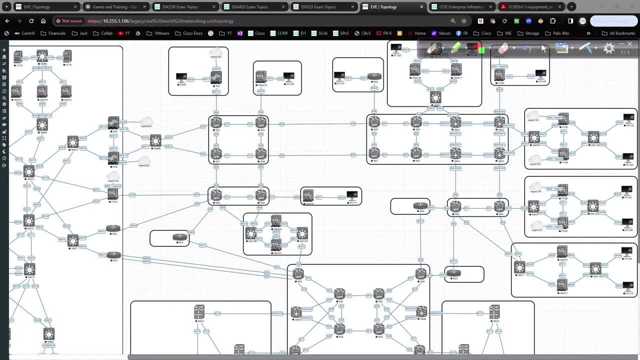 friday night seven o'clock I go live for a coaching session, So if you want to Join in then you know be my guest. you can join the call and hang out for a little bit. Okay, cool, Yeah, so if you've got time friday night seven o'clock to hang out for about an hour, 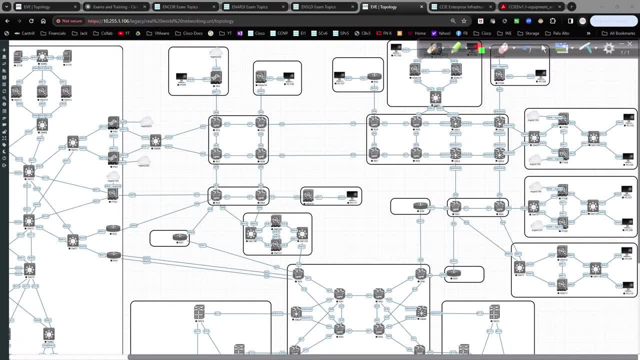 We'll, i'll be able to chat, So good stuff, dude. um. So actually another one came through Go ahead and uh, Well, i'm not gonna put this guy on blast on alive. Um, so anyway, i'm gonna let you guys go for the evening. It's been an awesome chat with you guys this evening.